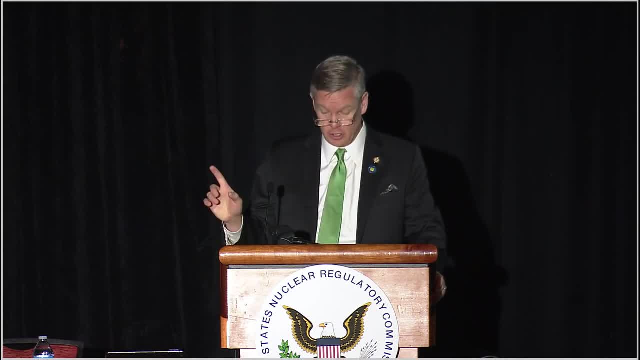 on licensing small modular reactors. I should note that just on Monday we added the United Kingdom to that arrangement as well Under our memorandum of cooperation. now, so far the NRC and CNSC have successfully collaborated on advanced reactor topics and have issued 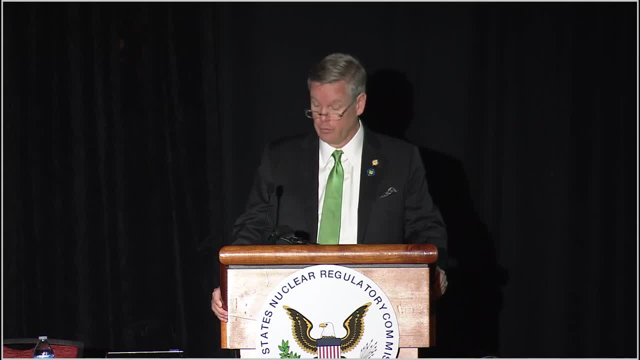 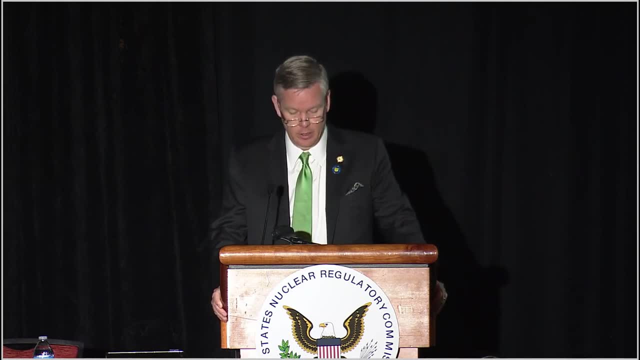 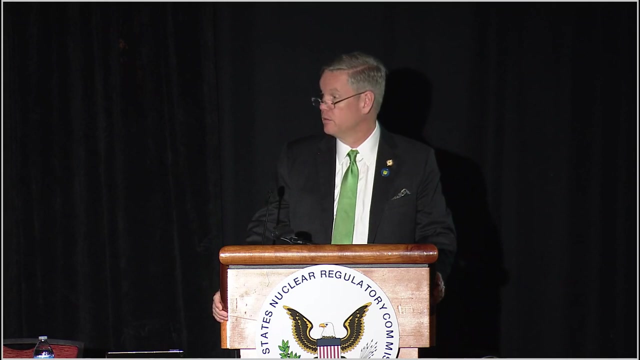 unified positions through first-of-a-kind joint reports. Both regulators see an opportunity to further this collaboration effort by jointly addressing tangible regulatory issues in licensing reviews. We found this interaction invaluable and I'm pleased to note that just yesterday, Ramzi Jamal of the CNSC and I assigned- well, I just already said that that we added. 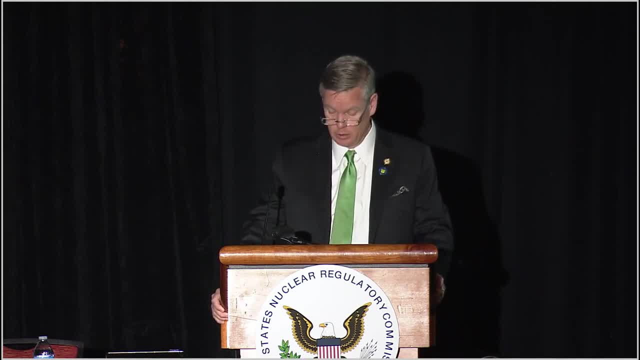 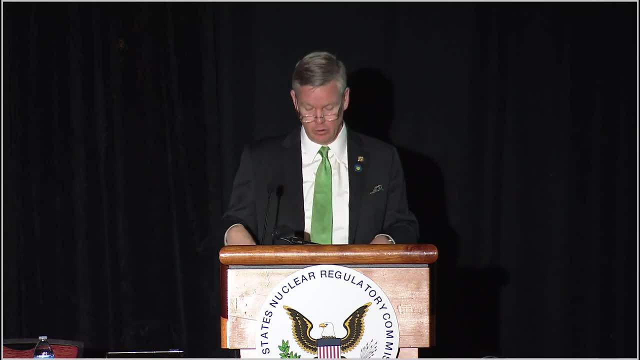 Mark Foy to this on Monday or on Tuesday, excuse me- and bringing them into the fold as we add more technical topics for joint reviews, I think is going to be absolutely valuable. This is critical and I expect this to be incredibly positive as we move forward Based. 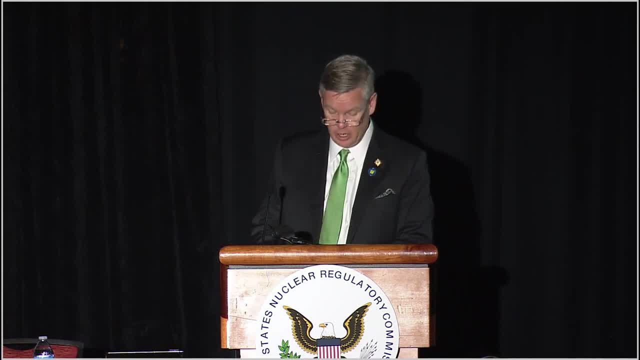 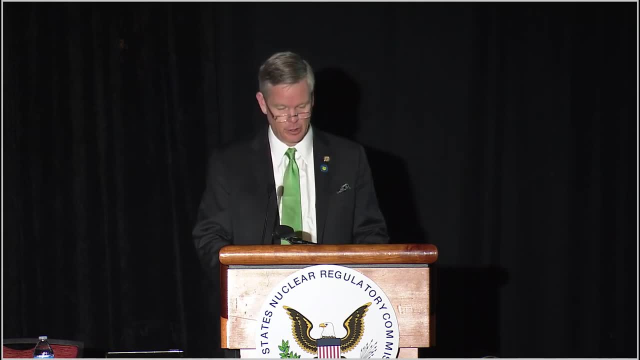 on the NRC's experience. I firmly support close collaboration with our international counterparts and we've gathered an esteemed group, as I said, of colleagues and friends here to share their perspectives. First, I'm joined by Mr Andrzej Głowacki Since March. 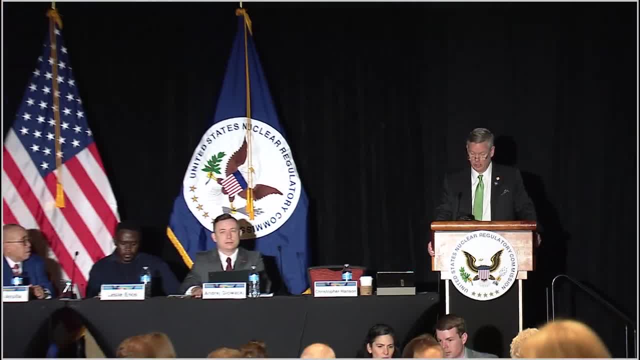 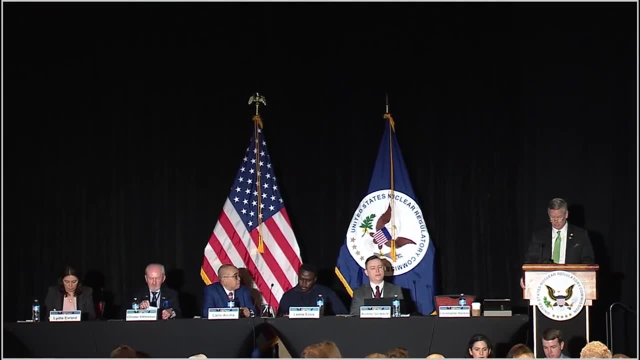 of 2023,. Mr Głowacki has served as the president of Poland's National Atomic Energy Agency, or PAA. He has worked for the PAA for more than 16 years, holding such positions as vice president of PAA and director of Nuclear Safety and Security Department. He has extensive international 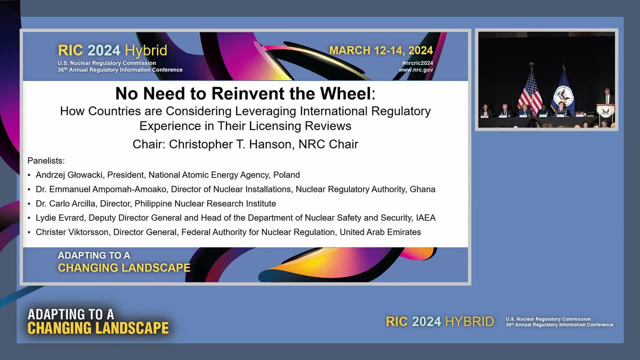 experience representing Poland at both the NEA and the IAEA. Next, in a last-minute addition, I am so pleased that Mr Lesley Enos has been able to join us from the Ghana Nuclear Regulatory Authority. He is a stress analyst at his organization. He has worked for the PAA for more than 16. years, holding such positions as vice president of PAA and director of Nuclear Safety and Security Department. He has been able to join us from the PAA for more than 16 years, holding such positions as vice president of PAA and director of Nuclear Safety and Security Department. He has worked 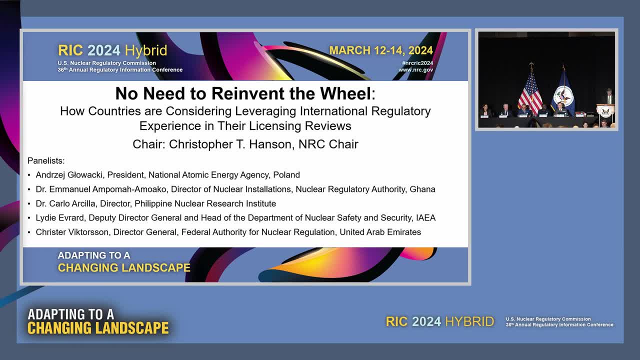 for the PAA for more than 16 years, holding such positions as vice president of PAA and director of Nuclear Safety and Security Department. He has worked for the PAA for more than 16 years, holding such positions as vice president of PAA and director of Nuclear Safety and Security Department. 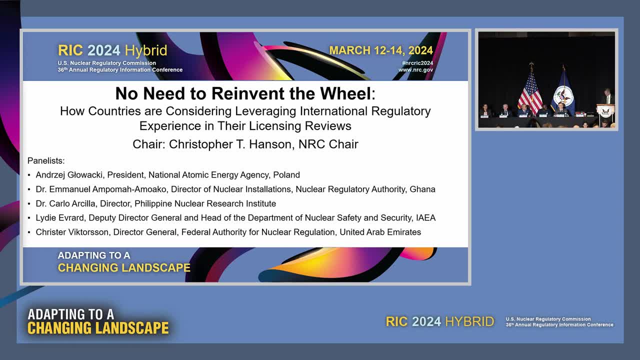 Next, Mr Enos is graciously stepping in today to share his agency's perspectives, and I look forward to hearing more about Ghana's plans for nuclear energy. Next, Dr Carlo Assia joins us from the Philippine Nuclear Research Institute, where 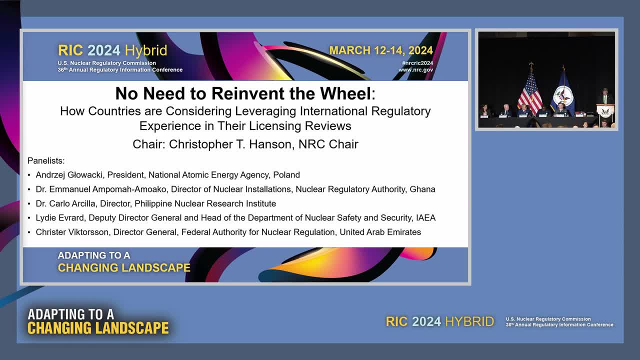 he has served as director since 2017.. In his capacity as the PNRI director, he is dedicated to promoting the peaceful application of atomic energy and supervising visitors to the similar atomic energy, and supervising the safe and responsible use of nuclear science and technology. 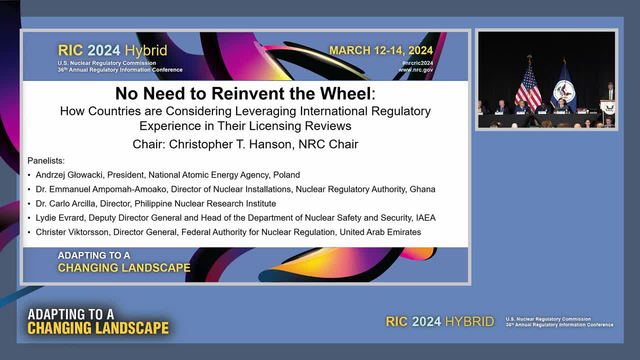 in the Philippines. Prior to his appointment, he served as the Director of the Philippine National Institute of Geological Sciences. Next, I'm joined by my good friend, Mr Krister Victorson, Director General of the Federal Authority for Nuclear Regulation. Director General Victorson has served as the head of FANR since 2015 and I'm pleased to 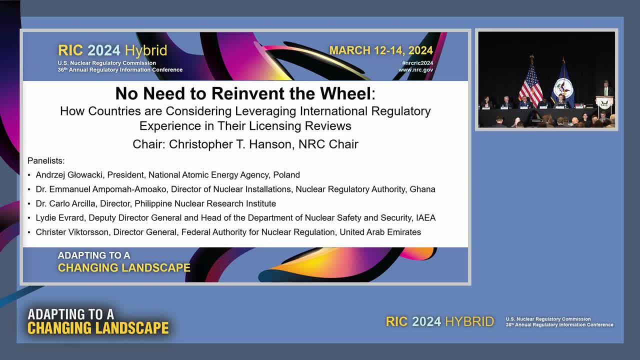 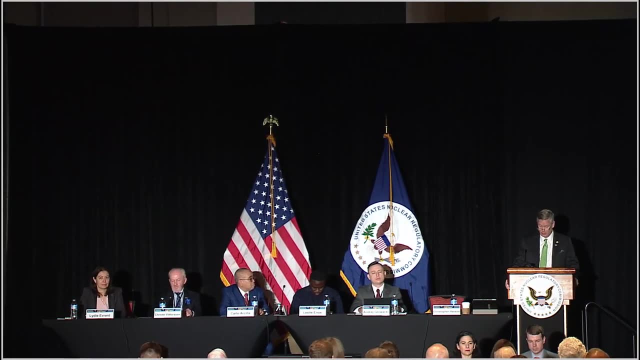 have served as a co-chair with him last year at the very successful International Conference on Effective Nuclear and Radiation Regulatory Systems in Abu Dhabi. Director General Victorson is a nuclear physicist with more than 35 years of national and international nuclear safety experience, including working at the NEA, the IAEA and serving as Deputy. 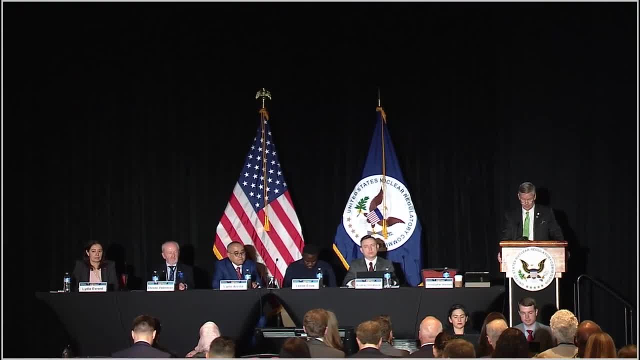 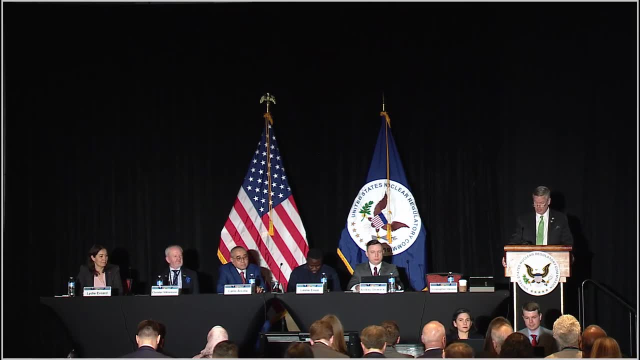 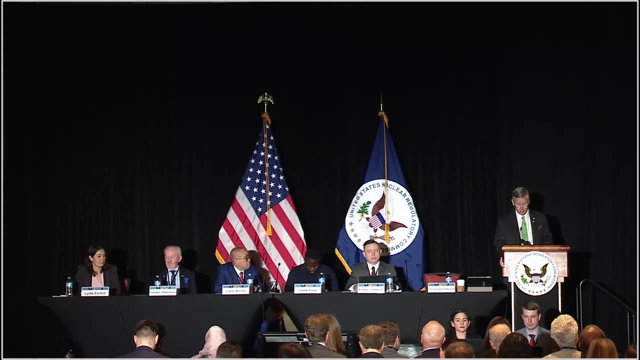 Director General at the Swedish Nuclear Safety Authority. Last, certainly not least, We'll hear from Ms Liddy Everard, Deputy Director General of the IAEA and the head of the Department of Nuclear Safety and Security. DDG Everard started her career at the French Ministry of Energy and has worked extensively. 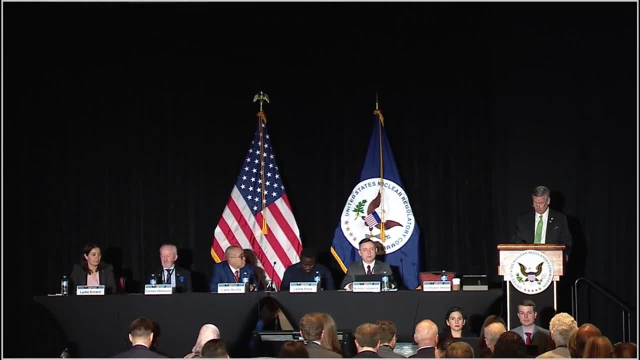 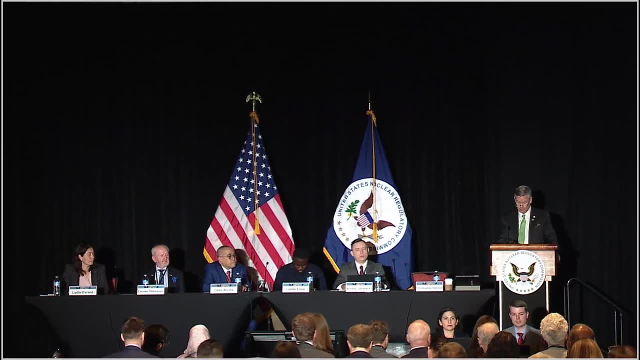 in the regulatory field over the last 25 years, including positions at the industry, research and environment directorate of France's Ministry of the Environment and France's Nuclear Safety Authority, where she most recently served as a commissioner. With such a strong panel day, 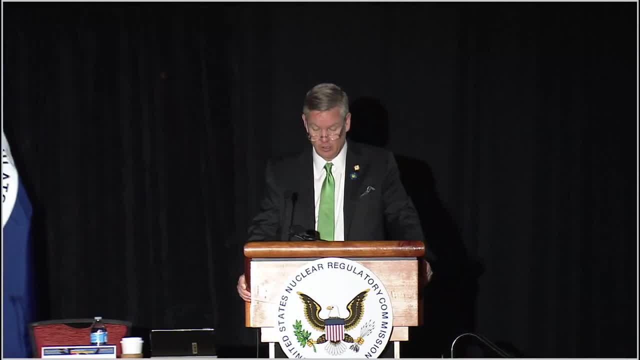 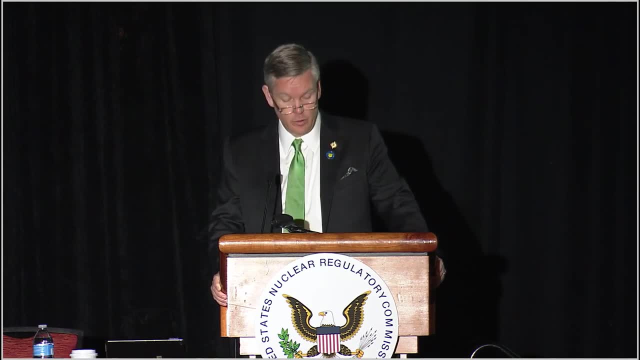 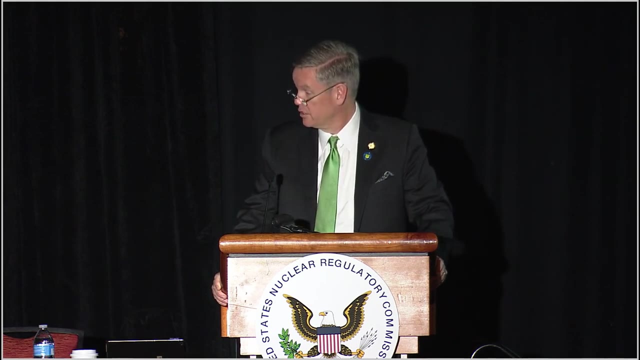 Thank you. Today, I'm certain, we'll have an exciting dialogue on the role that sharing international regulatory experience for licensing advanced reactors will play, as we do as we continue to see more advanced reactor designs develop. So, without further delay, I'll turn to our first panelist, President Klovatsky. 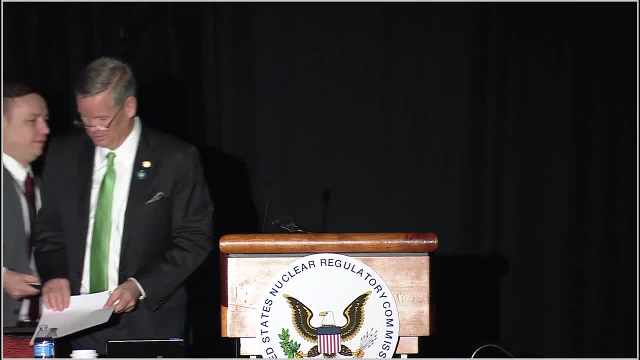 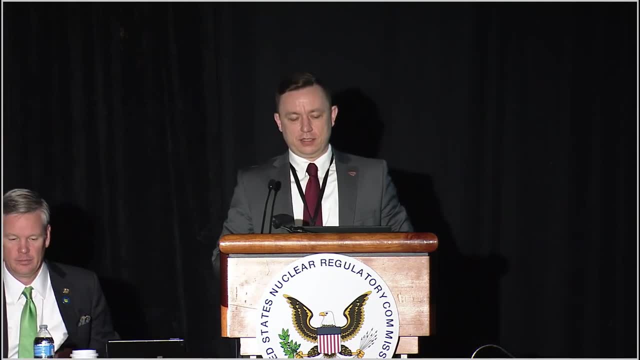 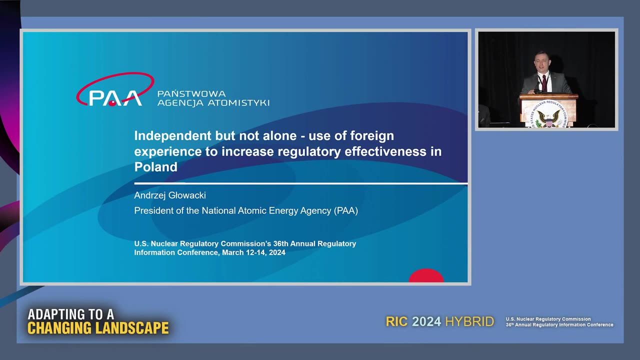 President Klovatsky. All right, Thank you, Chair, for your kind introduction. Good morning ladies and gentlemen. I'm a little bit like a movie star in this shiny, bright light. I'm going to walk you through our PE approach to preparation for the licensing of nuclear. 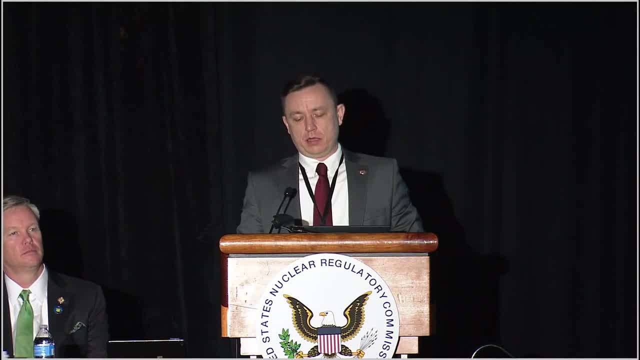 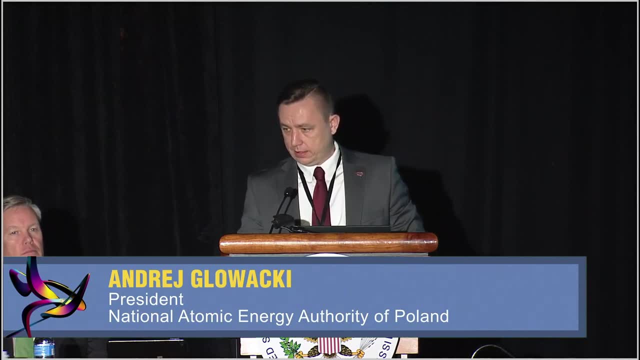 power plants, but also I'm going to talk about how to increase regulatory effectiveness by using other regulators' experience. So let's start, Okay. So the presentation is divided into three parts. I'm going to give you some overview of the current status of the deployment of nuclear 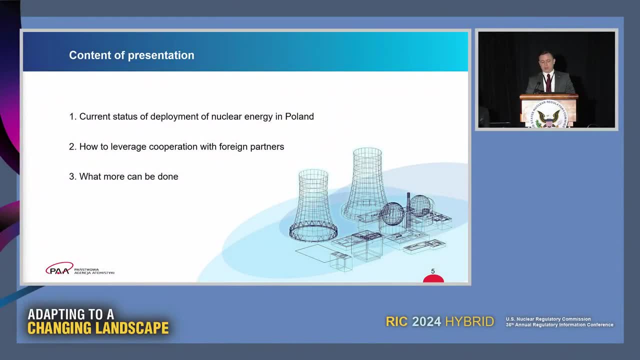 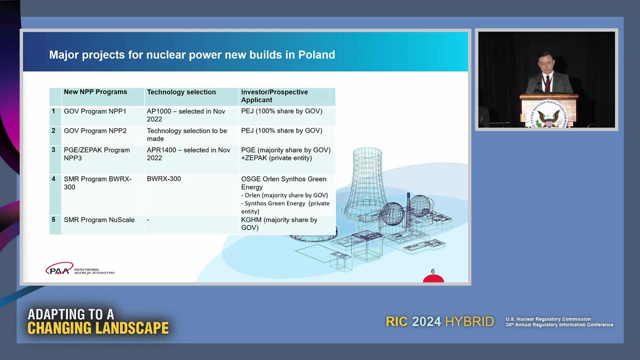 energy in Poland and I will give you some example: how to leverage cooperation with the foreign partners and what more can be done. Well, on this slide you get some information on the major projects of the new builds in Poland. There is a government. 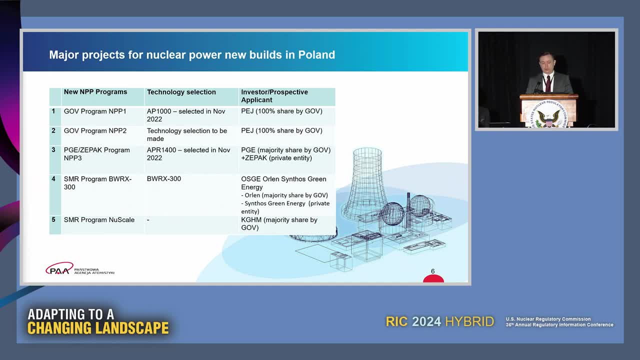 Polish nuclear power plant. There is a power program which envisage two nuclear power plants with the large, large light water reactors. The technology for this one has been already selected in November 2022.. That's going to be Westinghouse design AP1000.. 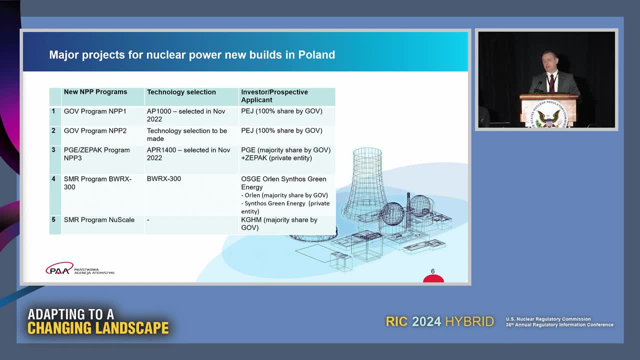 There is envisage to build a second nuclear power plant under this program, but the technology has not been selected yet. Okay, So the program is based on the APR1400 Korean design. but there is also a big great interest in SMRs in Poland and actually there are at least two main SMRs initiatives led by the 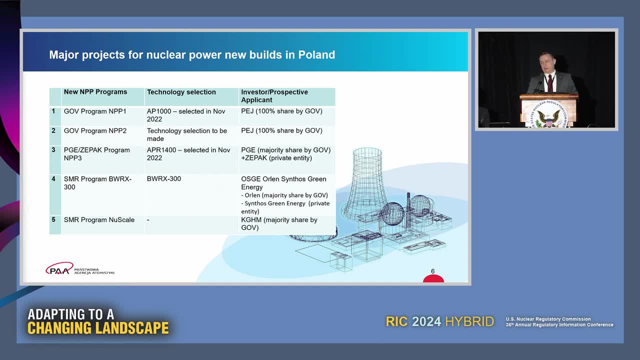 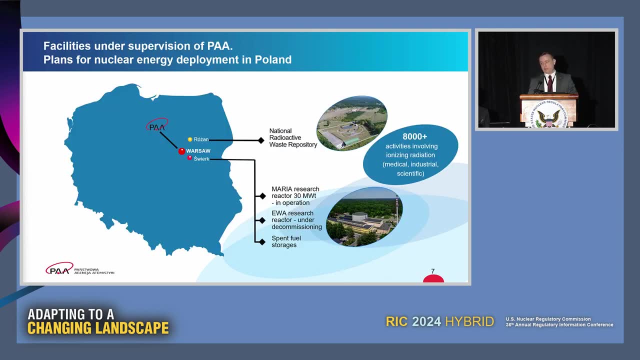 Polish business, and they are based on the BWRX300 and the new scale designs. Well, as of today, Poland has zero nuclear capacity. Our main nuclear facilities is research reactor Maria, with a thermal power of 30 megawatts. 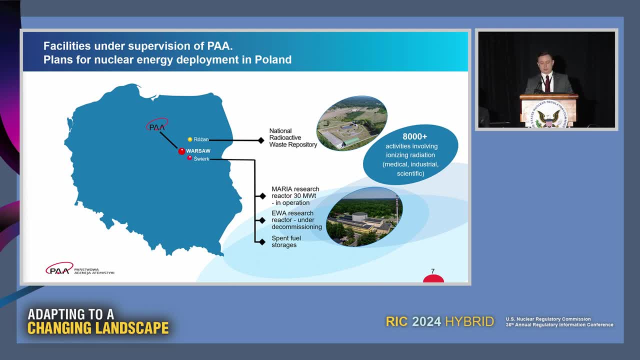 focusing on the production of radioisotopes distributed to a large number of countries in the world. The second research reactor, EVA, is under the commissioning. On the material side of house, we regulate over 8,000 activities involving use of ionizing. 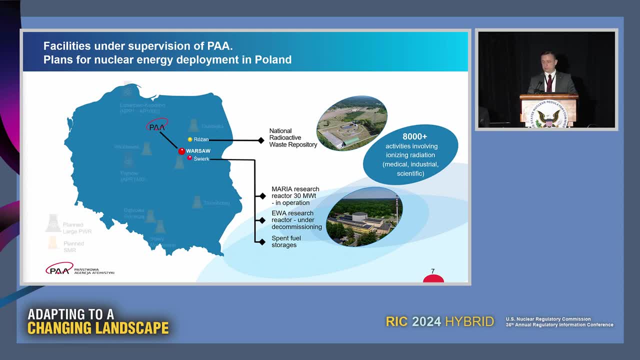 radiation in medicine, industry and science. Okay, So, as you can see, there is a quite big interest in introducing nuclear power in Poland. On the map you can see potential sites for the new builds and the one which is at very 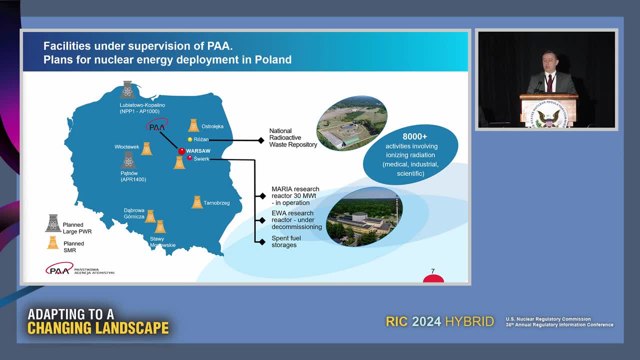 top of the map close to our sea, which is called Lubiatowo-Kopalina. this site has been selected for the first NPPL. Okay, So this is the first NPPL AP1000 design, Also in this gray color. in the center of Poland, you will see the potential site for. 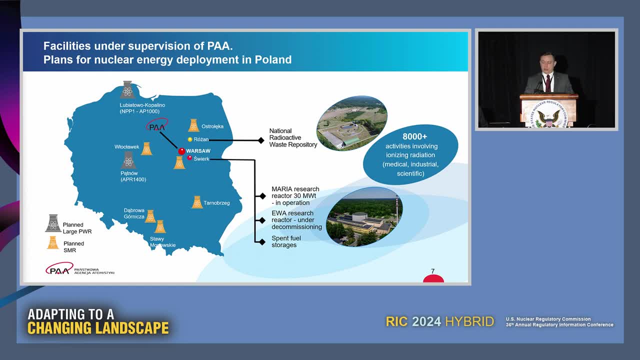 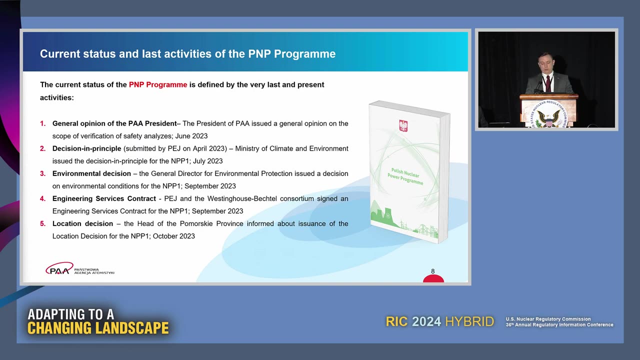 the Korean technology and the yellow-orange color is the potential, are the potential sites for the SMRs reactors. Now I'm going to give you a very quick overview And update of the recent developments of the government Polish nuclear power program. In the last year there has been several decisions made by the regulator and the government. 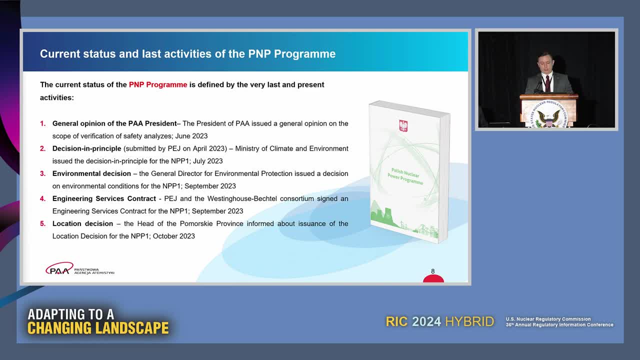 but also by the business or the company which is going to build the NPP. In last June I've issued the general opinion for the AP1000 design, which is the pre-licensing mechanism in Poland to inform prospective utility. Okay, 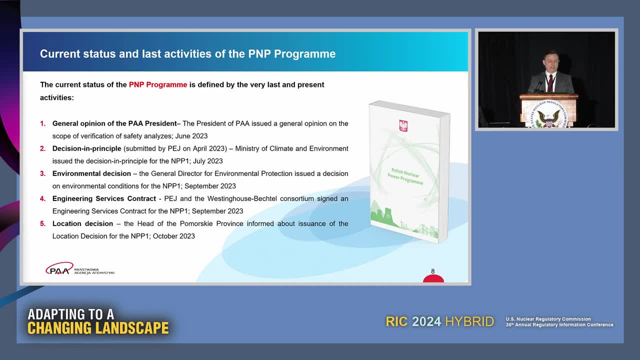 On regulatory expectations and explanations of the safety requirements based on the questions that they may ask or they might be asked by the utility. There were also some several decisions issued by other state authorities. Ministry of Climate and Environment issued a decision in principle for the first NPP that gives green light for 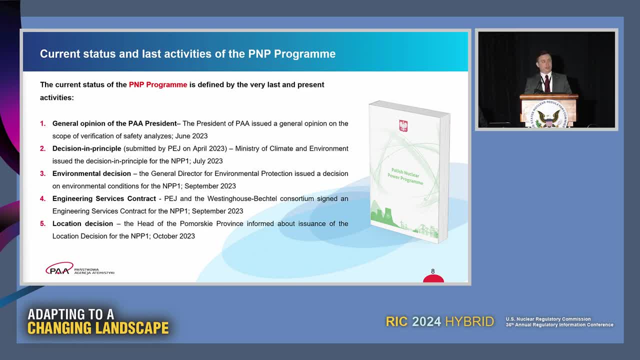 the investment in terms of political support based on national energy and national security decisions. Okay, And finally, the local governor of Pomorskie region issued location decision for the first NPP. that is an administrative prerequisite for any activities on the site. On the business side, Polish utility PJ, Polish nuclear power plant company- they signed contract. 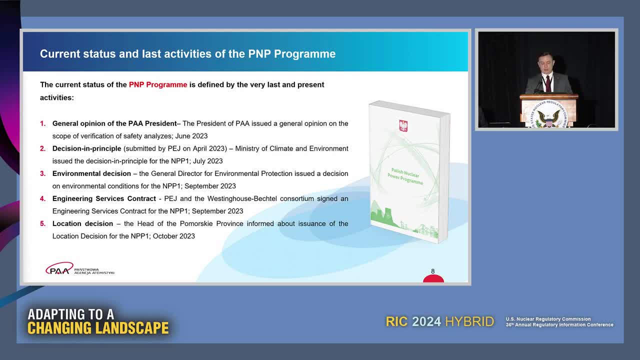 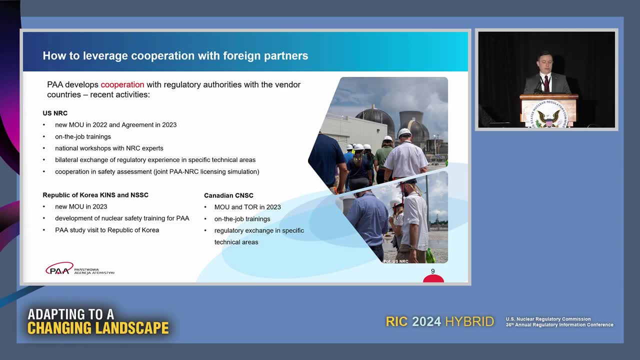 with the Westinghouse and Bechtel on engineering services. So you can see that it is rather ambitious program in Poland Also for PEA to be ready for this important task which is the licensing of the first nuclear power plant. we did a lot but we will continue and we continue to do this in. 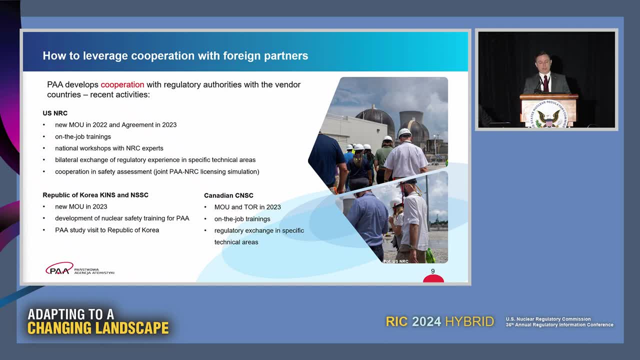 terms of our capacity building. We maintain and develop cooperation with a large number of regulators around the globe and, in particular, taking into account reactor technologies selected for the first investment in Poland. We focus on extending our cooperation with the three main partners: USNRC, Canadian CNSC. 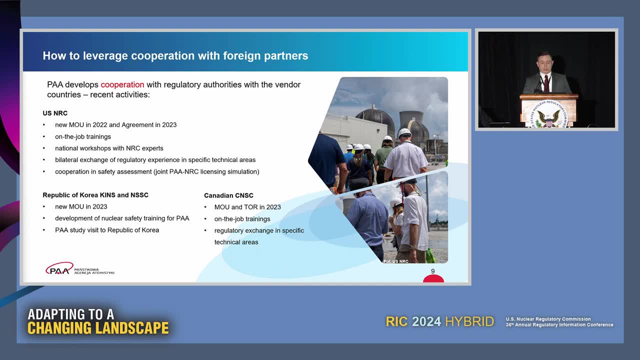 and Korean NSSC, together with the KINZ. Our cooperation is based on a few proven capacity building mechanism. It's an on-the-top training, which are the assignment of the PEA safety specialist and nuclear inspector to the foreign regulators. that technical workshops focus on exchanging. 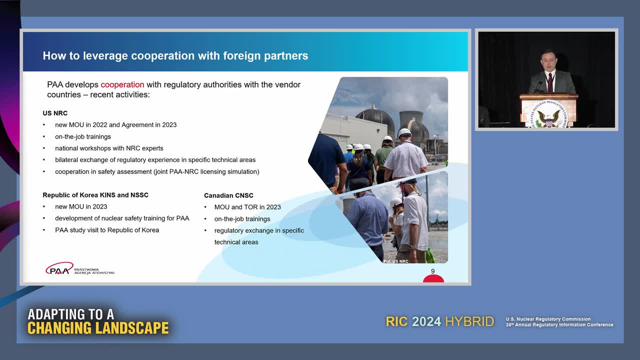 regulatory experience, Like just this year, this February we hosted NRC staff and their contractors to work with us for a couple of weeks to prepare documents which will be used in the licensing process. There is a tailored cooperation on safety assessment. I would like to mention here a successful two-year project with the USNRC under the 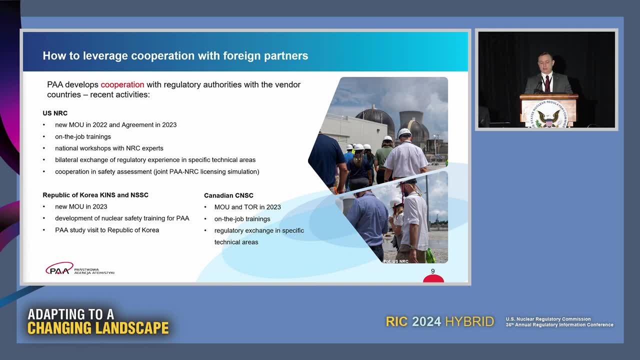 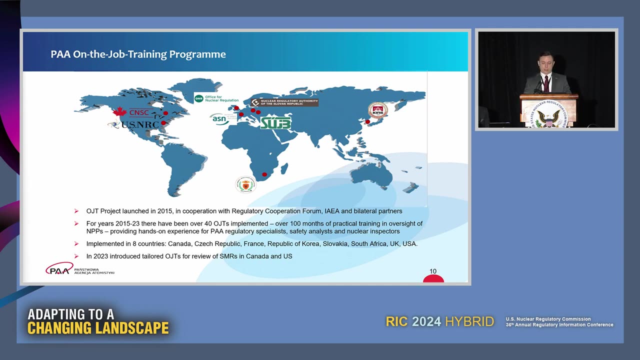 umbrella of IAEA, to simulate licensing process and safety review of construction application that was recognized by the IRS mission as a good practice. Well, I consider the on-the-job training program as a huge support in PEA's capacity building effort. We launched this program in 2015 with the help of several foreign regulators gathered. 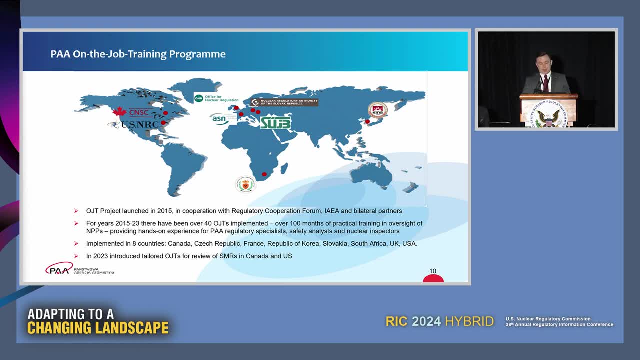 in regulatory cooperation forum that is active under the IAEA. We have already accomplished over 40 OJTs in eight countries, many of them hosted by the USNRC at the TTC in Chattanooga, Abu Dhabi. Thank you. And also as a site visit and technical visit to the Vogel III and IV construction we've 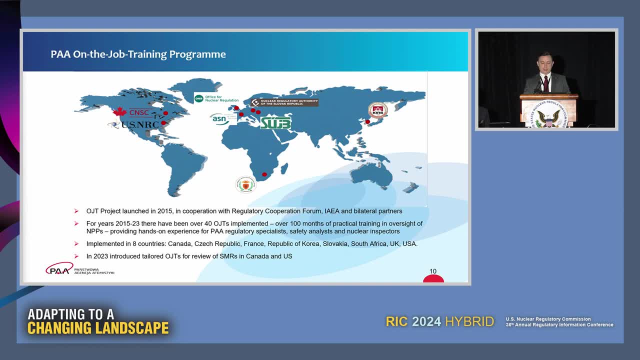 also started implementing OJT focus on SMR licensing. The assignment of our people to foreign regulators gave our staff a great opportunity to get hands-on experience of regulatory work in the field of help them to prepare for performing their regulatory job. when we will perform our work? 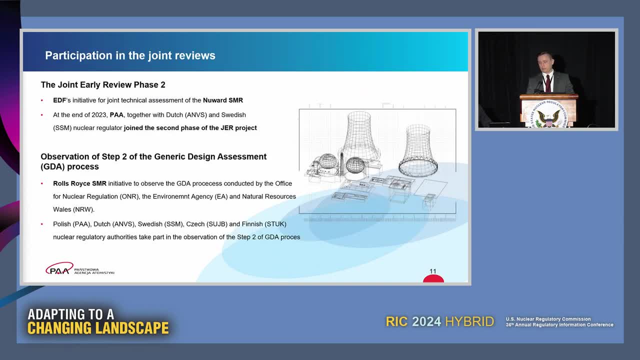 Well, we've joined two initiatives recently which also give us opportunity to be familiarized with the technologies. but also, like I've mentioned, we believe that the best thing, what you can do, preparing for the application, is to get to have hands-on experience. hands-on. 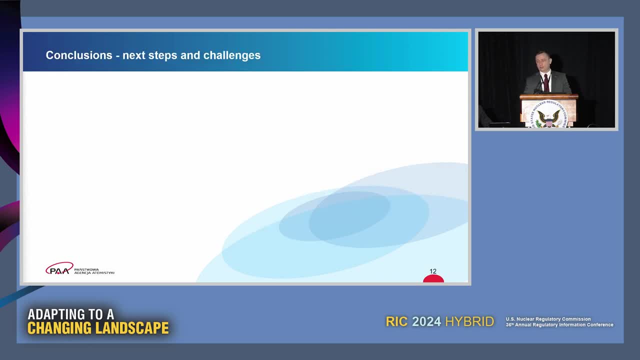 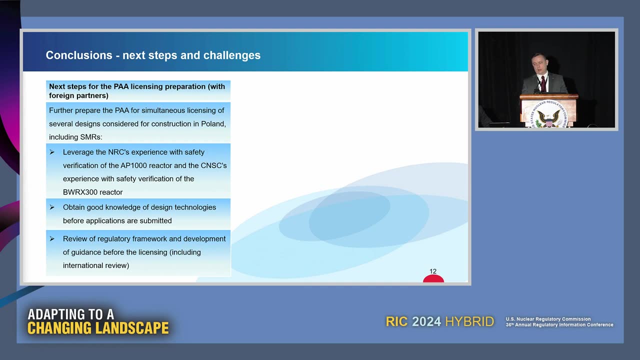 training. So that's what we're trying to do: to work with the documents. Well, as a conclusion, our main challenges that we are facing is to have a simultaneously license more than one application. That's a big challenge. Our original assumption was to have the same technology under the Polish nuclear power. 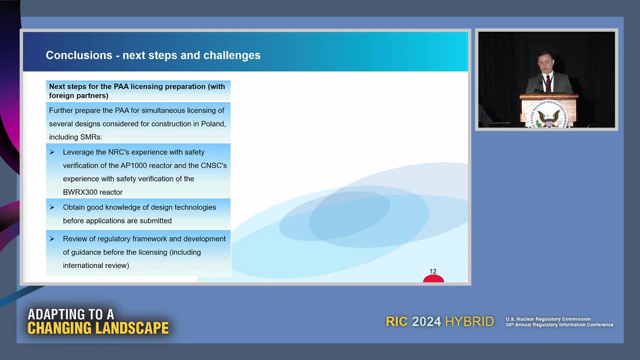 program. Right now we have like more than four new builds, projects that have been developed in Poland. So we adjusted our approach and capacity building to be ready for what lies ahead. Well, international cooperation, especially with the US, NRC and CNSC, is crucial in our 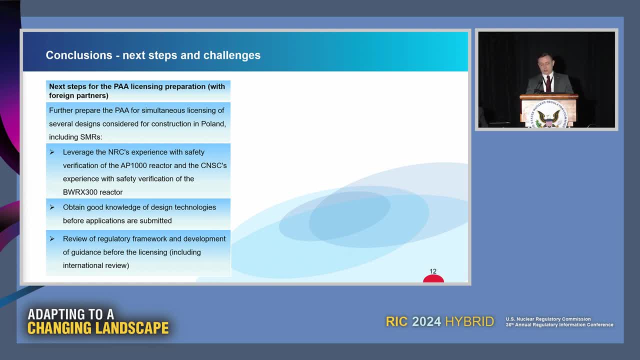 efforts to achieve full regulatory readiness. We are working to obtain good knowledge of design technologies before applications are submitted. Secondly, we also review our regulatory framework And in this way we are using IAEA safety guides and requirements to develop, to update. 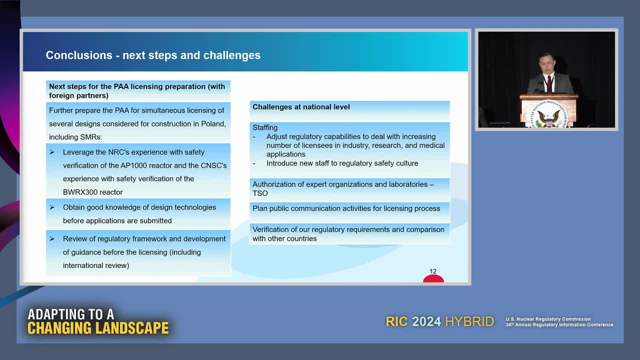 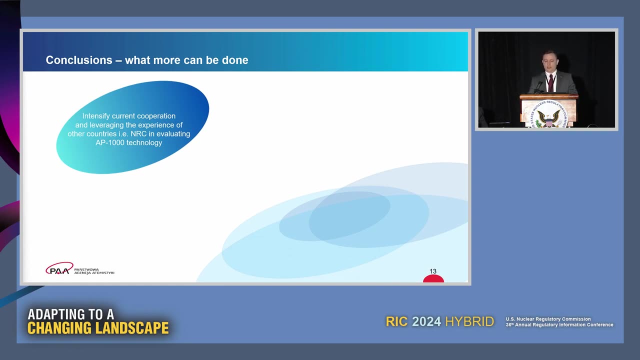 our current legislative framework. What are the next steps? Well, we will continue intensifying current cooperation and leveraging the experience of other regulators, like US NRC, to use pre-licensing technologies. So we will continue to use pre-licensing technologies. 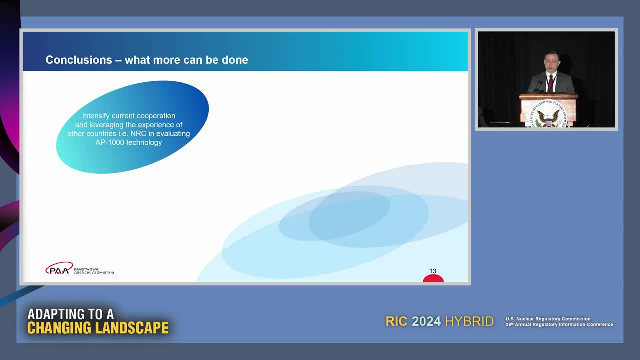 This will be done through a pre-licensing period as much as possible to prepare ourselves for incoming application. We need to remember that once the application come we will be on the clock, but we can somehow extend time available by making best use of time that we have in the pre-licensing. 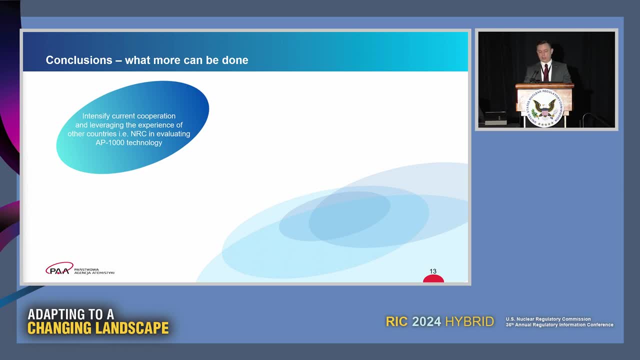 phase, PEE will continue to join verification with other regulators on the safety of selected technical solutions in framework of the pre-licensing or licensing, as a part of the process of strengthening regulatory readiness. in some areas we are also we are also starting to share. 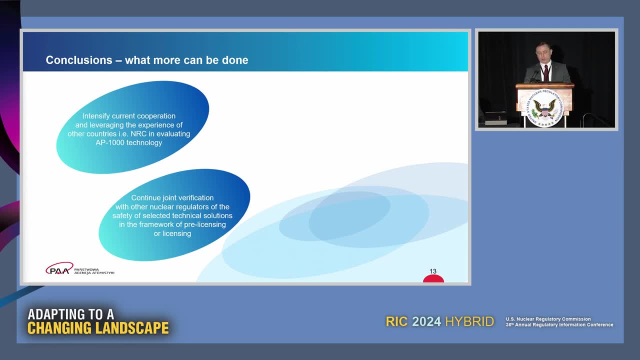 our experience and knowledge with other regulators, including other embarking countries like members of the RCF. well, finally, I'm gonna touch the harmonization of the nuclear regulatory requirements and, as I mentioned, our approach is that. well, while using the IEA safety standard, we think we are in a 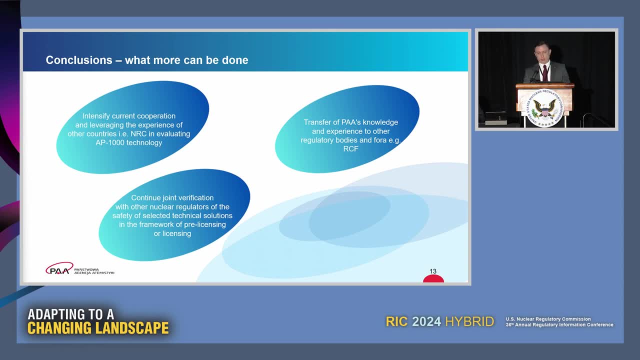 more harmonized way and be being ready to also make changes in the best possible ways. best practice and use best practices which are in the in the world. well, with that, I think I'm a little bit over the top the time, unfortunately, but I want to emphasize that we are not alone in the 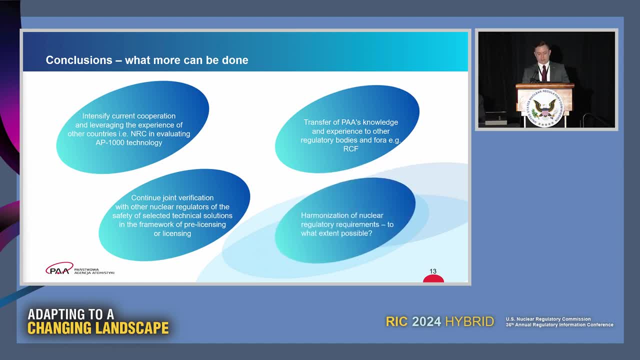 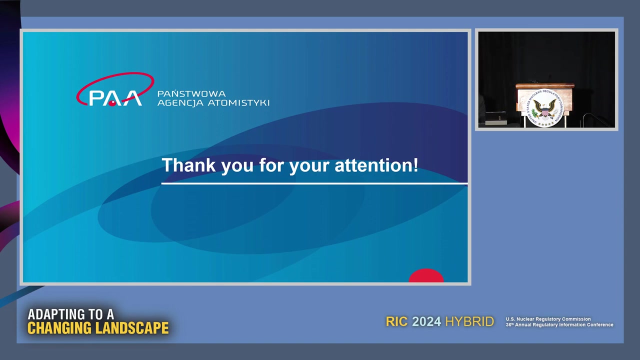 process and, like chairman Hanson quoted, the optimism is a force multiplier and we are very looking forward to further cooperate with with the all the regulators, and especially to get the best that we can take from your experience and that. thank you very much for your attention. Thank you very much, President Glowacki, really appreciate all of your remarks. 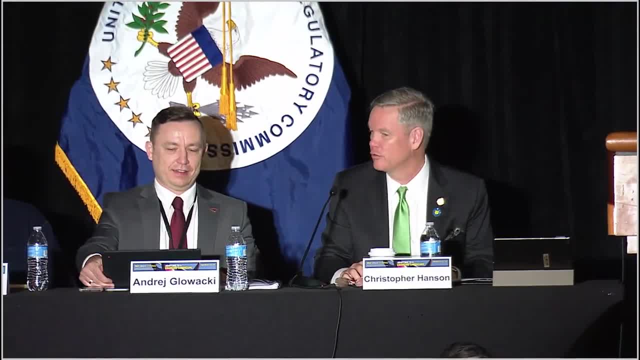 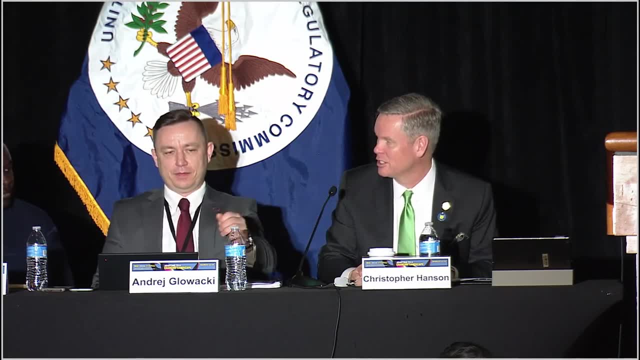 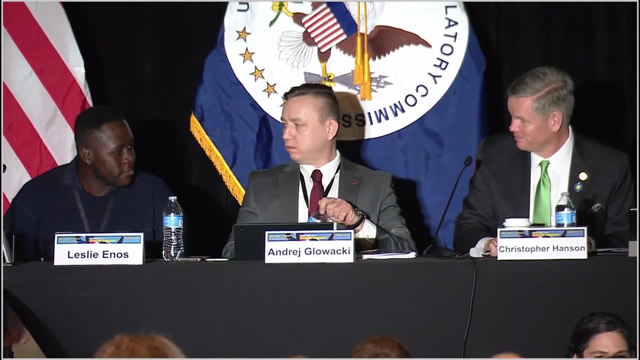 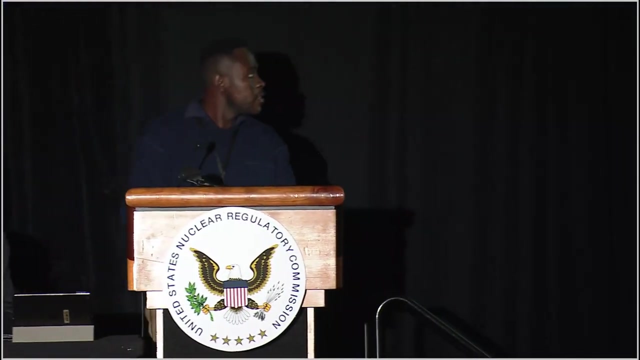 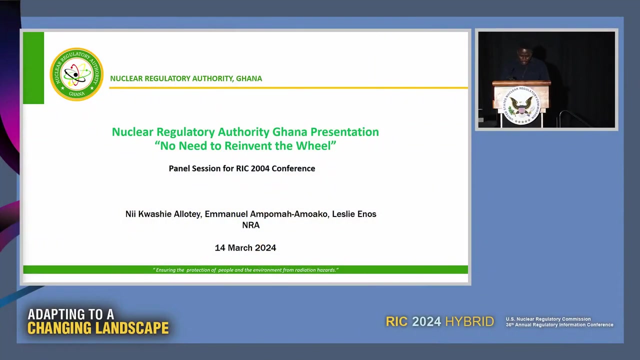 really fascinating overview of the activities that are going on in Poland. next I'll hand the mic over to our friend, Mr Enes, from the Ghanian Nuclear Regulatory Authority, from the Ghanian Nuclear Regulatory Authority, and we look forward to your remarks. good morning, chairman Hansen, my fellow. 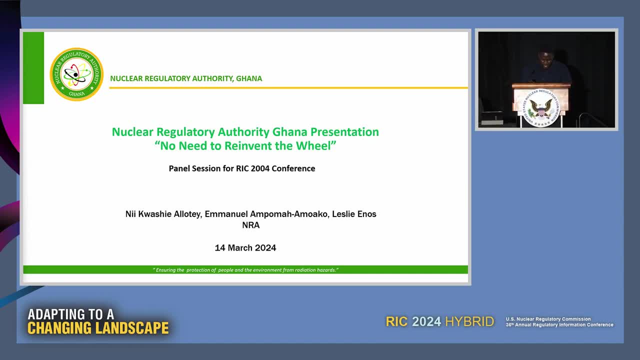 panelists, ladies and gentlemen of the conference, I would like to thank Tim and Hansen for giving me the opportunity to give present Ghana's perspective on a subject at hand. I am here today to replace the director of nuclear installations of the Nuclear Regulation Authority of Ghana. unfortunately, he 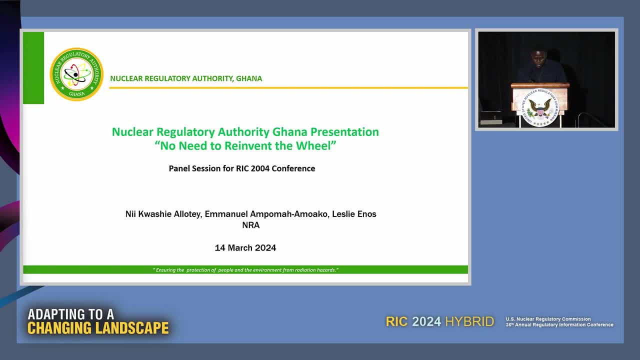 wasn't able to be here today, so I'm hoping that I would help provide our perspective in a very good way. so my name is Leslie Enos and I am a stress analyst of the Nuclear Regulation Authority of Ghana, and today's presentation I'm going to be talking about some few things. I'm 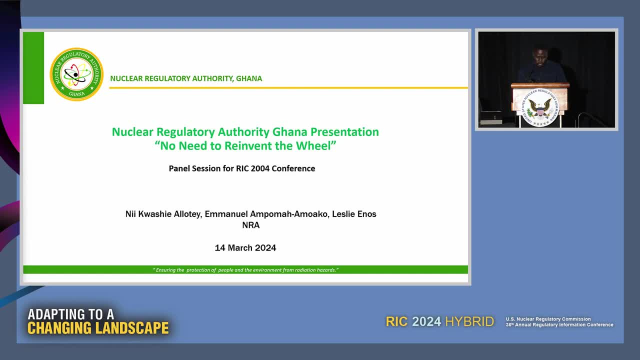 going to give a brief history of the Ghana Nuclear Regulation Authority. then I'm going to follow it up with a brief description of what we do and how we regulate nuclear installations and other radiological facilities. then, halfway around the line, I'm going to give a description of all. 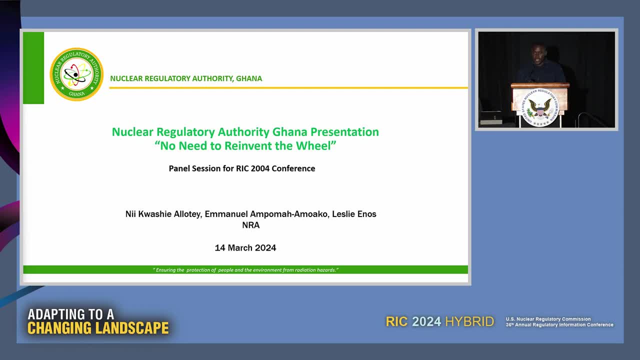 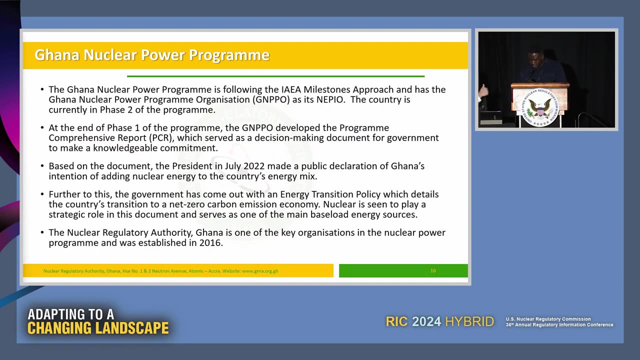 the international corporations we have been engaging so far and some of the challenges that we have faced. okay, so the nuclear program of Ghana was formed by the GNPPO. the GNPPO was formed by the government, which constituted several institutions, some from the various power. 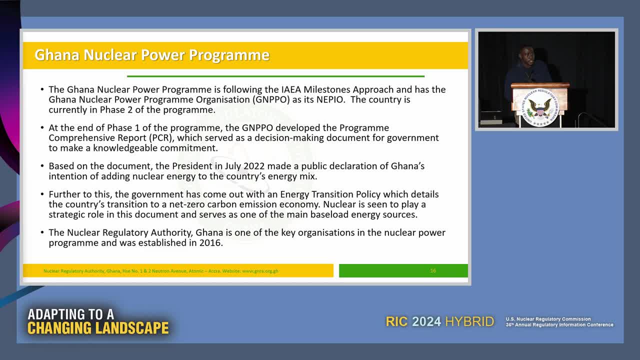 plant companies, the Nuclear Power Institute, the Ghana Atomic Energy Commission as well as the Nuclear Regulatory Authority. So at the end of the phase one program, the GNPPO developed a program comprehensive report And this was the main document which served as a decision-making document for the government. 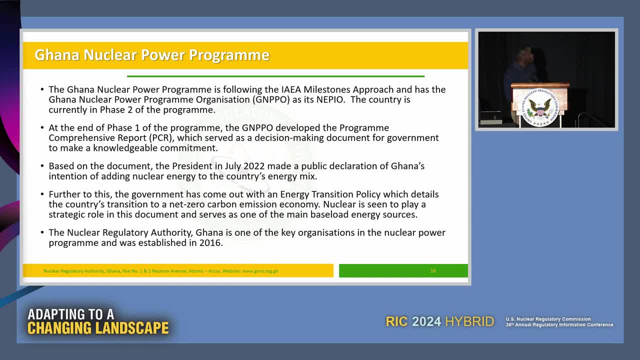 in order to show their commitment in the nuclear power program And based on this document, the President, Honorable Akufo-Addo, in July of 2022, made a public declaration of Ghana's intentions of adding nuclear power to our energy mix. 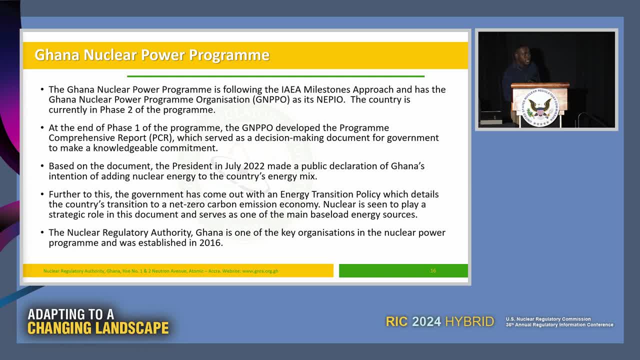 Furthermore, the government also developed a energy transition policy which also details the country's transition to a net zero carbon emission economy. The Nuclear Regulatory Authority was a very vital institution which was formed in the year 2016, which was mandated by the legal framework of the Act which gives us our mandate. 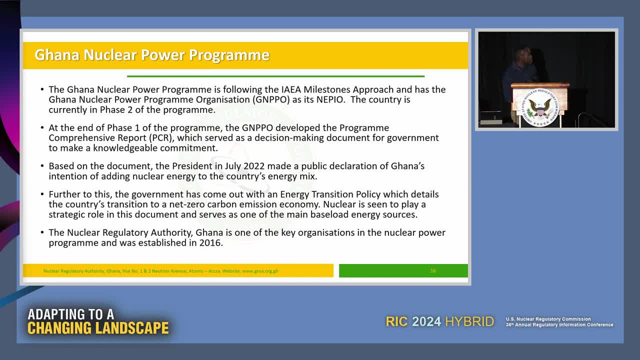 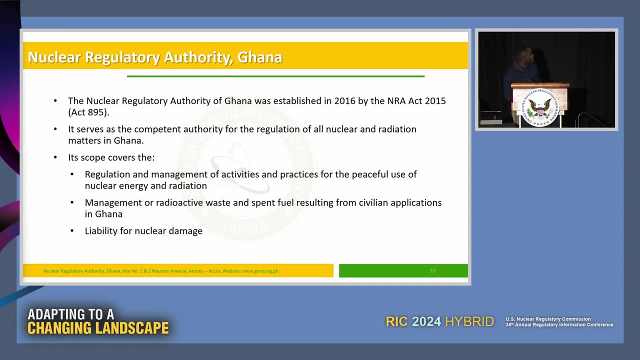 in order to regulate all nuclear facilities and regulatory facilities. Okay, So the Nuclear Regulatory Authority is guided by the NRA Act 895, and the authority is supposed to serve as the competent authority for regulation of all nuclear and electrical matters. So this scopes development of regulations and guidelines. 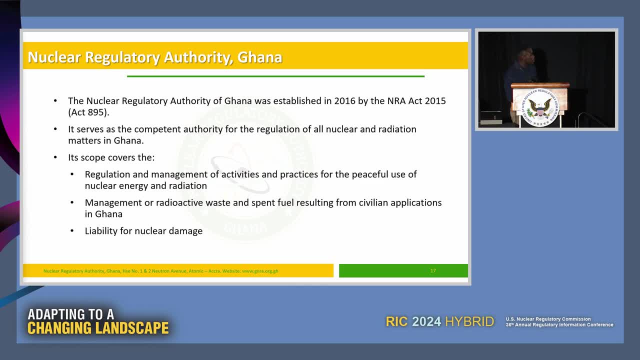 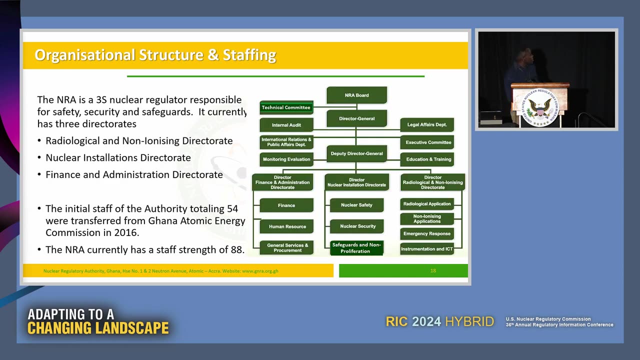 Okay, Thank you. Next slide. And the NRA Act 895 includes in-depth measures to enable the region to manage in the case of a nuclear accident, from oil gas to industrial energy. This is a brief overview of the NRA. So the NRA has three main branches, which is the Radio-Electrical and Non-Arenalization. 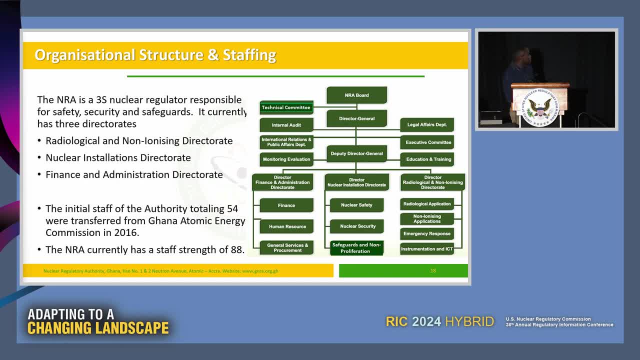 Direct Rate, the Nuclear Installation Direct Rate and the Financial & Administrative Direct Rate. So, since the NRA is a very advanced organization, the NRA is not just an organization. The authority has currently 88 staff and most of 50% of the staff came from the Ghana Atomic Energy in the year 2060 when the NRA was formed. 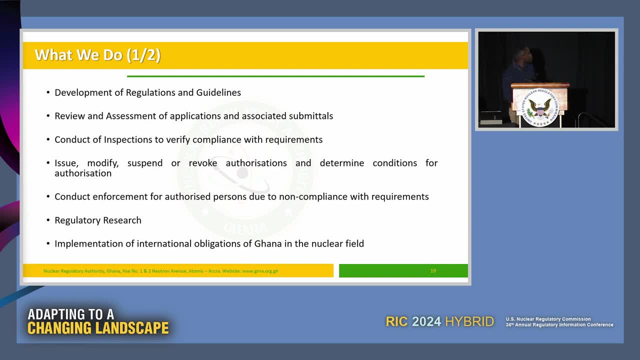 So, like I said before, what we do is basically the same as most regulatory bodies. We try to conduct inspections to verify compliance. we issue authorizations and licensing. we conduct enforcement duties as well: regulatory research and implementations of international obligations of Ghana in the nuclear field. 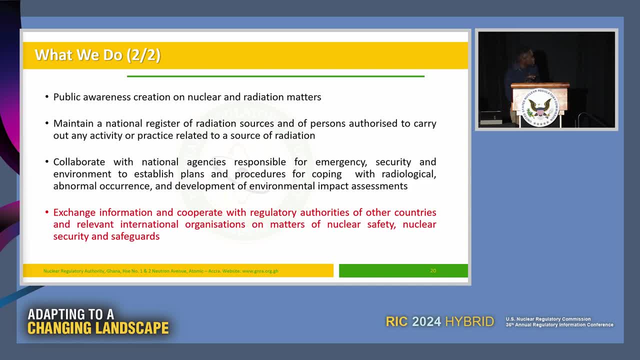 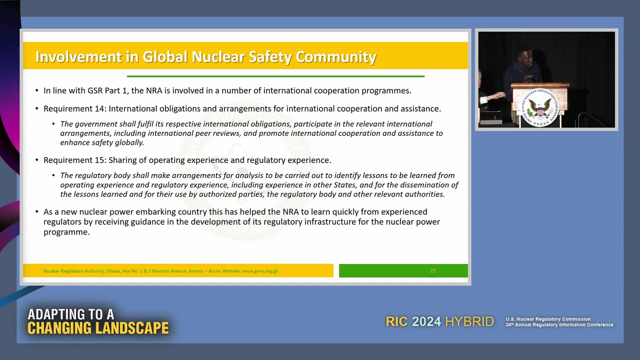 Also, we maintain a national register for radioactive radiation sources. We also try to create public awareness on nuclear and radiation matters In terms of our global nuclear safety community. we follow the IEA's General Safety Requirements, Part 1,, and this mandates us that we should have international obligations. 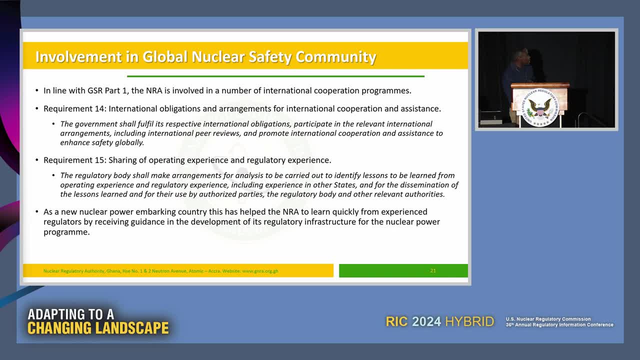 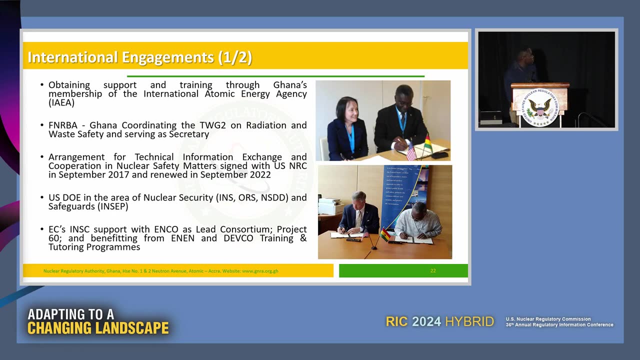 We should have international obligations and arrangements for international corporations and assistance, And also we should be able to share operating experiences and regulatory experiences among other member state countries. Thank you. Through the work of our senior management, we have been able to engage with other international partners and been able to sign agreements with certain member states. 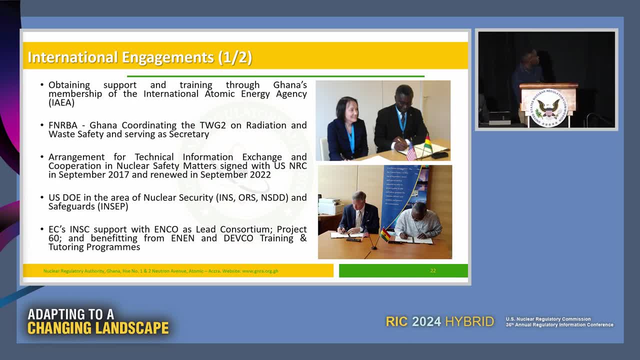 So Ghana. Ghana is part of the FNRB and also is receiving help from the US Department of Energy in the area of nuclear security, And also signed an MOU with the European institutions such as the INSC and ENCO. 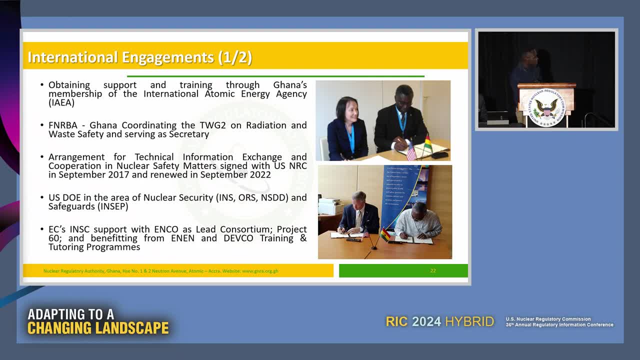 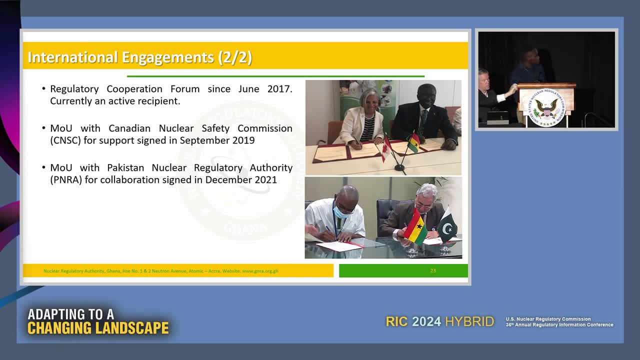 And with these institutions, we are benefiting from trainees and tutoring programs. So also, Also, we have an MOU with the Canadian Nuclear Safety Commission, which was signed in 2019 of September, and with the Pakistan Nuclear Regulatory Authority, which was also signed. 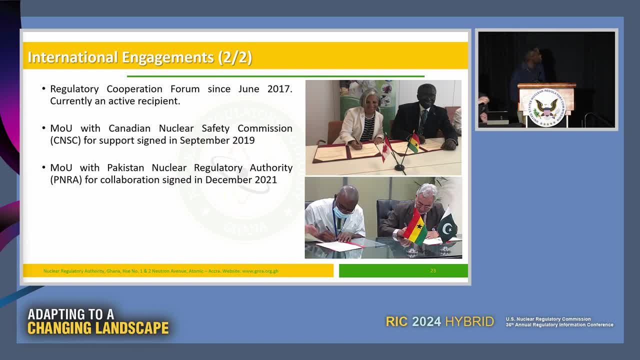 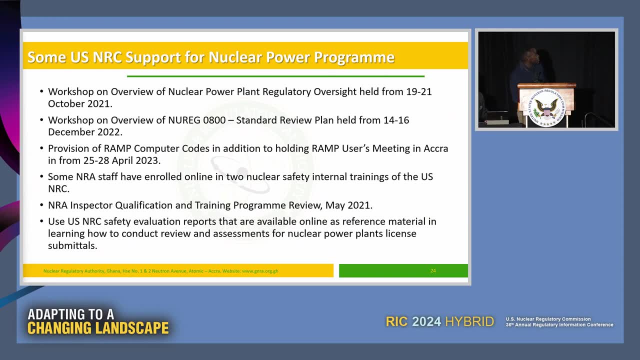 in December 2021.. Some more on the NRC support for our nuclear program. We are privileged to receive a lot of help from the US NRC and these are just a few that I would like to mention. So I was part of the workshop on the overview of NUREC 0800, because we were trying to develop 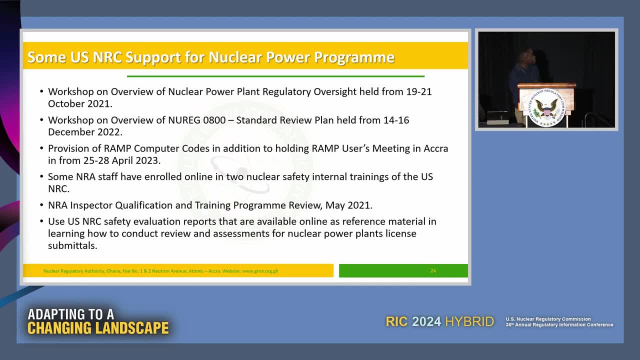 our standard review plan and this was held in Accra between 14 to 16 December of the year 2022. And also we were also given some RAMP computer course training in April 2023. And the NRA Inspector Qualification and Training Program review took place also in. 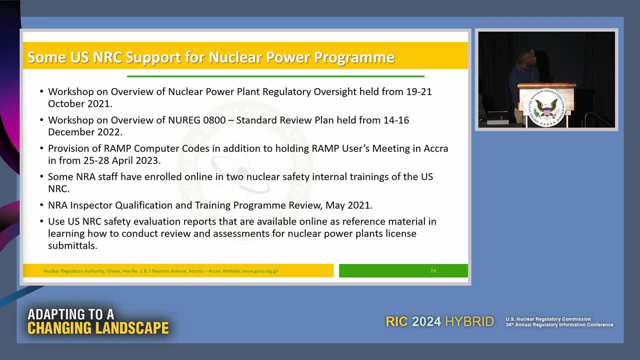 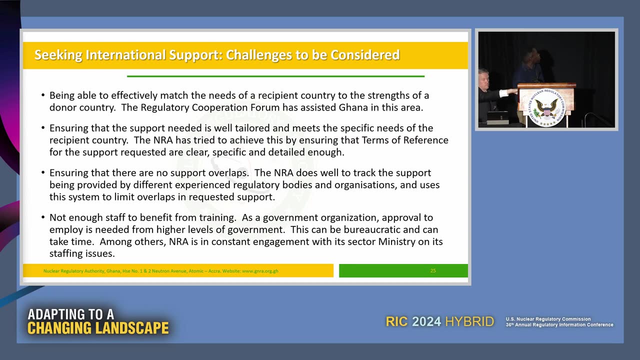 Michigan, May 2021.. And, lastly, the safety evaluation reports that are available online is used as a reference, also in order for us to help us develop ours as well. More on the international support: We are having some challenges so far, and just to mention a few, 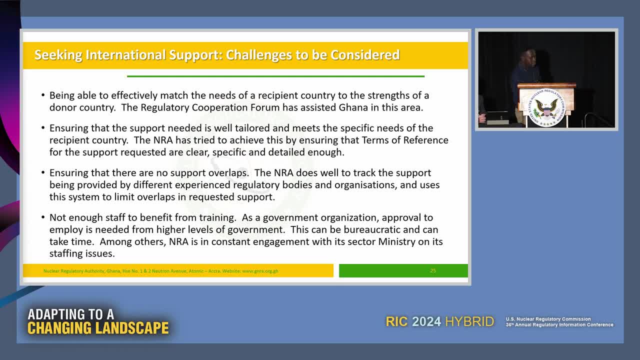 We are having some challenges. We are having some difficulties of staff, shortage of staff and, because it's a government organization, we need permission from the government to employ. So we are hoping that the government increases our staff in order to perform our duties. 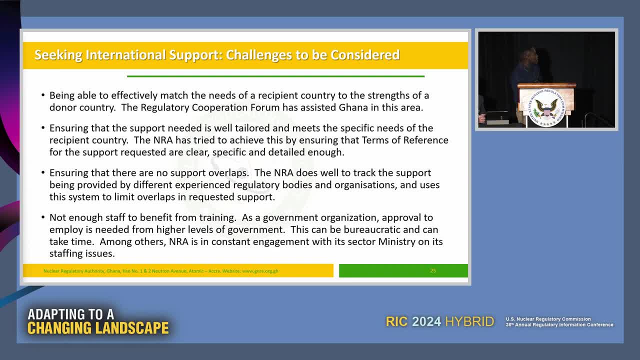 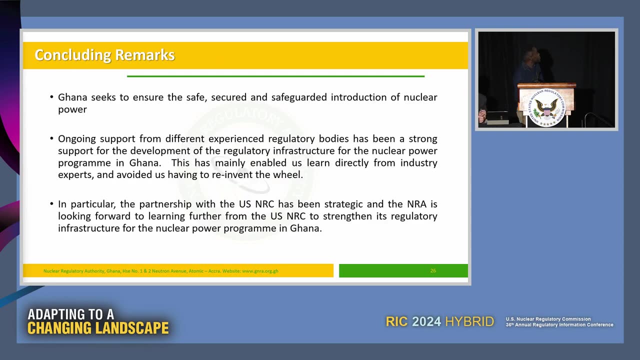 And also we try to ensure that there are no supporting overlaps in terms of international supports that are given to us And also we ensure that support needed is well tailored and meets specific needs of our country's requirements. Thank you. To conclude my presentation, I would like to say that Ghana is seeking to ensure safe. 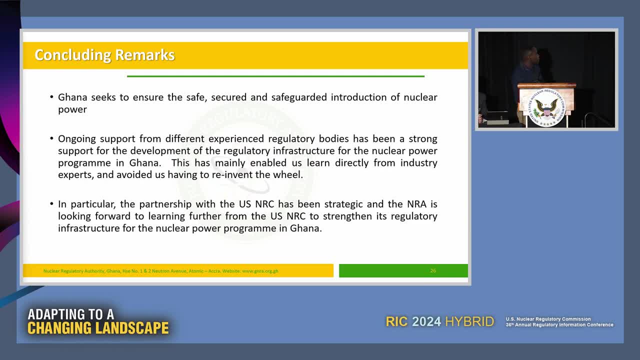 and secured and safeguard introduction of nuclear power And there is ongoing support from different experience regulatory bodies And we are also in particular in which partnership with the US NRC And this has been very strategic And we are hoping We are looking forward to further help from the US NRC as well. 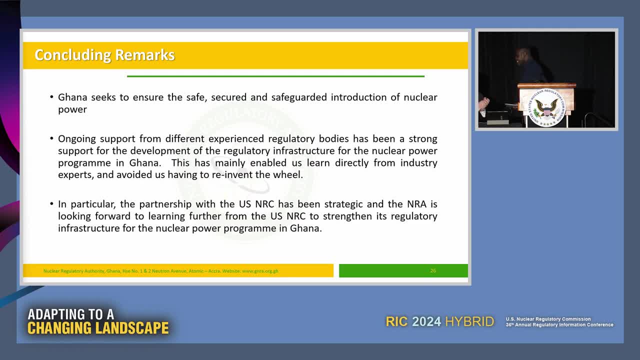 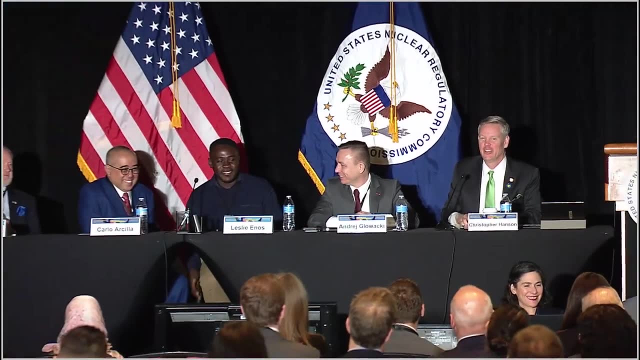 Thank you. Thank you very much, Mr Enos, And we really appreciate your filling in here, I think, with about 15 minutes notice, So really there's a lot of adaptability there. Thank you, Thank you, Thank you. 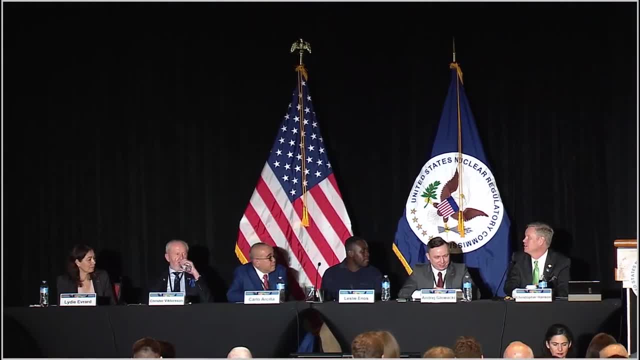 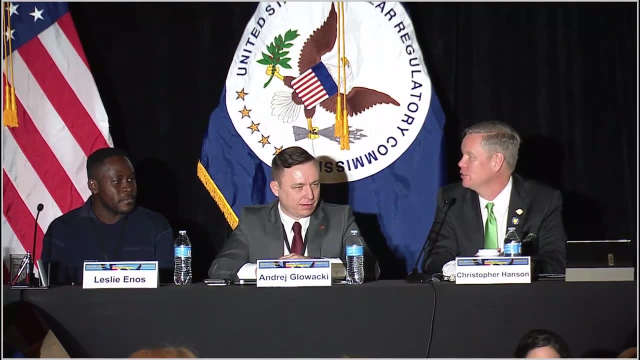 And certainly one of the other things that I think is coming up in Ghana is a peer review mission to kind of review preparatory activities to regulate nuclear energy- I think coming up in 2025. And we look forward to continuing to support that. 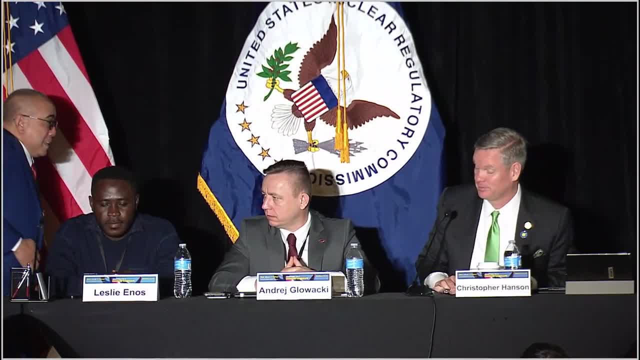 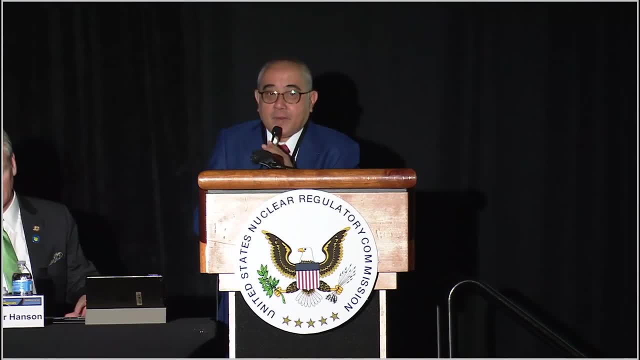 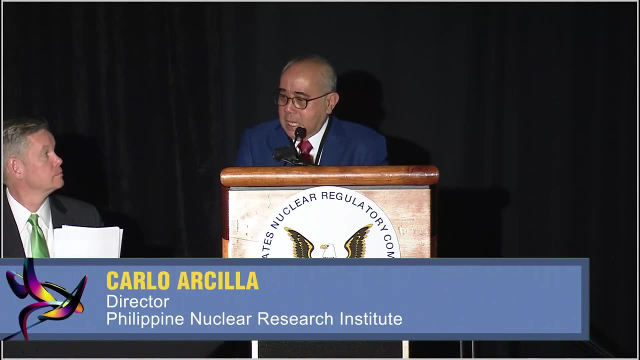 With that, I will hand it over to Dr Carlo Arcea. Thank you very much. Thank you, NRC, for inviting us here. So this is my presentation. We have a long history of nuclear. We had a Triga reactor since the late 50s. 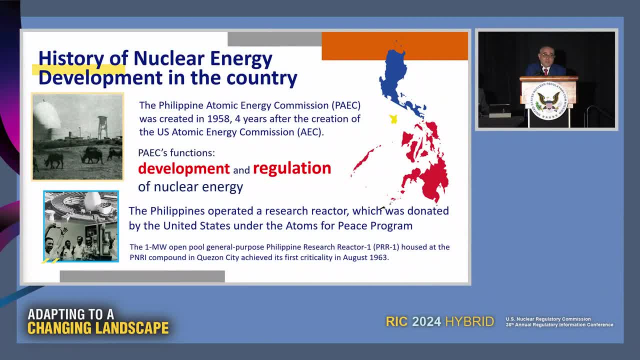 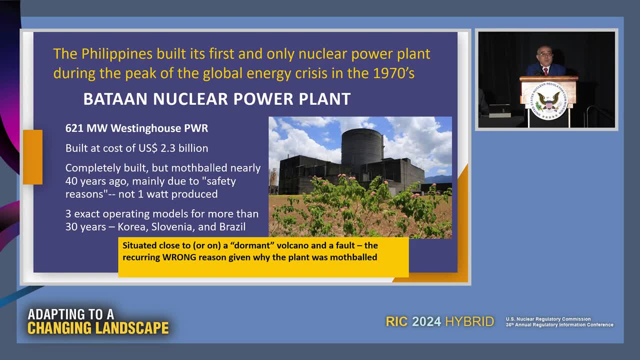 And actually we repurposed that research reactor just recently and made the first subcritical reactor made from Triga fuel And we were the first to build a nuclear plant in the Southeast Asian region. And we are the first to build a nuclear plant in the Southeast Asian region. 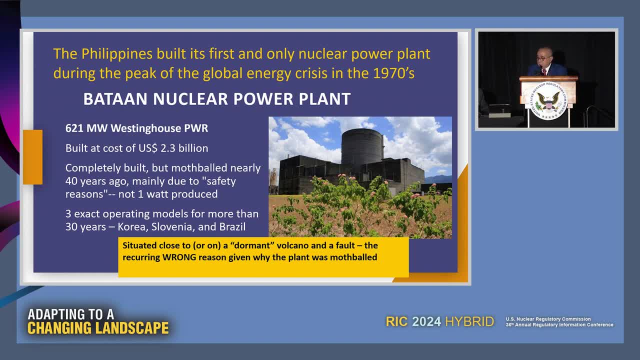 This is the first subcritical reactor made from Triga fuel And we were the first to build a nuclear plant in the Southeast Asian region, a Westinghouse PWR, but was never used. It was completed, The fuel was outside, but in 1986, two things happened. 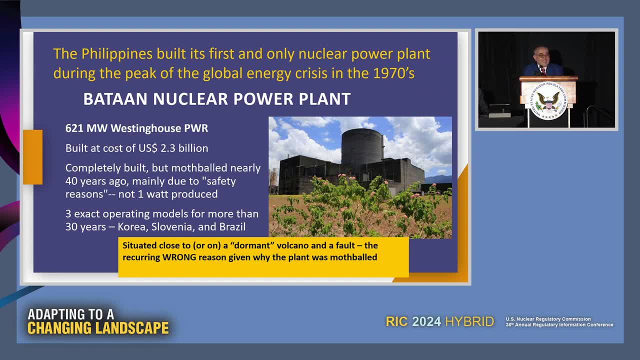 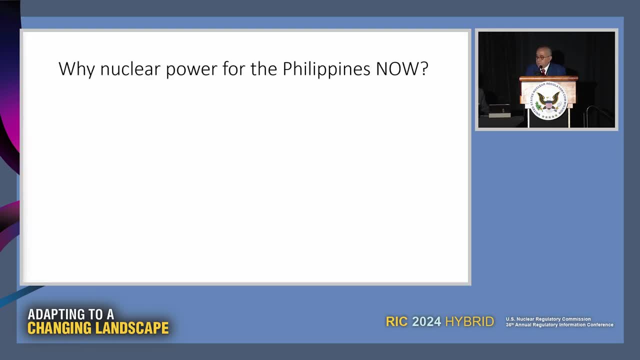 Chernobyl happened and we had a leadership change and that's it. It was confined to the bin and there are three exact models of this operating. But why do we consider nuclear power now? We have very expensive electricity rates, the most expensive in Asia per capita. 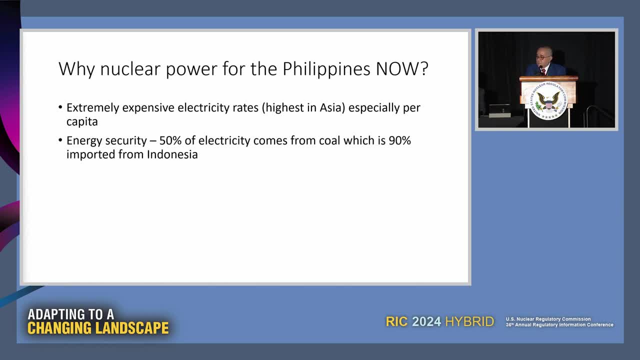 Fifty percent of our electricity comes from coal, which is 90 percent imported, and then 20 percent from a depleting gas field in the South China Sea, which is a hotbed of problems right now and which provides backload for international renewals. 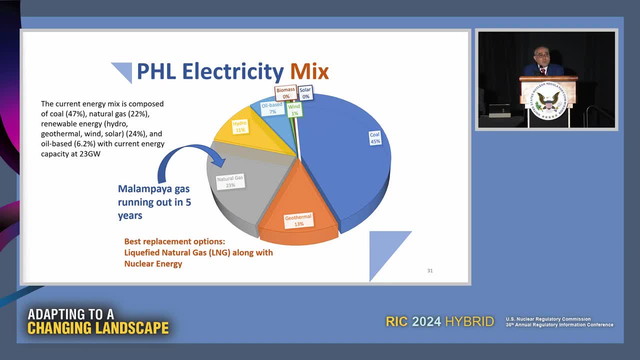 Here is our electricity mix. By the way, we are number two or number three in geothermal, so our renewables is actually not bad as compared to many other countries. But you can see this, The difficulty here: 70 percent of the base load is under threat. 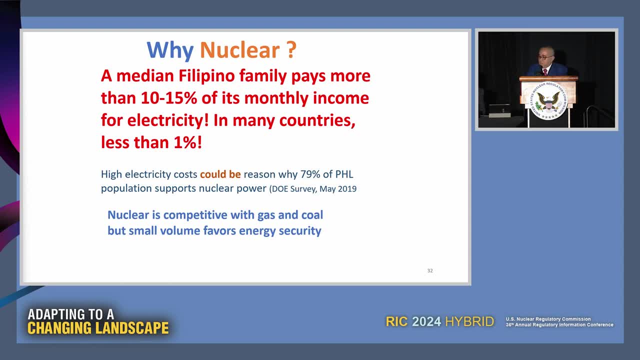 Why nuclear? Because the median Filipino family pays more than 10 to 15 percent of take-home pay. This is an oppressive rate if you compare your electricity rates And there was a survey done in 2019 that 79 percent of the population supports nuclear. 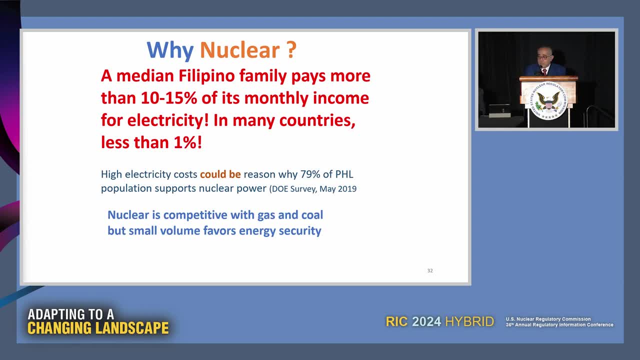 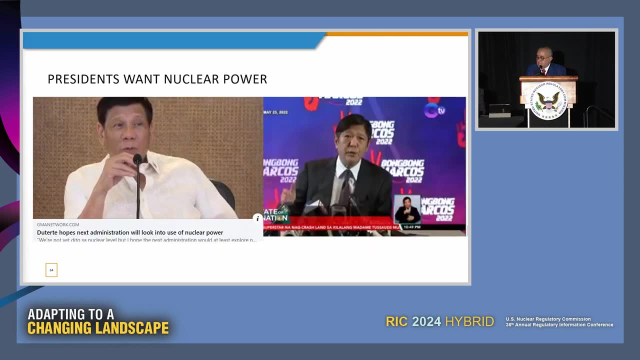 because of the high electricity costs. We were surprised by these results. The national position, one of the IEA 90 milestones, has been signed by a president and the two presidents that we have want nuclear power. The current president, in his first state of the nation, said: we need nuclear. 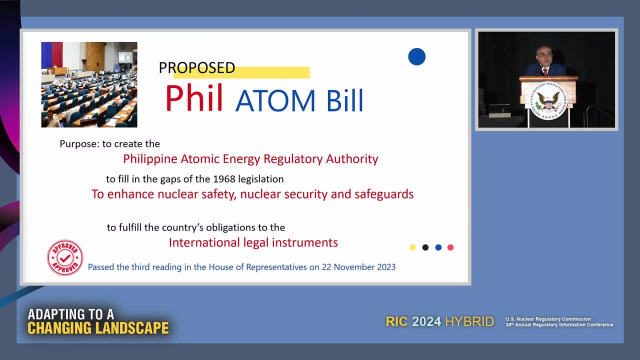 So, and as a result, there is the Philippine Atomic Bill to create an independent regulatory authority. Right now, we are the regulators- I am the head of the regulation- but we're also promotion, And our problem with the research reactor is that we made a reactor and we have to license it. 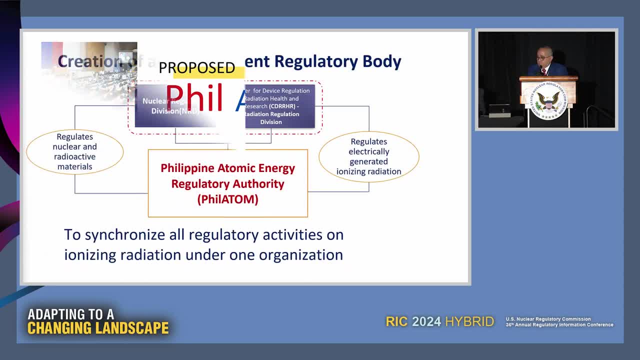 So at least we have to license it. So this is a clear case of conflict of interest. So this is it, and then it will take the X-ray machines come from our FDA and that will be put into a regulatory authority called the Philatom. 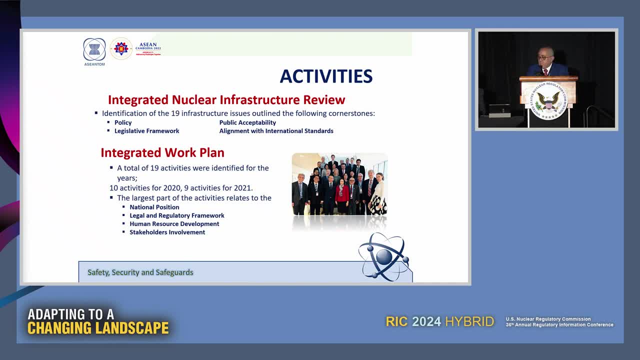 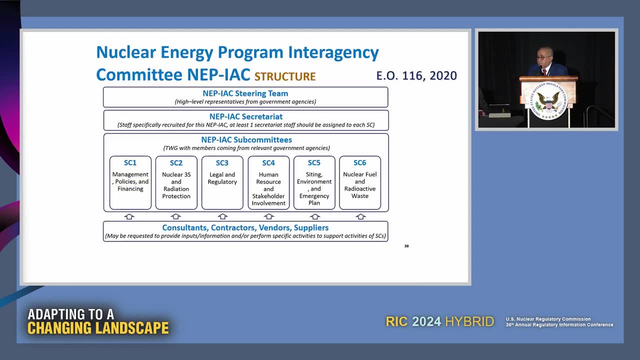 We are following the IEA infrastructure guidelines. We had had an intermission and we will request for another one this year. An integrated work plan was done but was stopped by COVID, And we have an EPIO dividing the 19 milestones into six. 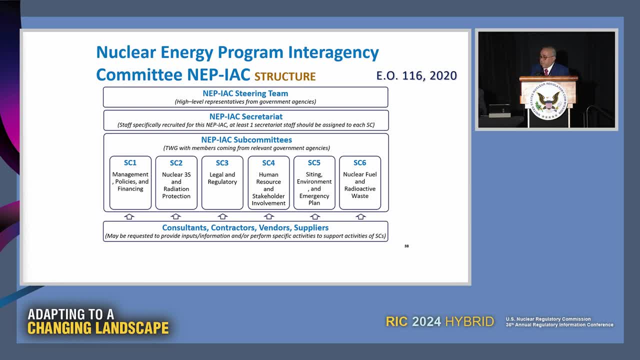 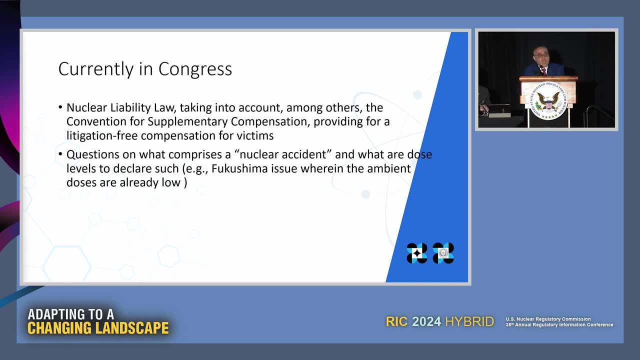 This is the reason why we have to have two or three subcommittees, and this has been very active in the past two or three years And in Congress. actually just this week, as you were here, a nuclear liability law passed the lower house and it's now in the Senate. 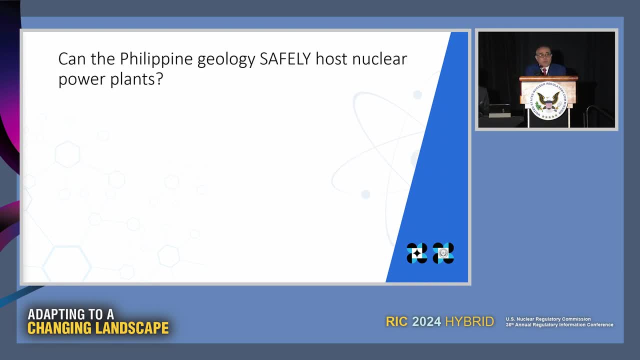 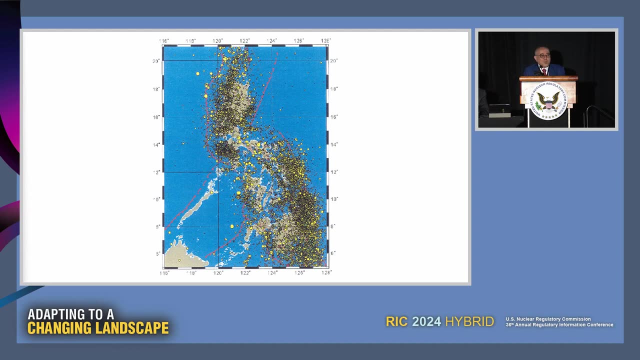 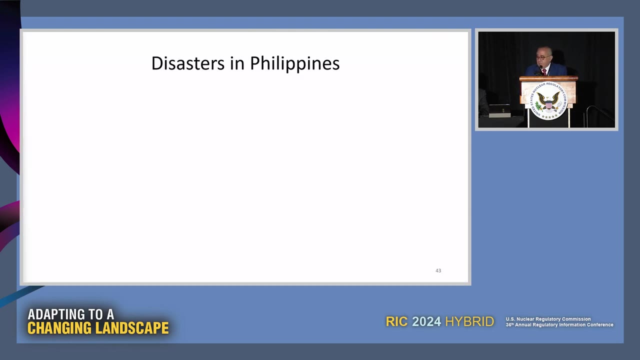 So we will have two bills, a safety law and a nuclear liability law that hopefully will be passed this year. Now people ask me: can we safely host nuclear power plants? Because these are earthquakes, many earthquakes. This is a volcanic eruption in Taal two years ago, So we have many disasters. 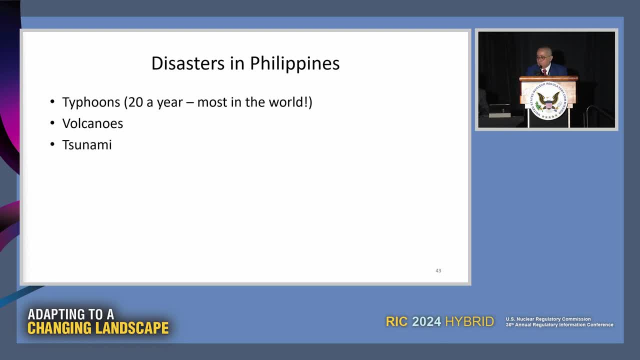 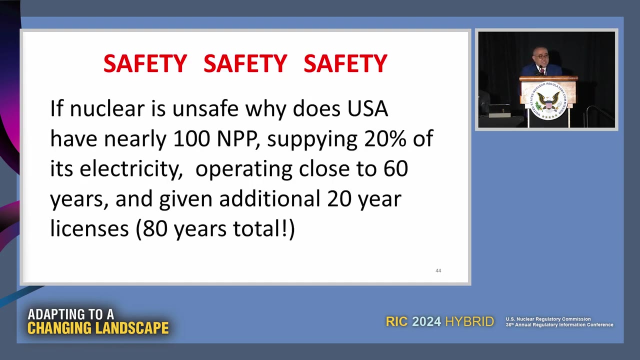 in the Philippines. We have the most typhoons in the world: volcanoes, tsunami, earthquakes, floods, landslides and Anyway. so when people ask me about safety, my answer to that is: if nuclear science, why does America have nearly 100 nuclear plants supplying 20% of 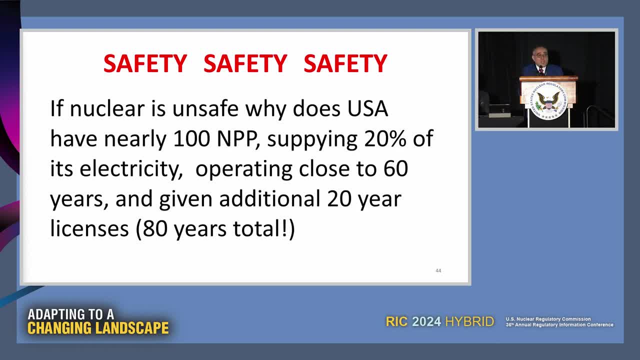 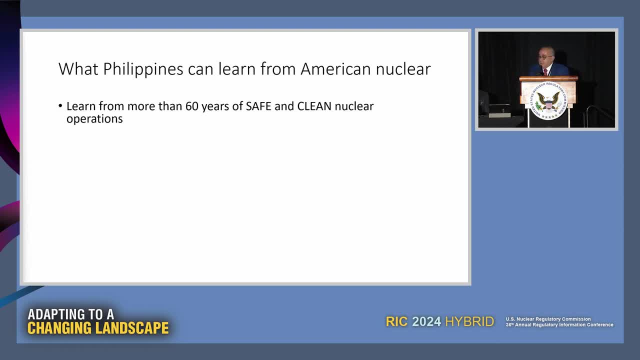 electricity and operating for close to 60 years. So we rely on the American experience- 80 years total- And we can learn many things from American nuclear 60 years of safe and clean nuclear operations. privately owned The nuclear plants in the Philippines will. 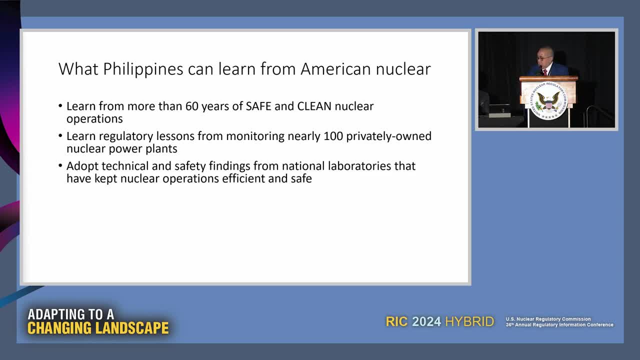 be privately owned And we can adopt safety and technical findings. I'm learning a lot from this conference and from productive Private government initiatives, PPPs And train future manpower. I owe my training to the US. I'm a Fulbright scholar. I did my master's and doctorate here, Thank you. But 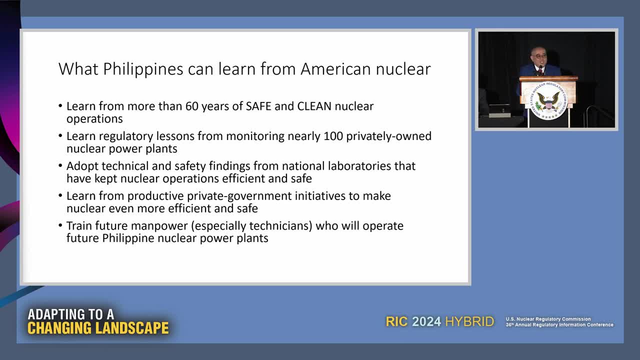 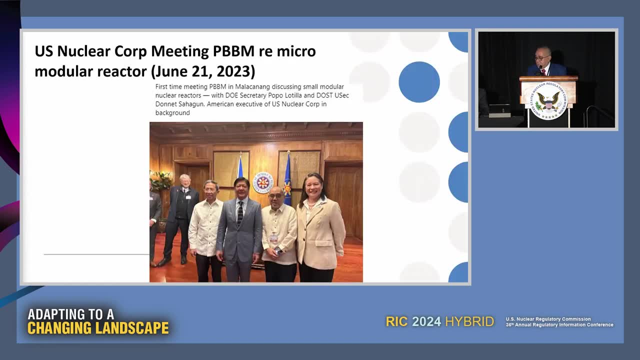 I also tutored black and Hispanic kids in Chicago. I'm proud of those I tutored. They are now productive citizens. Here is our president meeting with US nuclear cooperation. and then This is a small modular or micromodular plants. Our president is technical. I was impressed. 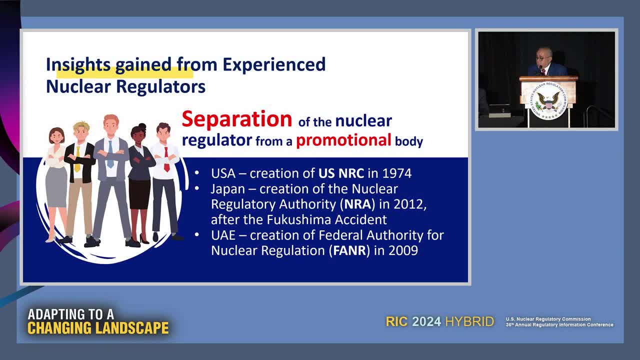 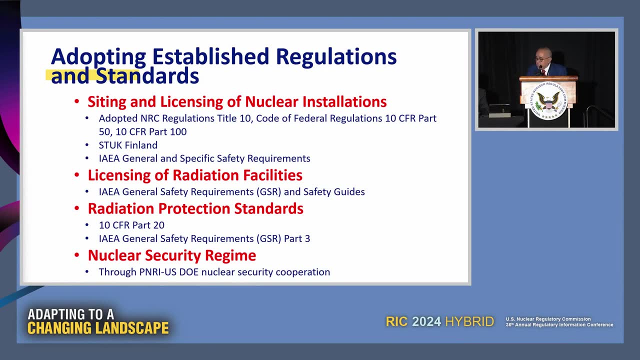 by his questioning And then so So the insight we gained from the experienced regulators, the separation of the promotional body, which is also happening in the US, that's really important. And we adopt and establish regulations and standards for siting licensing protection. 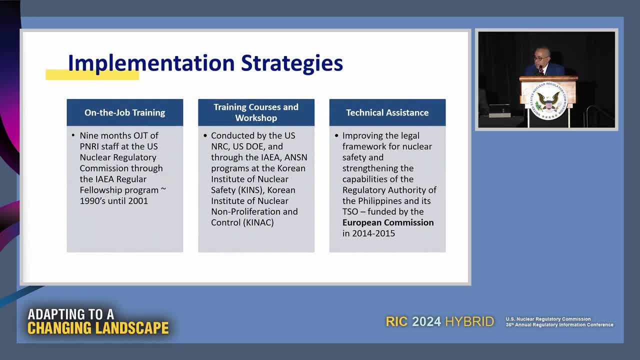 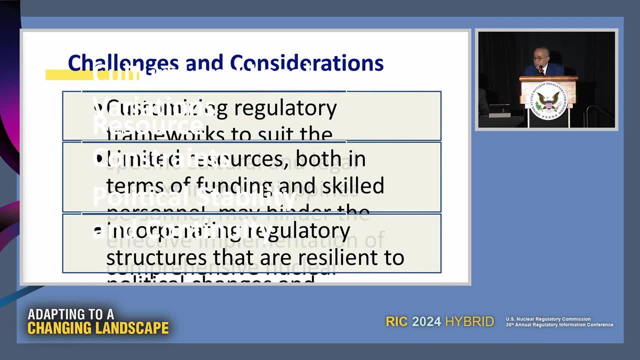 standards And we want to learn more And train. these are the strategies that we want: Training course and workshops, technical assistances And the challenge considerations One when we created the: There are pushbacks from interfering government regulation. Some government regulators don't want to surrender their turf. 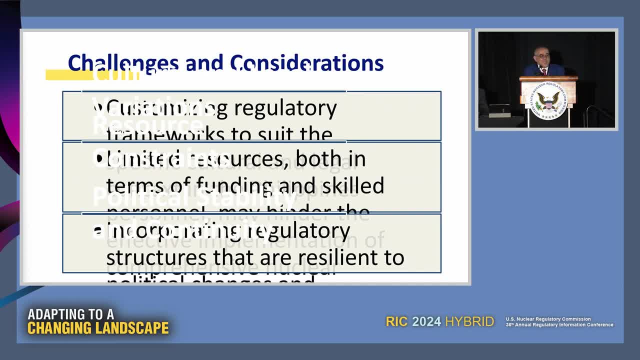 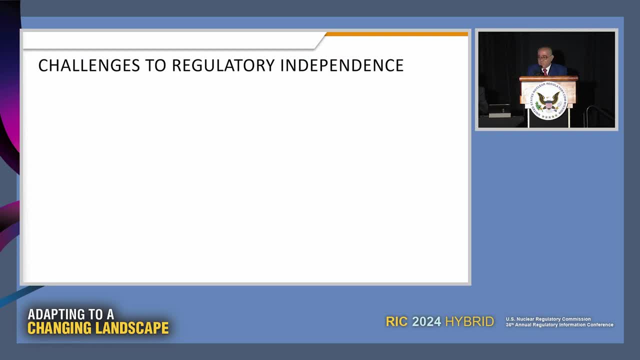 And then there are also some, as I said, the oligarchs and the politicians. Those are the real disasters, by the way. The rest you can live with. So challenges to regulatory independence, this perceived overlapping regulatory coverages. For example, there was an attempt to introduce commercial policy into safety law And we 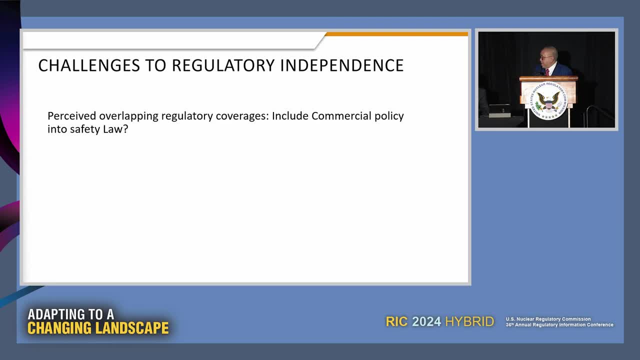 were saying that we had a law review by the IAEA, But some power policies up to now are trying to insert this And fortunately they will be defeated. The nuclear safety law was voted 200 versus 7.. So And how do you fund an independent regulatory body without yearly congressional budgetary? 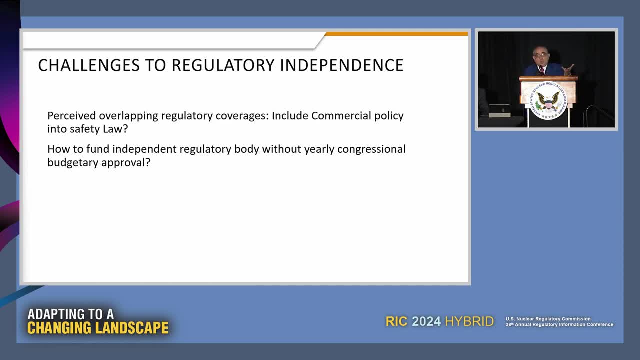 approval Because you can be held hostage by Congressmen who want the nuclear plant approved in their in the jurisdiction. So And we have to integrate into nuclear law the updated convention on nuclear. I'm very proud to say that the CSC Convention for Supplemental Compensation is well integrated. 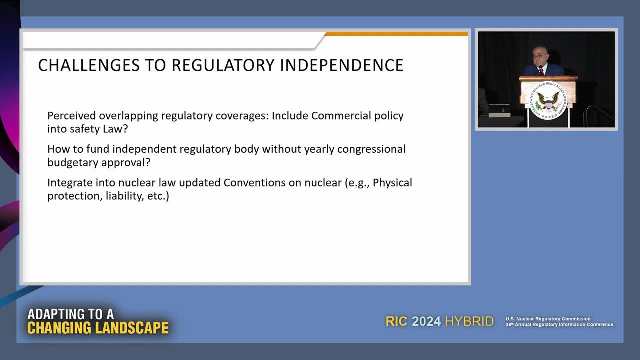 due to our nuclear liability, But there are no other organizations that can do that. So that's what I want to show you: law which is being discussed and will be passed this year. Then how do you select the regulators? That's why I was very curious how the regulators are selected. technical versus legal background. 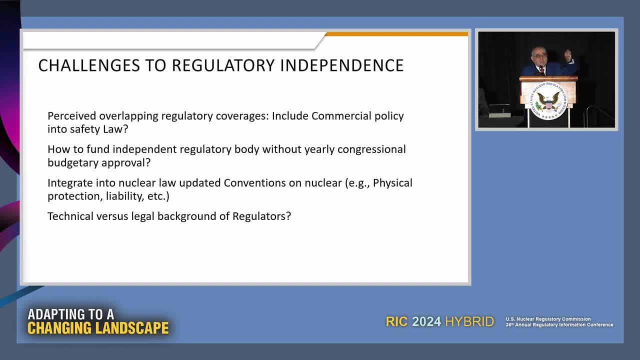 In our law. it says there that the regulators have to have technical background. no lawyers, I mean you can have a law degree if you have a scientific background. Anyway, I have a lot of lawyer jokes I can tell you in the break. 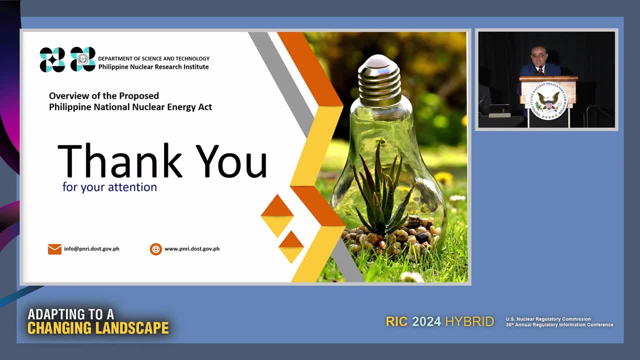 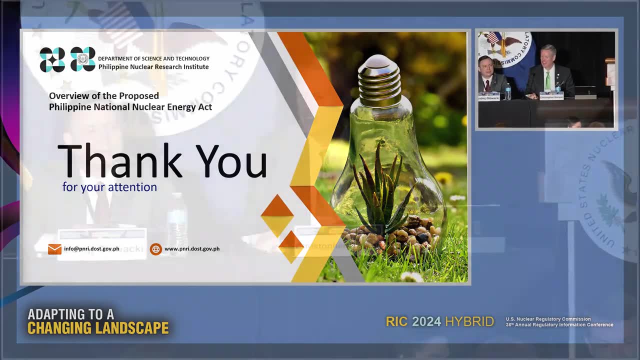 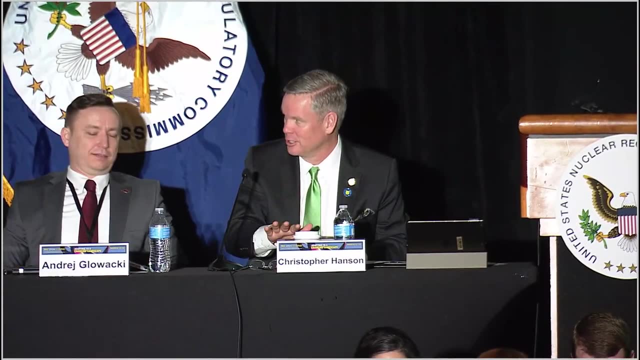 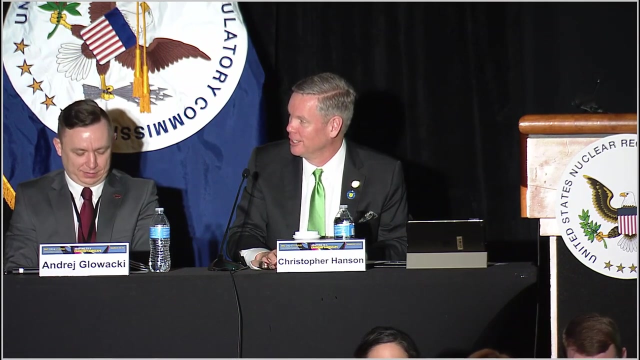 So future prospects are this. So thank you very much for listening. Thank you very, very much, Dr Acilla. We do have both technical people and lawyers in the NRC. We benefit from both. I personally, I mean you- hardly ever travel without a lawyer. 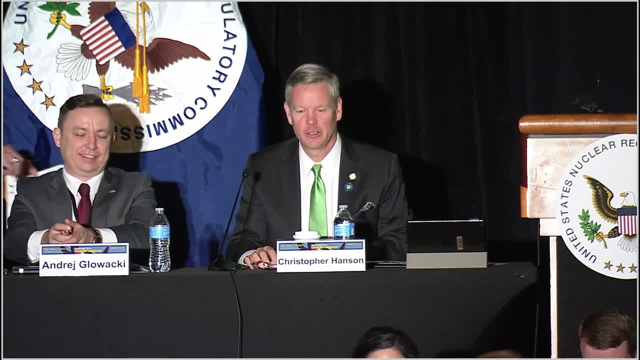 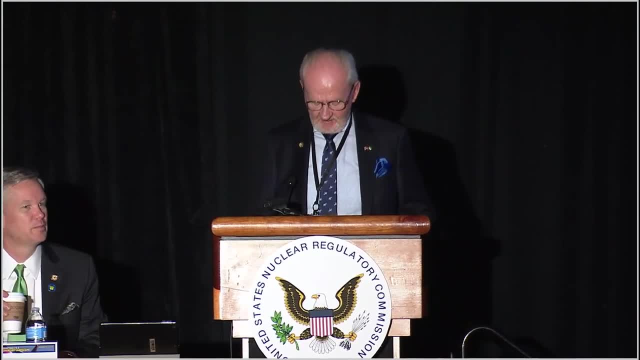 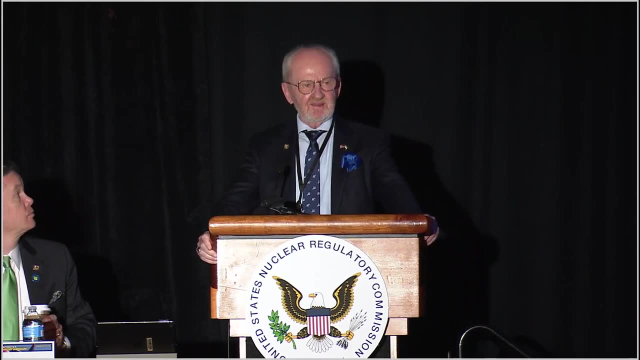 So please let me hand over the microphone now to my good friend, Krister Victorsen. So thank you. Thank you, Chris, and good morning to everyone. It's a pleasure to be here And to addressing this particular rick with. 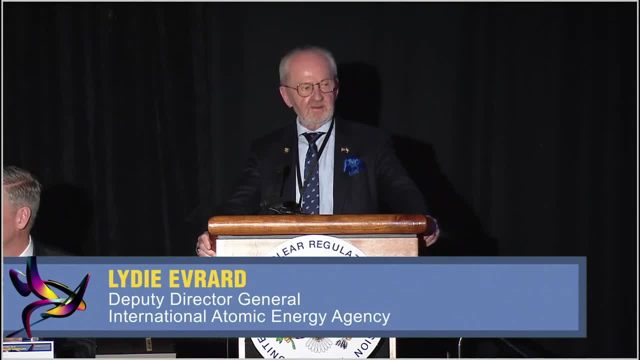 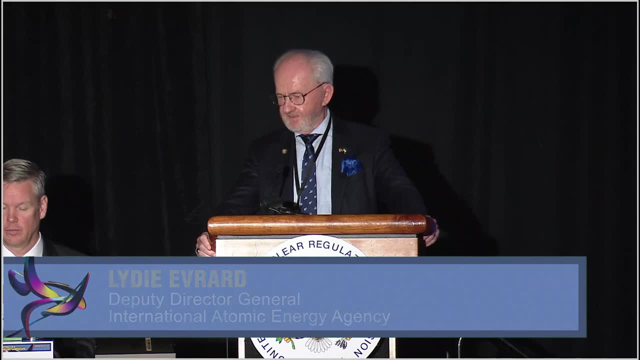 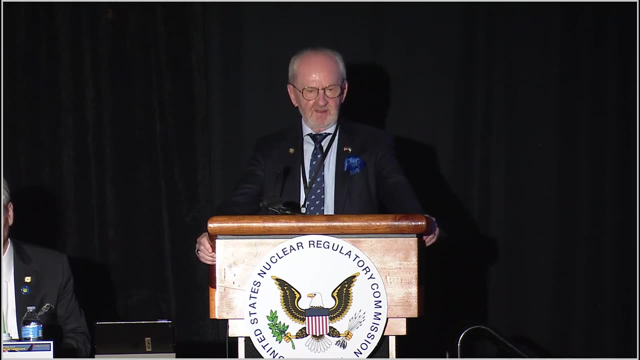 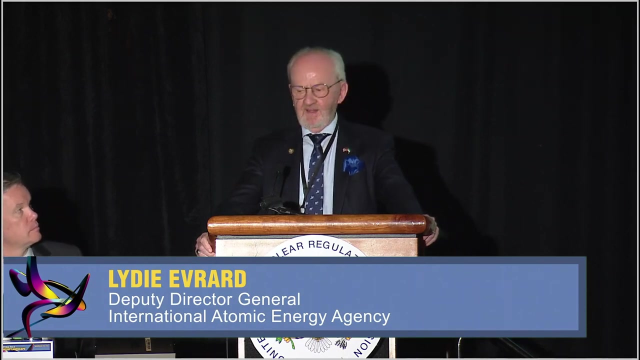 I think these are Liddy's slides. That's all right, But it's all right, We're going to, We're going to go, We're going to switch the slides. yeah, Addressing the changing landscapes in the world. So I have chosen to title my presentation to FANR, which is the Federal Authority for 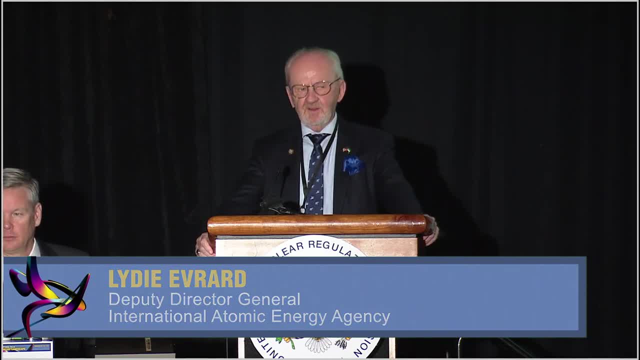 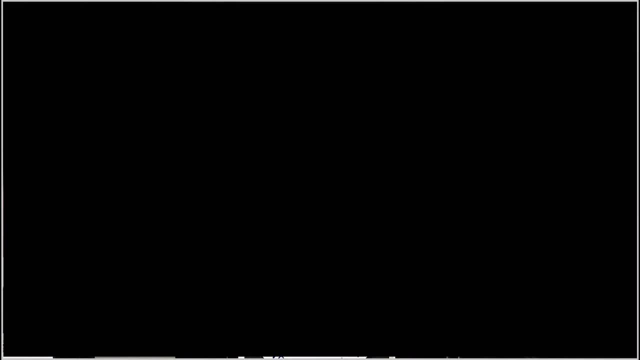 Nuclear Regulation in the UAE, which is the Nuclear Regulatory Authority, and, as my friend from Philippines mentioned, We were created in 2009.. And we do have a Or live in a very changing landscape. So let me quickly take you through some of the historical points that we have faced. 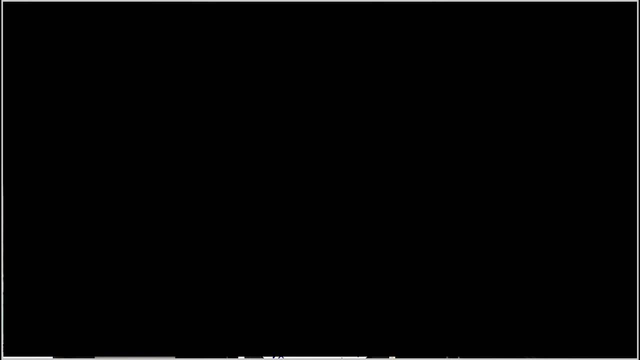 and the successes that we have made. If you could take the next slide, please. Yeah, Yes, he's coming. So this is a picture with the four nuclear power plants that now are in operation. So the first one went into operation in commercial operation in 21.. The second one in 22.. The third one in 23.. And the fourth one- We gave the operating license in November last year And they are now in the startup phase- went critical And in a few weeks I believe they will connect to the grid and then commercial operation. 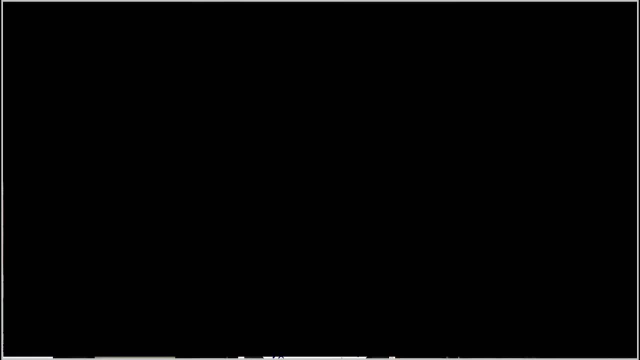 later this year. So this site, it was a beach, a beautiful beach, when I went there the first time in 2009.. And now it's completely different: A small city With a lot of infrastructure that is needed for a nuclear power plant. 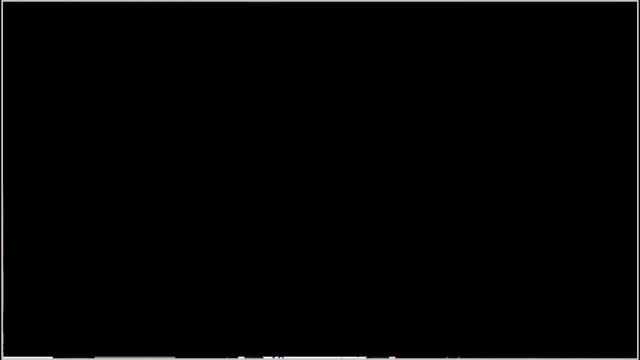 So it's a major project And the interesting thing is that Fanner and ENEC, which is the Emirates Nuclear Energy Corporation, that is the developer and it's an Abu Dhabi government entity. We are a federal entity. There is a difference between the two. 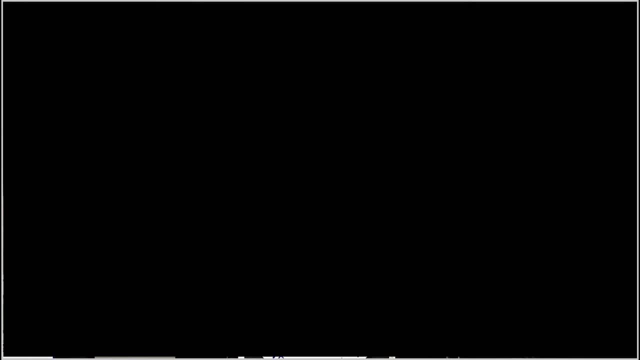 So we were established at the same time. In 2009,, we were sitting in the same building. Only a small wall was separated- me and Mohammed Hamadi, who is the CEO of ENEC. So this was, I think, the start of the creation of a good safety culture. 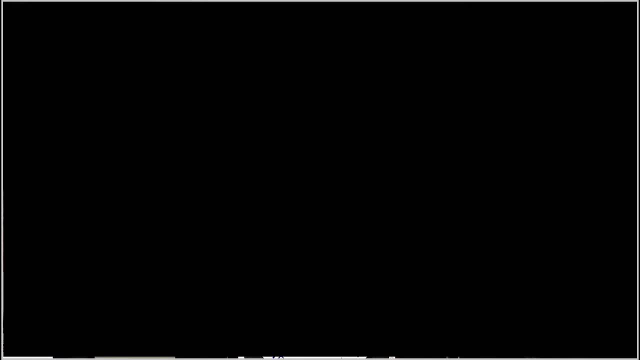 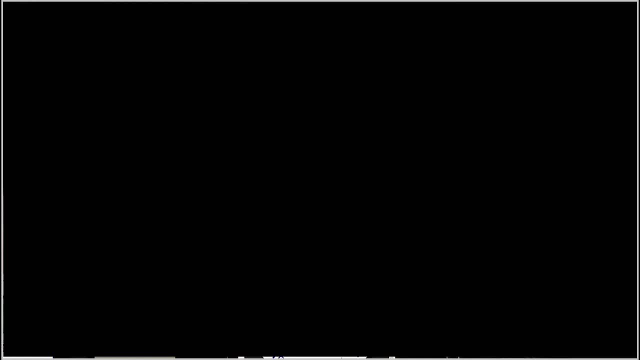 approach of the IEA. so it was sort of built during the same time as the milestone approach was created. So we had this- we worked on the same timeline both of us, so we knew when ENEC needed a. because there were no regulations in place, We had to start from scratch with the regulation. 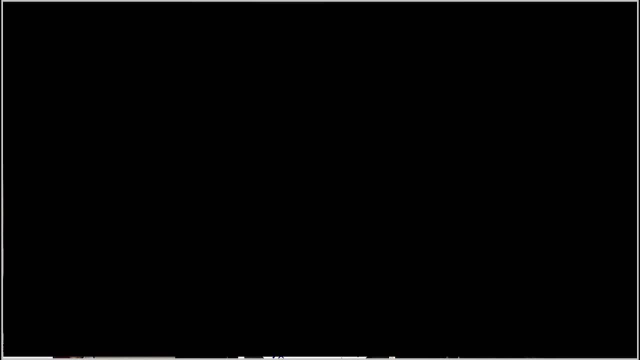 Anyway, it's a long story and there's many interesting topics to be covered, but the first license application we got in December 2010.. So between 2009 and December 2010, we worked on a sort of pre-licensing concept. We knew which reactor would be chosen, because the reactor was 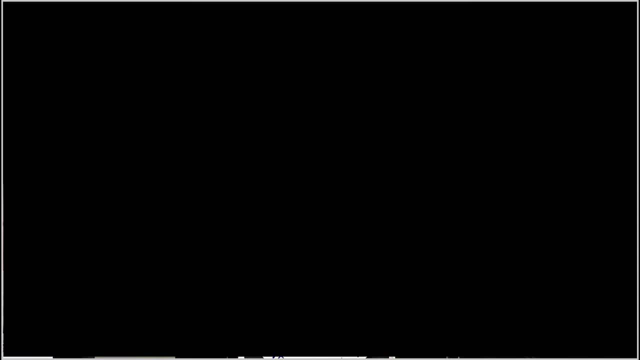 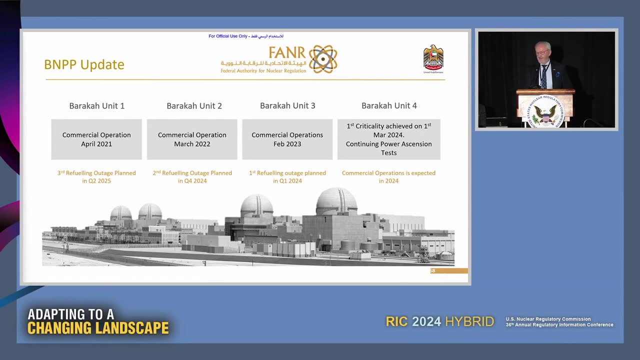 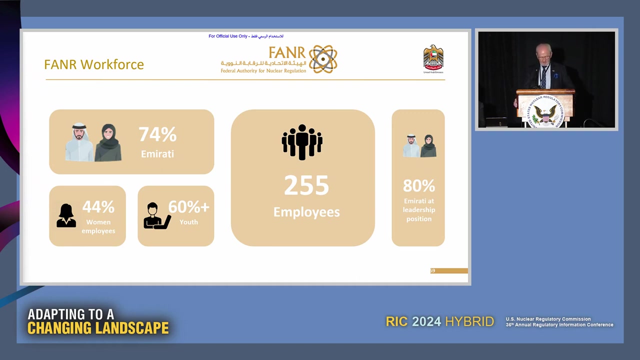 chosen. the contract was signed already in December 2009.. And today we have the full infrastructure covering all the 19 elements of the IEA milestone document. Next slide, please. So this is Fanner, some numbers. That shows where we are today. We are 255 staff. We have the responsibility, not only Baraka, we are 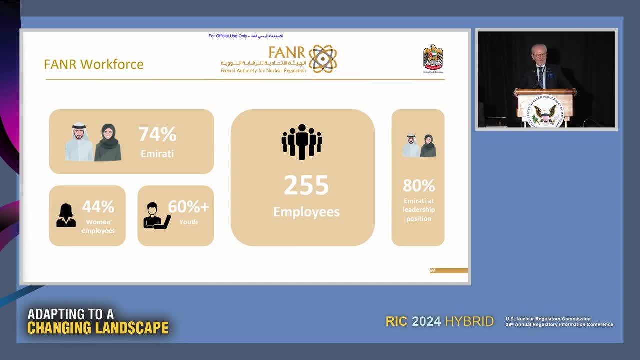 regulating all the medical and industrial use of radiation. We have security aspects, of course, and safeguards, So all these nuclear aspects we are in charge of. We started to be a completely foreign expert-driven organization. Today we are an Emirati-led organization And the number of Emiratis are 74. And two of them are: 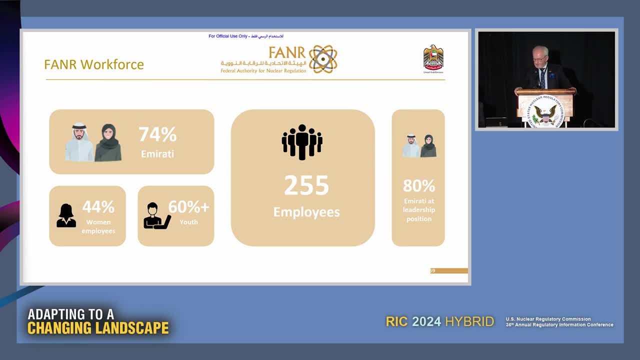 here with me. So this is the two you see in the same box that says 74.. They are with me. So Rashid- he's not dressed in white, a Kandura today- And Meera, the two of us here today for the space and nature. 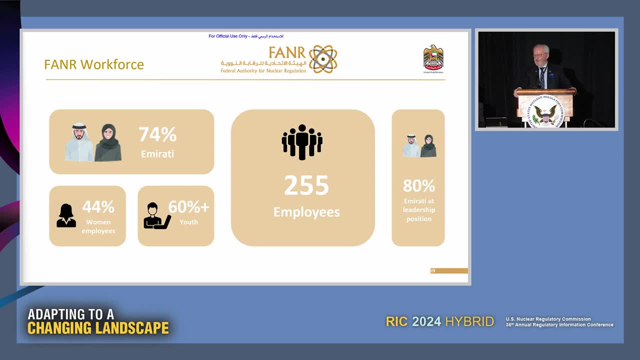 yu, who normally is in Black Abaya when they work. So they are with me and they have been with us about 10 years and they are today two of the many influencers I would say in FANR impacting the organization. 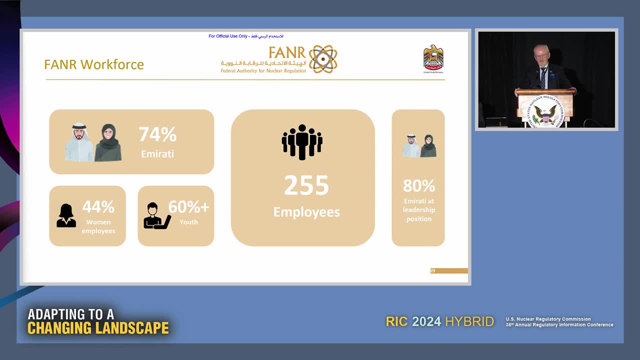 Mira is an inspector, has been a resident inspector in Baraka and Rashid is the manager of international cooperation. So I'm very proud of you. So we have had a very successful emiratization program. so I'm very confident that the nationals in the UAE. 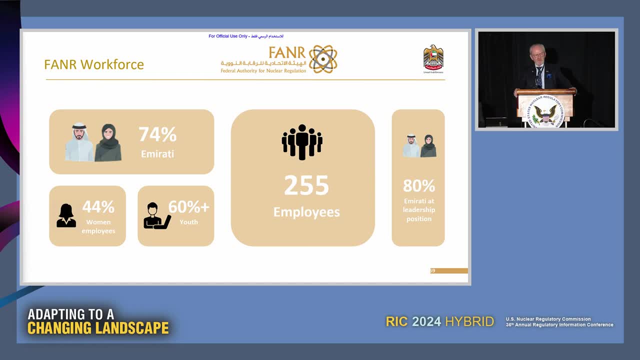 will shoulder the responsibility for safety, security and safeguards in an excellent way. We have a lot of females. We have 44%. We have a lot of women. We have a lot of women, We have a lot of females and this has come naturally. 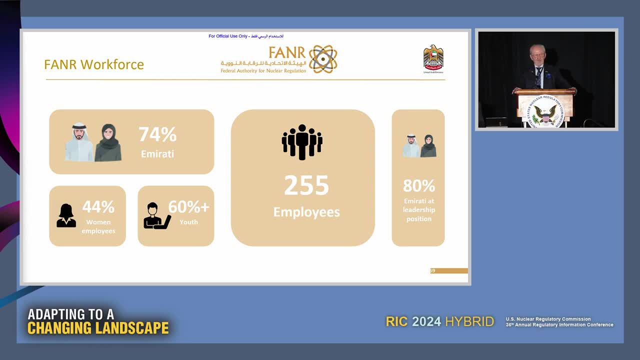 because in the UAE, the majority of the STEM students are females, So it has been a natural evolution. We have a very young population We are. 60% are below 35.. The youth is defined as between 18 and 35.. 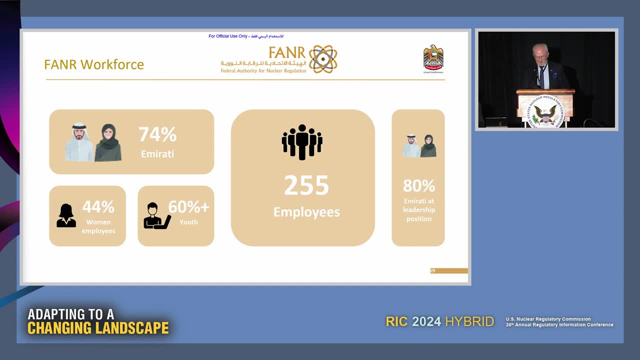 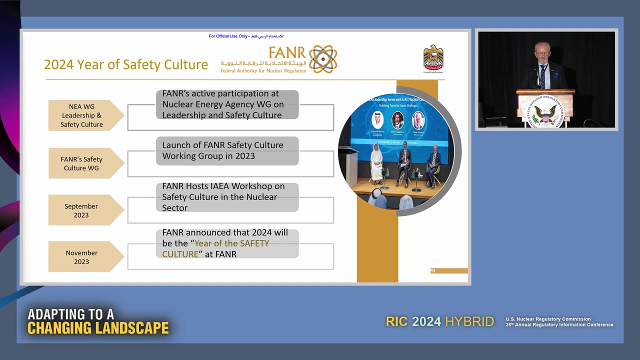 We have many leadership positions, 80% are. that's why I said emirate-led organization, Next slide, please. So we do have now all the reactors in operation, So we have switched from licensing into operational oversight And then, of course, as you all realize, safety culture. 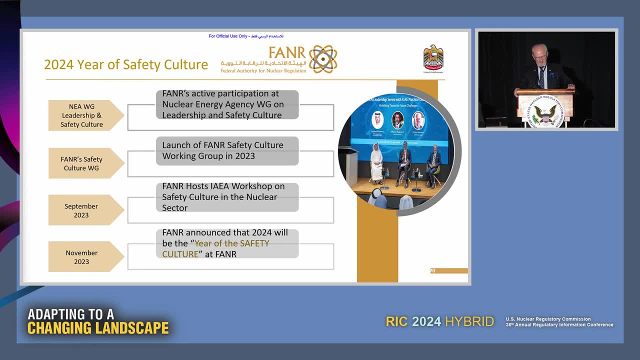 it's an important aspect of the operation. So we have been active internationally. You heard yesterday in one of the sessions about the NEA working group on leadership and safety culture. We have been there. We have created an internal safety culture working group. 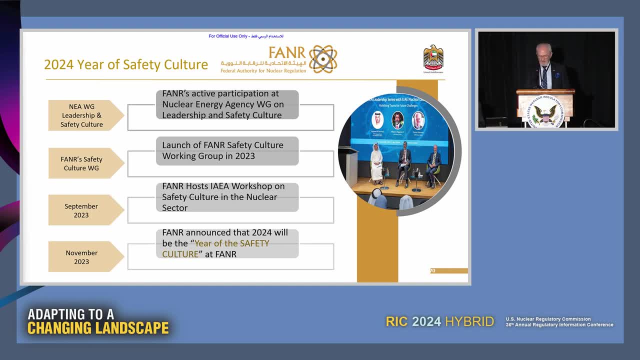 We had an IEA mission in September. We have been there to teach us about how to do a self-assessment of the internal safety culture, which we will do next year probably, And I announced in November last year that 2024 will be a year. 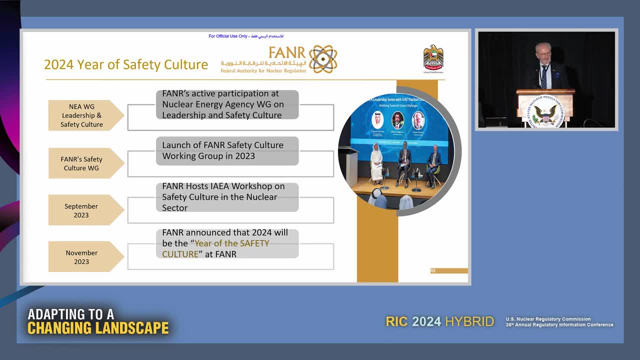 of safety culture at Fanner which will influence our own program and our own inspectors particularly focus on the inspectors. The resident inspectors have do have an important influence. They have an important influence on the safety culture of the operator in particular. 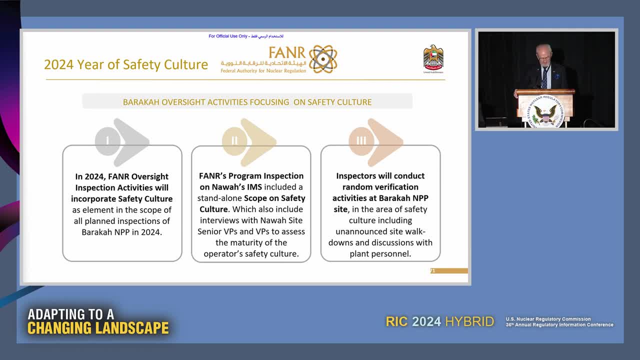 Next slide, please. I will be quick. So we will also focus our oversight activities on safety culture. not only, of course, but we will include an element of safety culture in most of the inspections that we are doing. Next one, please. 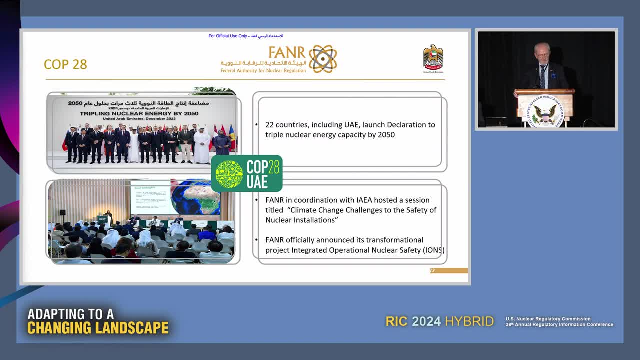 So another change. Next one is the COP-28.. So on the 2nd of December last year in Dubai, 22 heads of states came physically to Dubai to sign the tripling declaration of nuclear energy by 2050 in the perspective of the climate change. 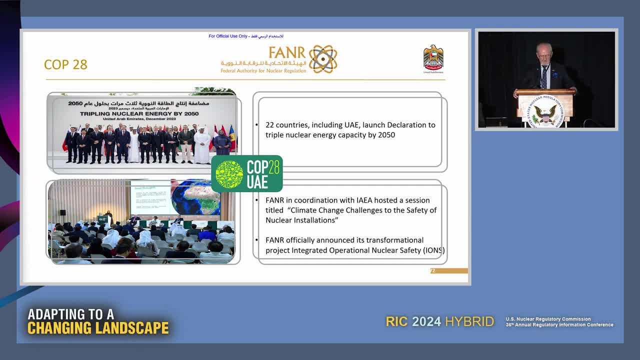 On this opportunity, we also had a workshop with the IEA. Next slide, please. So on the 2nd of December last year we also had a workshop with the IEA, with WMO and with the presence of EDF on the resilience. 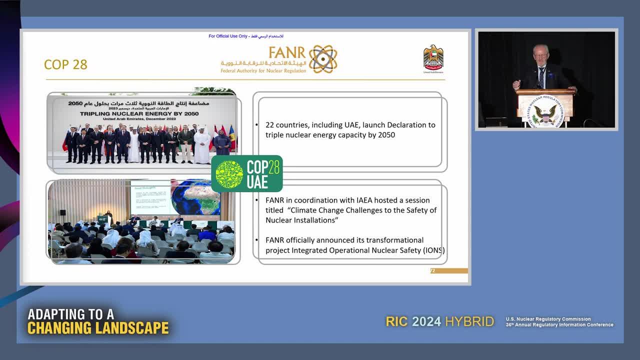 of nuclear power plants for challenges caused by climate change. So we have officially launched and working now on a transformational project which we call integrated operation and nuclear safety. I can talk more about it later. Next slide please. Next slide please. 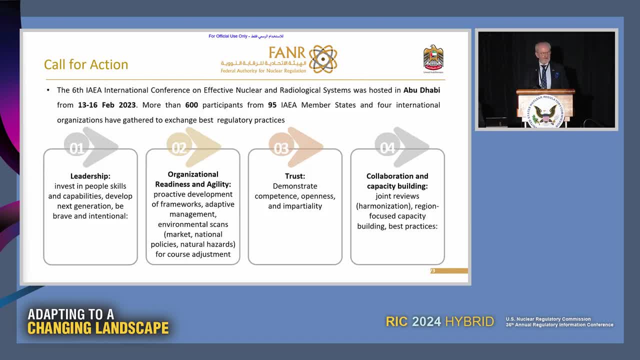 We had another important event that I would like to point to, namely the regulatory conference, And the regulatory conference agreed on four themes, and these themes are not only for Fanner, it's for all regulators. So we worked together with NRC chairman Chris to make sure that we have a follow-up and make sure 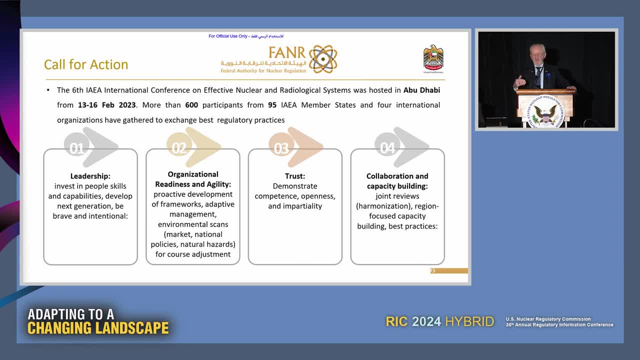 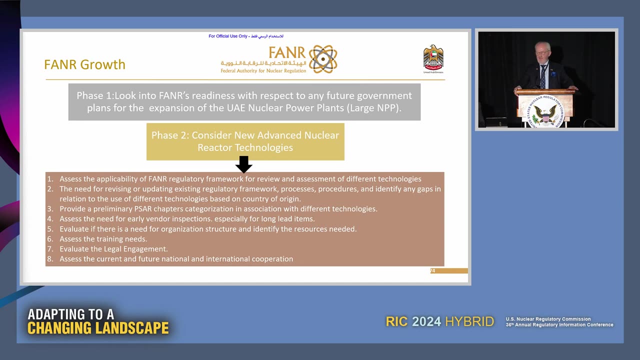 that regulators really commit and take actions in these four areas, and we are certainly doing it inside Fanner. Next one, please. So, based on this COP28 signal, we realized that more nuclear will come. We don't know. no decision has been made in the UAE, but we expect. 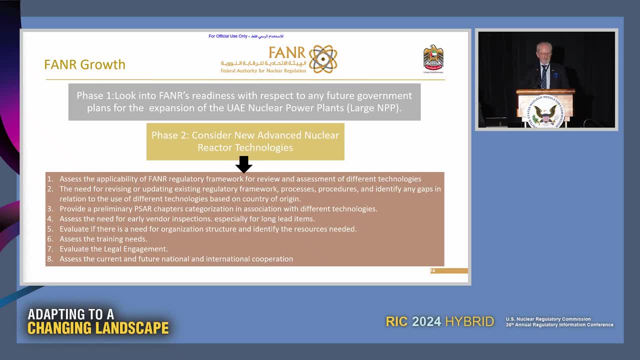 and, as we have heard during this conference, we expect that more nuclear will come. we need to be ready as regulators, so we have created a task force- we call it fanner growth- to study the consequences of of additional big reactors and SMRs. and this is just some information about the. and the last land slide is next one. 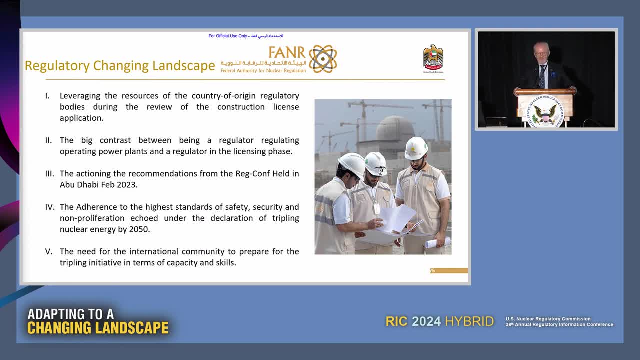 talking about the, the changing regulatory landscape so many of us have- many of my colleagues have mentioned, is leveraging the resources and we certainly did that when we when we started licensing of baraka. these are Korean APR 1400 reactors. there was a reference plant in Korea, built and 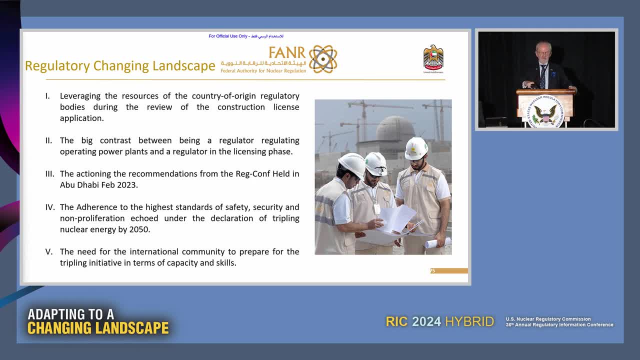 operated licensed. the reactor was licensed by nrc before system 80 plus of combustion and engineering, it was licensed by Kinz. So we said in Fanner, why should we redo everything? There is no reason. We trust what NRC did and we trust what Kinz did. 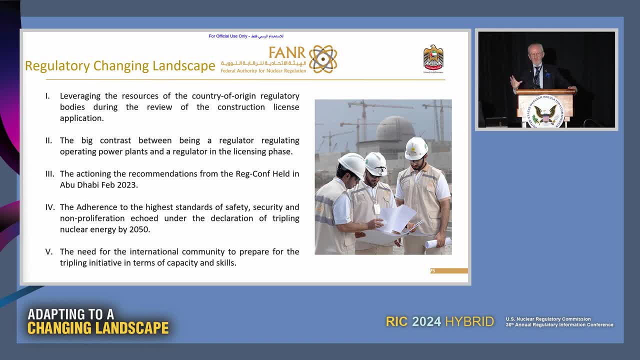 Of course, we reviewed exactly what they did, So this allowed us to focus on specific UAE factors like the weather, environment, et cetera, and on the organizational setup on the topics that we were responsible ourselves. So also, and the second message is that there is 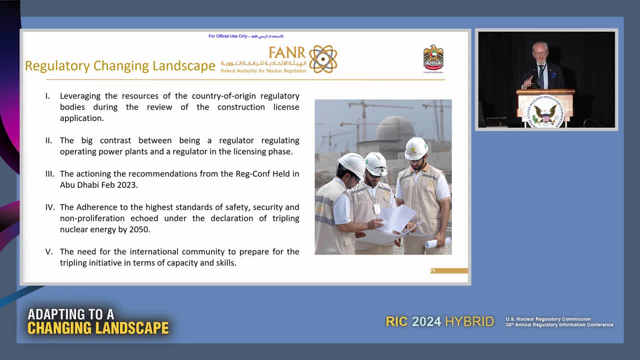 a big contrast between being a regulator with operational oversight and licensing. This is: you have in operational oversight. you need to be ready. You have to have the full oversight or full infrastructure And you need to be ready to act 24-7.. 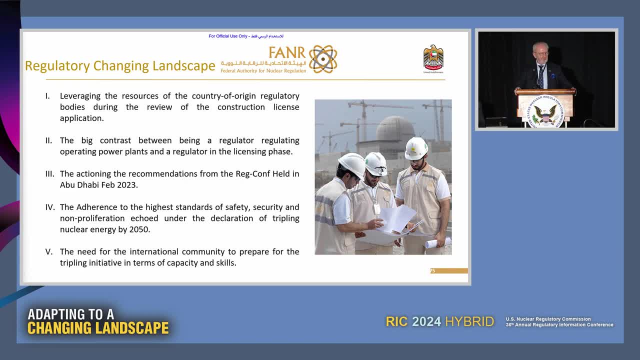 And we have experienced that at Fanner Many weekends. we have worked- and this is a must- And we are adhering to the recommendations from the REG conference and we make sure that we have the highest standard for safety, security and safeguards under this tripling. 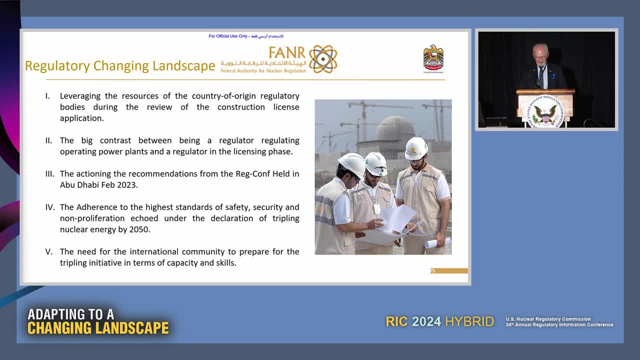 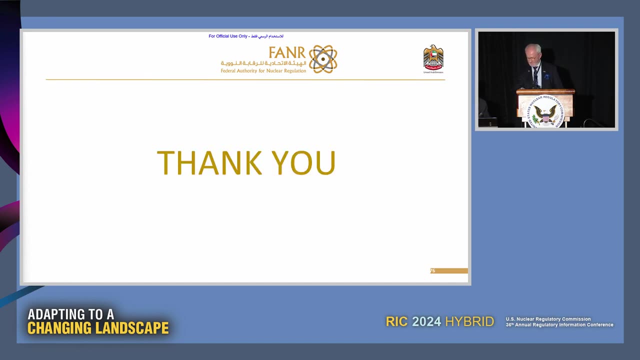 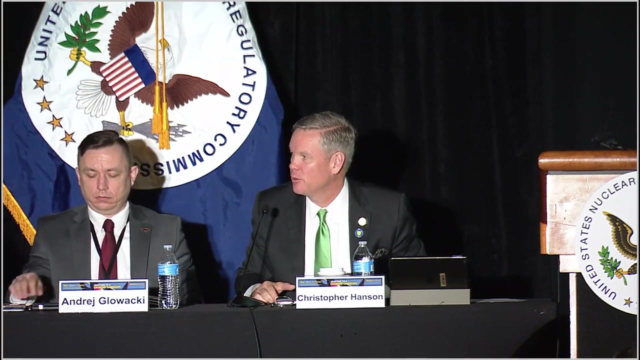 And this needs some additional, also international cooperation. So I would really urge the international regulatory community to work together in order to challenge or to face all the challenges of the tripling initiative. Thank you very much. Thank you very much, Director General Victorsen. 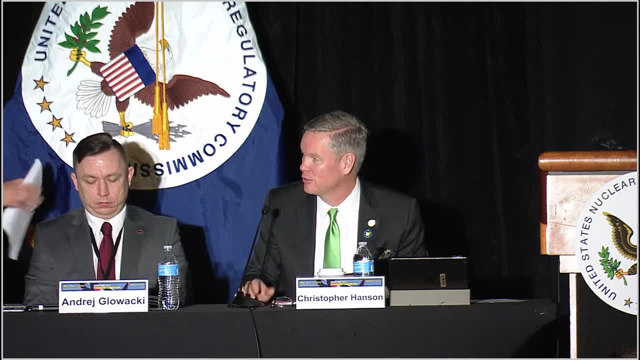 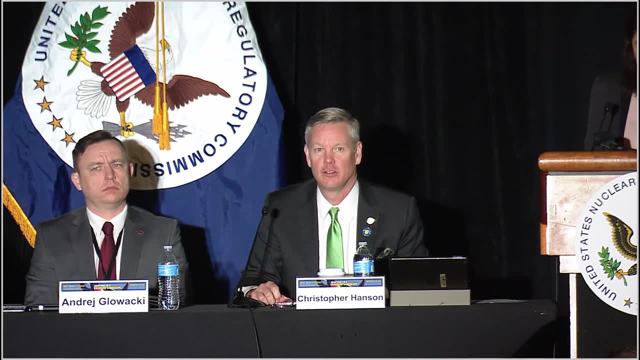 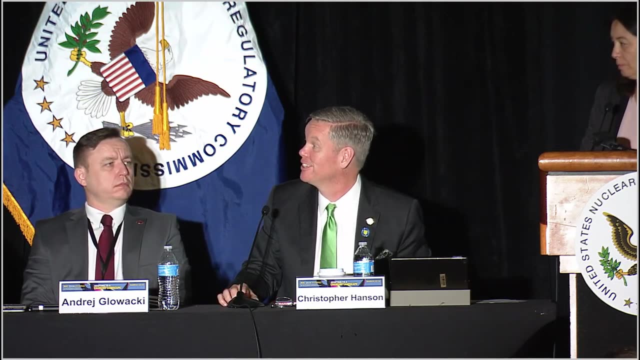 for your presentation And I would note that there are even, I think, some really leading edge things going on in the UAE with regard to regulation, For instance, your dedicated cybersecurity incident response center, and I believe there's a director for innovation. 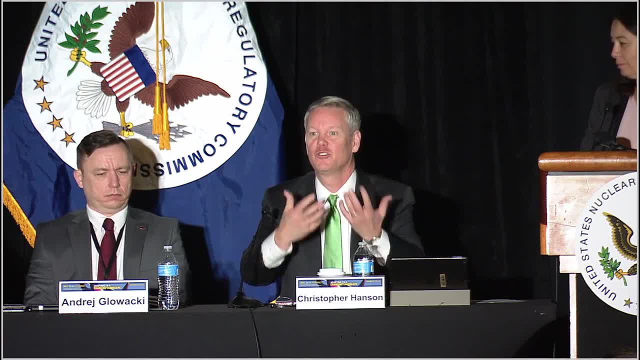 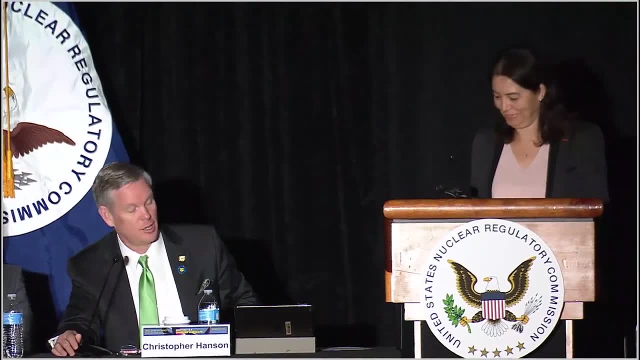 in your organization now that, even as you're building this capability, you're also leaning forward and looking at changes as well. So thank you very much, And next I'd like to hand over the microphone to Deputy Director General Liddy Everard. 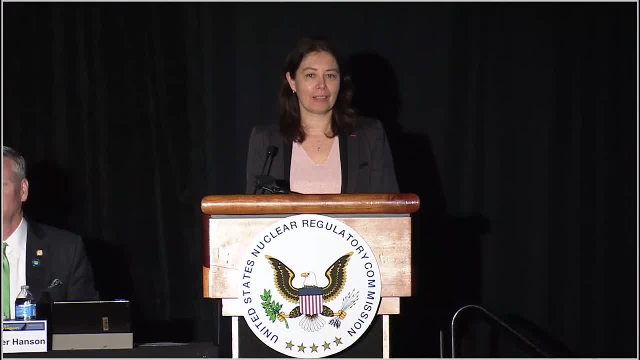 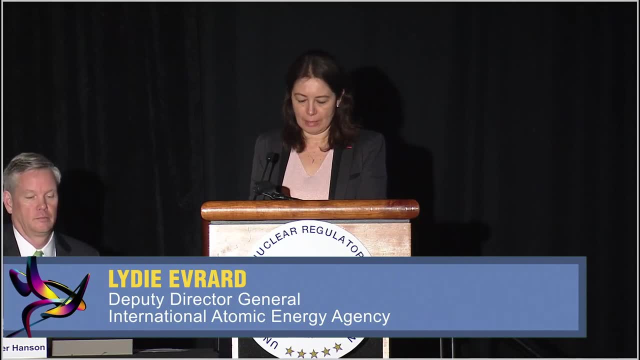 Thank you. Thank you very much, Chris. Good morning, ladies and gentlemen. Good morning, Good morning. It's my great pleasure to address you today at the RIC And I will give you an overview of the AAE activities to support regulatory infrastructure and SMR safety. 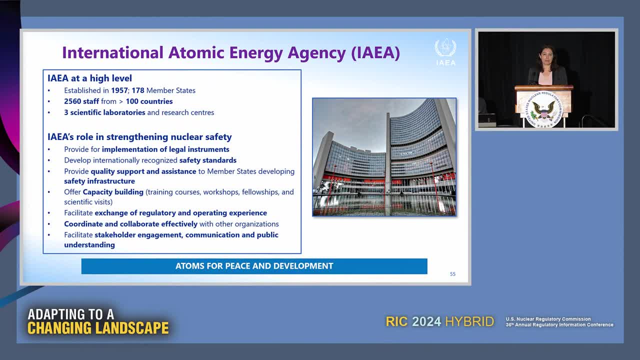 First, the AAEE, established in 1957, has 178 member states and works under the motto Atoms for Peace and Development. The mission of the Department of Nuclear Safety and Security is to provide a strong and sustainable global nuclear safety and security. 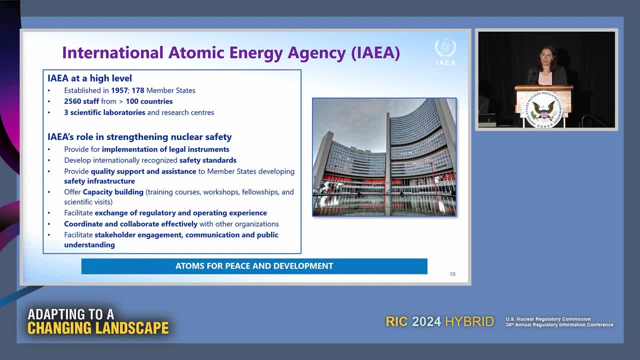 frameworks, with the development of safety standards, the provision of peer reviews for their application and the implementation of legal instruments such as the Convention on Nuclear Safety. The agency is highly committed to building national capabilities in nuclear safety, especially for embarking countries. 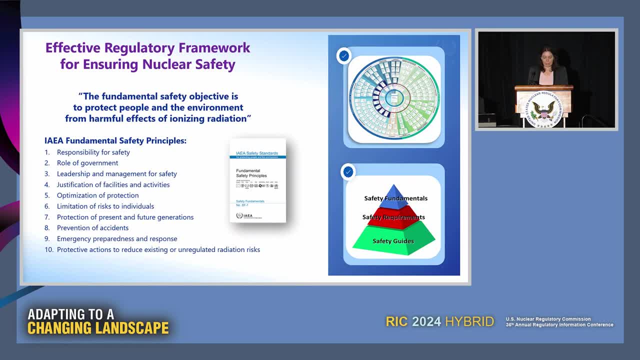 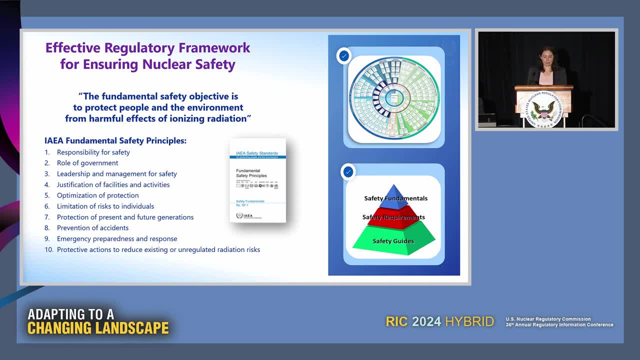 worldwide. To date, 134 safety standards have been published and 136 are under development. There are three levels of safety standards, safety fundamentals, with one safety objective, which is on the slide, and that states that this fundamental safety objective is to protect people and the environment. 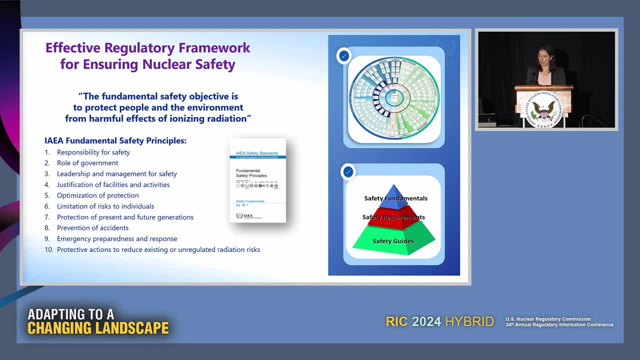 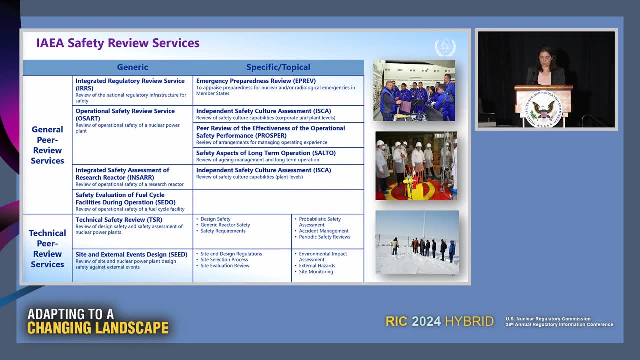 from harmful effects of ionizing radiation. And then there are other levels, so safety requirements and safety guides. The AAEE supports its member states via safety review services in which member states' practices are compared with these international safety standards. In 2023, the agency conducted a review of the safety standards. 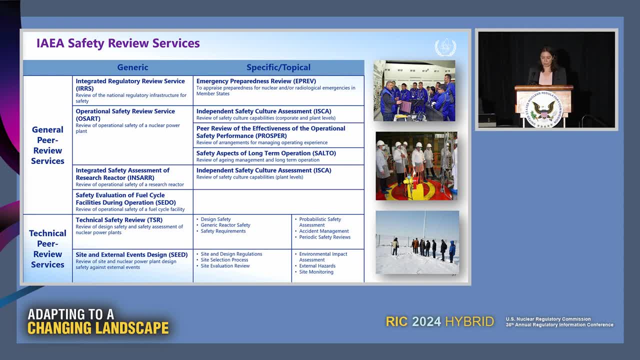 The agency conducted over 60 safety-related peer reviews and advisory missions and, as you can see, there are many different reviews, for instance, on regulatory infrastructure, such as ARES, missions on operational safety, other missions on long-term operational safety. 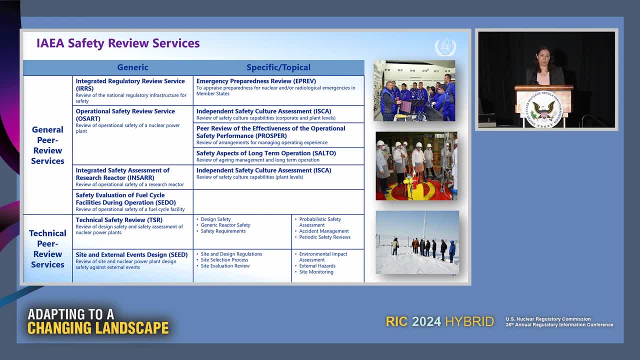 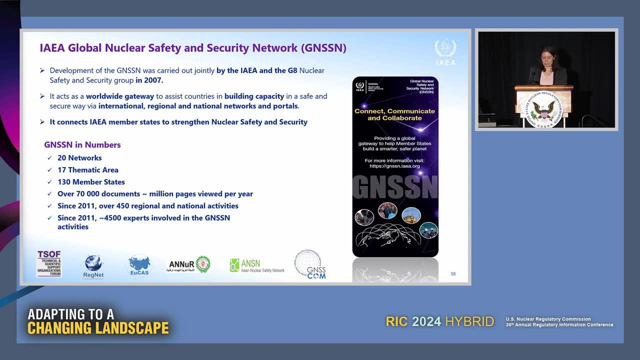 so SALTO, but also on topical matters such as safety of research reactor or safety of fuel cycle facilities. The Global Nuclear Safety and Security Network, so the GNSSN, is a web platform whose missions comprise three elements: First, sharing knowledge, experience and lessons learned, supporting interactions and 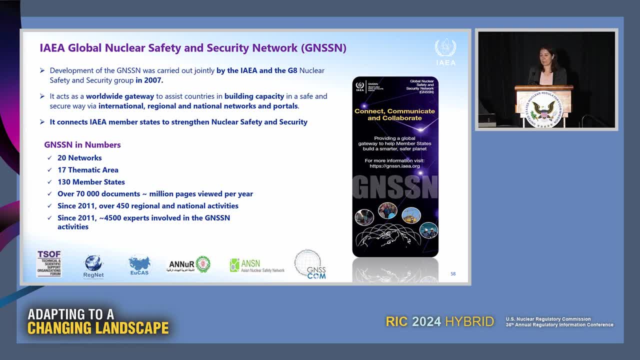 collaboration amongst member states and supporting capacity building. The GNSSN includes 20 networks in total. That includes the Global Nuclear Safety and Security Network, the GNSSN, and the Global Nuclear Safety and Security Network, which includes regional and topical networks. 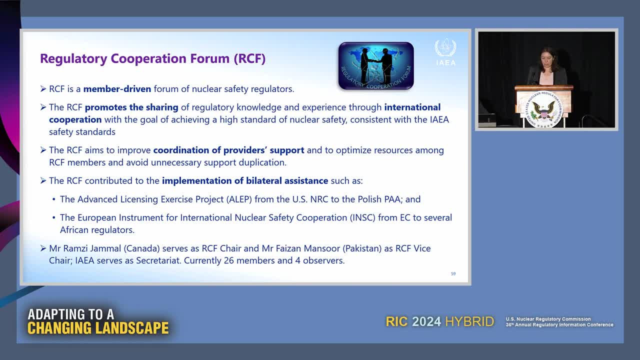 The Regulatory Cooperation Forum, so RCF, facilitates collaboration between member states with established nuclear power programs and member states embarking or expanding on such programs. The RCF has contributed to multiple instances of bilateral assistance, including engagement between the US and Poland and activities of the European Commission in Africa. 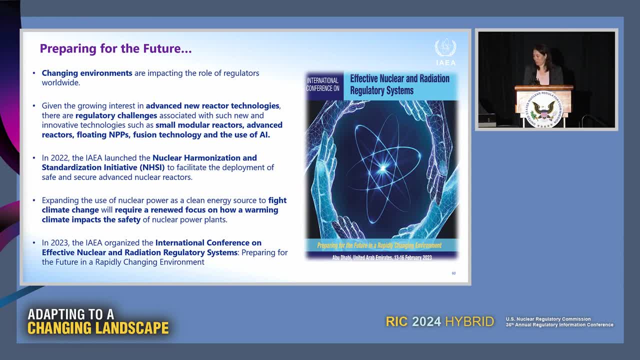 So this slide is, you know, directly linked to the topic of the RIG. so that's interesting to have this kind of connection. That means that it's really, you know, a major topic for all of us. So how are we preparing for the future? 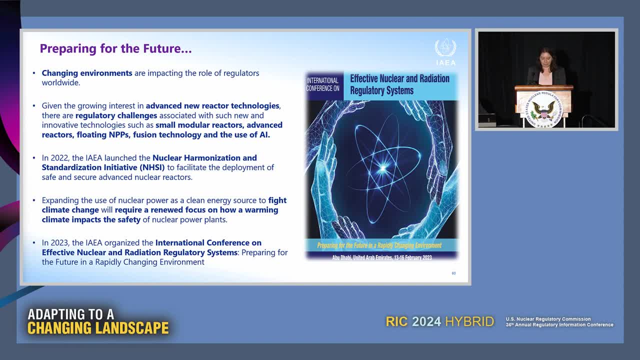 In 2023, we had this regulatory conference, which is on the slide, And, as you already mentioned. so the environment we are working in is always evolving, which impacts the role of regulators. The past few years have brought several examples: the global pandemic, of course, emerging new. 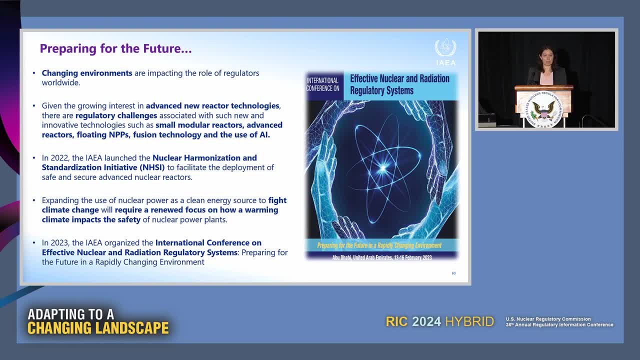 technologies or ensuring nuclear safety and security during armed conflicts. So this is a few examples that illustrate what we need to address- And usually in a kind of unpredictable conditions, In 2023,. with this international conference in Abu Dhabi, regulators shared their experience. 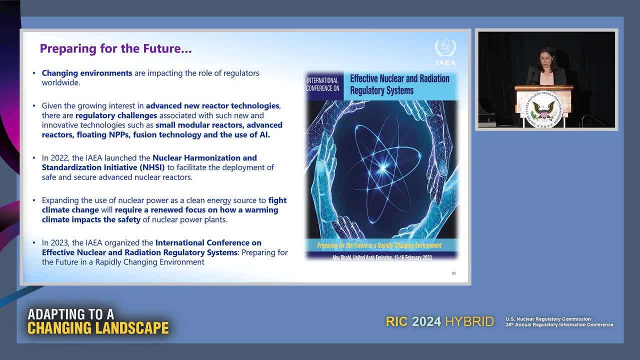 particularly with regard to building resilience and agility to respond to new challenges. Thank you very much again to you, Chair Hansen, and to Christa Victor-Sum for serving as president and vice president. Thank you to the United Nations, Thank you. Thank you to the Arab Emirates for hosting this conference, which was a very successful. 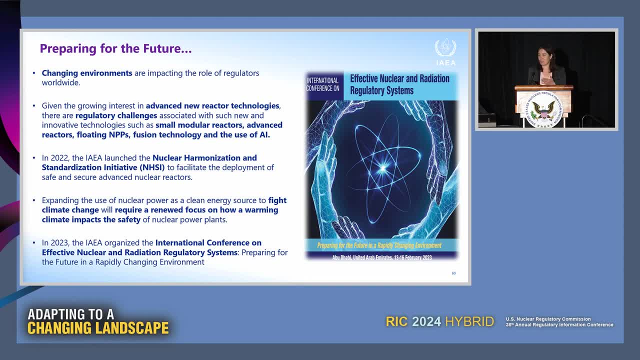 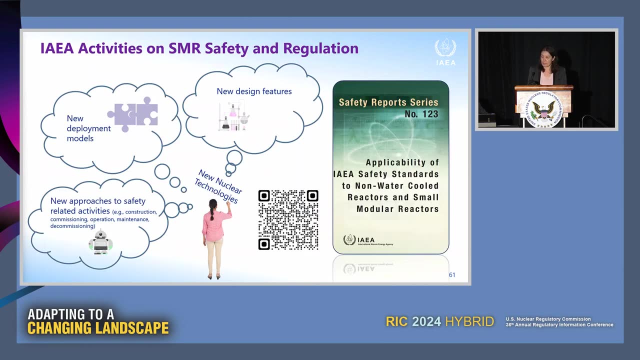 conference with more than 600 participants And this very clear call for action. This is the next step. I think a conference is an important step, but the follow-up actions are equally, you know, important. Now moving on to the agency activities and SMRs. 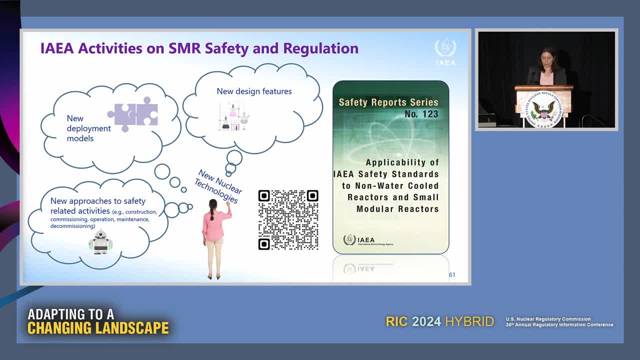 In 2022, the agency completed an extensive review of the applicability of the safety related matters to SMRs, and this review of applicability is guiding us for preparing our plan for the future on how to address safety-related matters for SMRs. 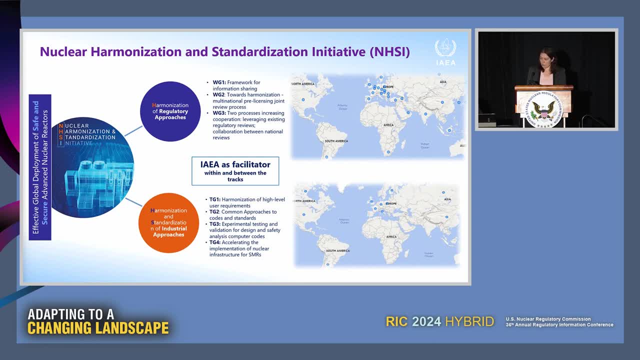 In 2022, the director general of the IAEA launched a new initiative called the NECI- that stands for Nuclear Harmonization and Standardization Initiative- with the objective to achieve progress towards harmonization of regulatory approaches and standardization of designs, and thereby facilitating the safe and secure deployment of SMRs. 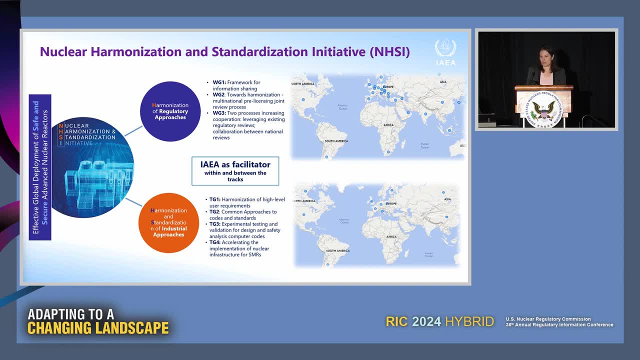 NECI has two tracks: one on industrial matters and another one on regulatory matters. Regarding the regulatory track, there are three working groups dealing with how to share information. Second, how to develop a multinational pre-licensing joint review program. Third, how to develop best practices for regulators to work together on ongoing regulatory 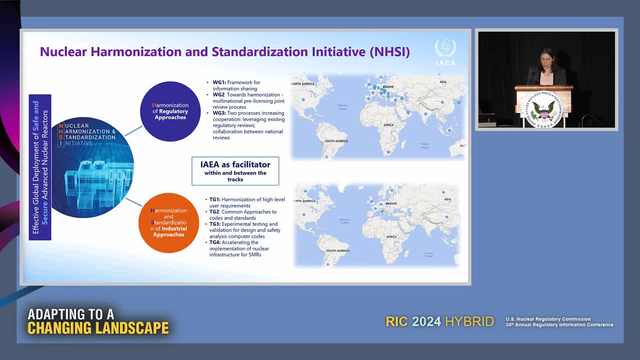 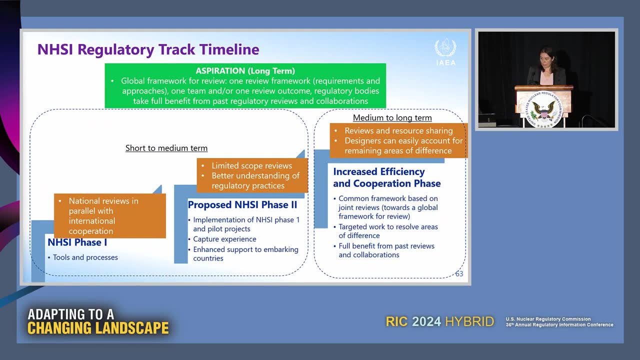 reviews. As you can see from the map, there is a broad participation from several member states throughout the world. Regarding NECI timeline, we are currently finalizing the first phase of NECI and we are preparing for the next steps to be discussed at the plenary meeting of NECI. 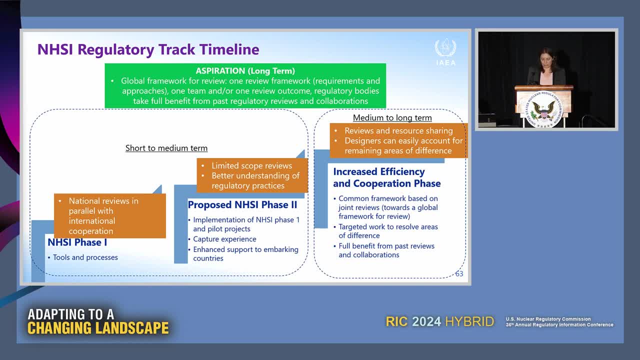 Our long-term aspiration is to develop a common review framework, and this is really our main objective. We plan to continue to enhance processes for regulators to leverage and learn from past reviews, thereby saving resources while still maintaining a high level of safety and allowing regulators to maintain their sovereignty in decision making. 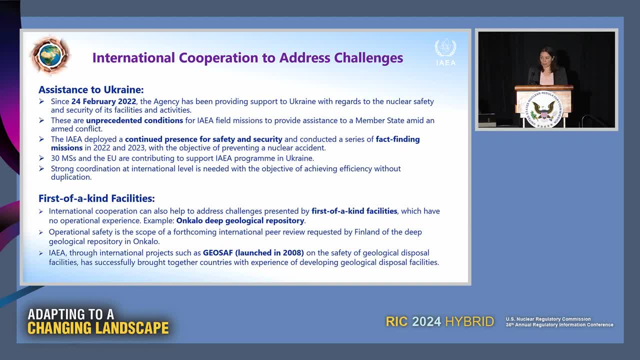 Thank you. International cooperation also provides a foundation for addressing global challenges, including in unprecedented conditions. I would like to give two examples. First, on the assistance to Ukraine: Since February 2022, the agency has been providing support to Ukraine with regard to the safety. 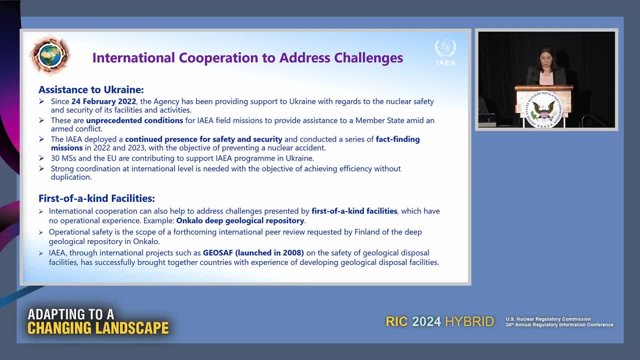 and security of its facilities and with the main objective of preventing a nuclear accident in Ukraine. In particular, we have deployed continuous presence of the agency in Ukraine. We have delivered equipment, safety and security-related equipment to Ukraine thanks to a strong support from multiple states, and I would like to thank very much the US, who is one of the. 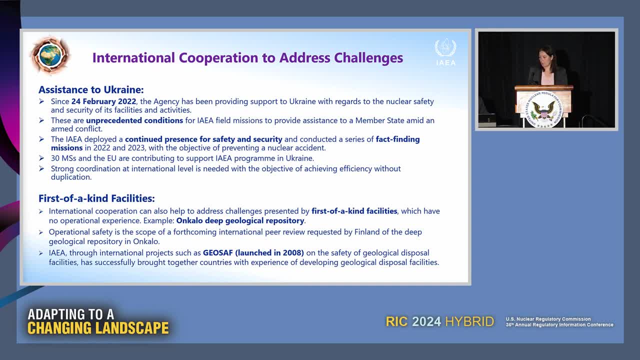 major supporters for this comprehensive program of assistance for Ukraine. We also develop- and this is the second, completely different comprehensive program for the US and India. The US has gotten very engaged with Ukraine and its international partners and the sister. 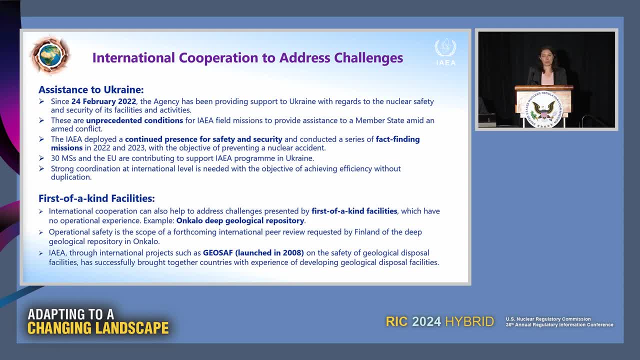 different, of course, examples. We developed some support and assistance- ad hoc support to member states with first-of-a-kind facilities. For instance, we are working with Finland for the deep geological repository and we are working on a peer review to address operational safety of such a facility. 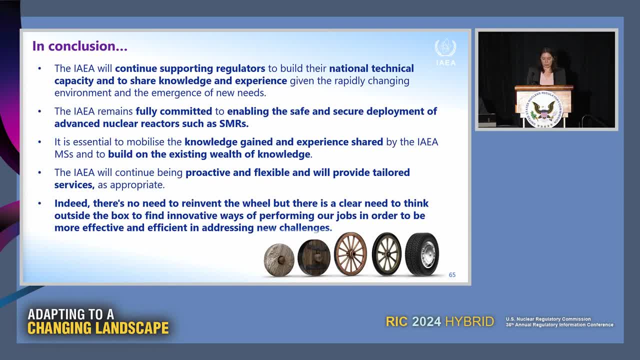 In conclusion, the agency will continue to support member states for knowledge and experience sharing, to build on the existing wealth of knowledge, to remain proactive and flexible in responding to the diversity of member states' needs and to contribute to strengthening safety and security worldwide in this rapidly changing. 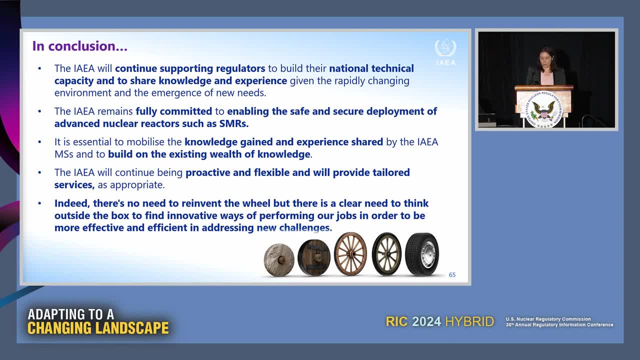 environment. I agree that there is no need to reinvent the wheel- This is a topic of this session- but there is a clear need to think outside the box, to find innovative ways of performing our mission in order to be more effective and more. 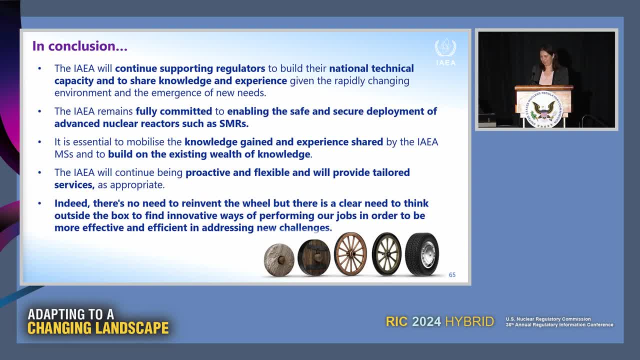 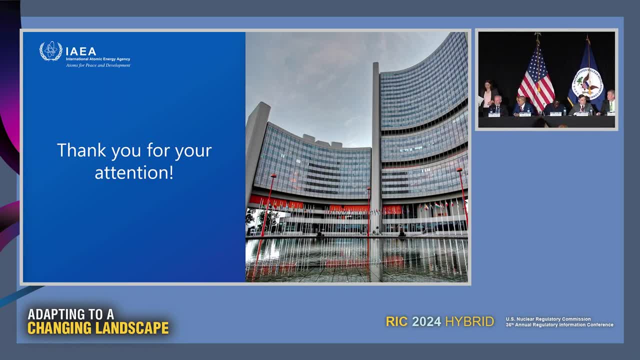 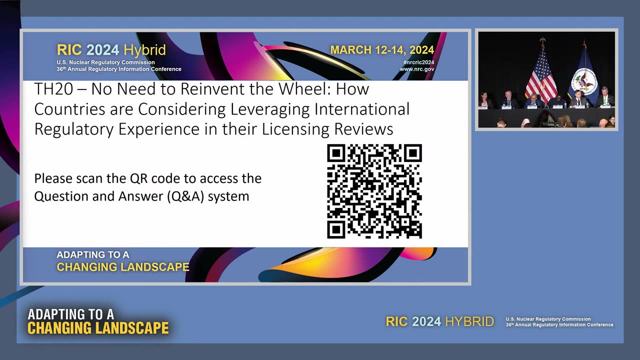 efficient in addressing new challenges. Thank you very much. Thank you, Liddy, for that, and particularly that last bullet in the closing sentiment. I couldn't agree more obviously. Well, let's get into some questions here and have a bit. 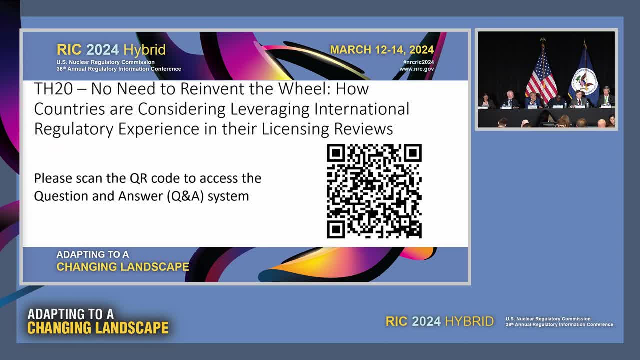 of a discussion I'd like to start off with- I think this is a question for Poland and our friends from Ghana and the Philippines- really about how is your country planning to leverage licensing reviews and data from vendor countries in your review process? 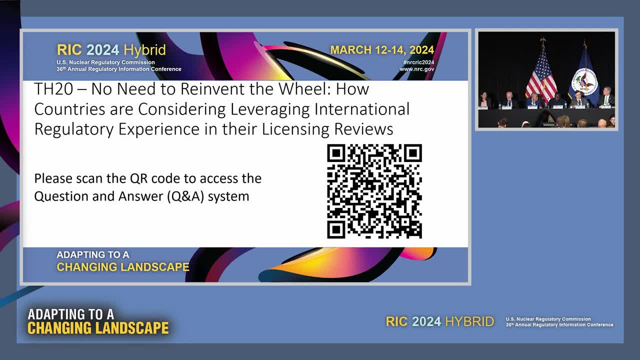 I think this could be a question as well for Fanner, in order to talk about pre-existing reviews on the APR 1400 and other thinking about how, if new technologies are going to be deployed in the UAE as well, and what do you think are the 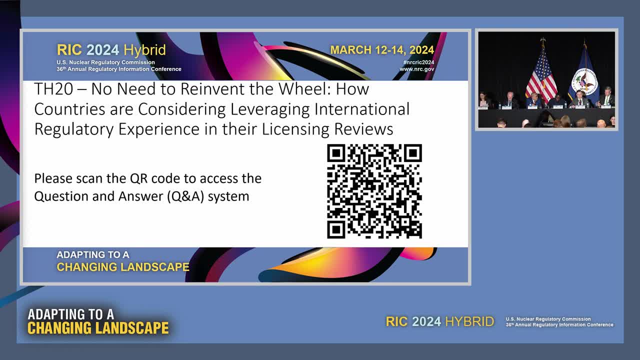 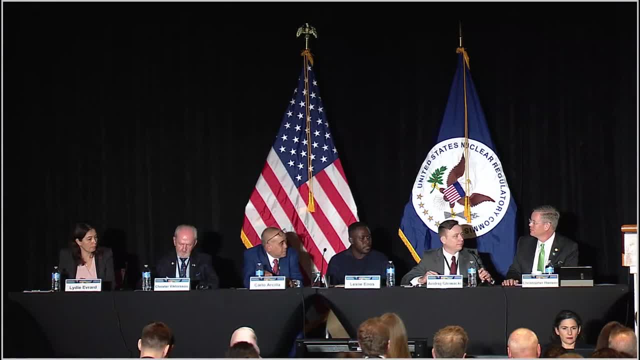 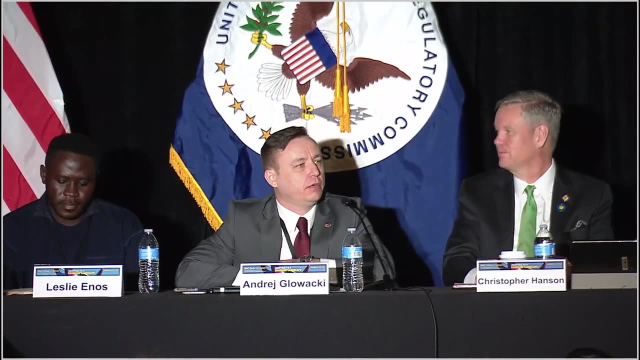 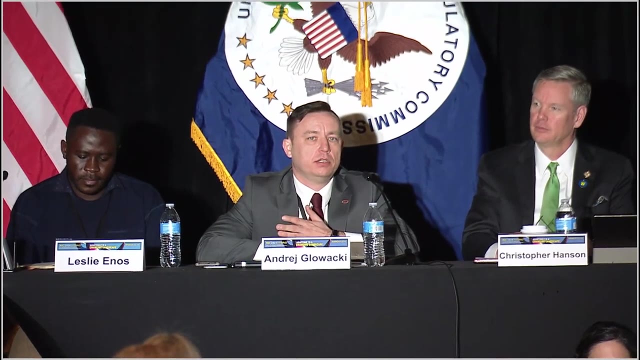 greatest challenges to accepting information from another country in your national review process. You can go first. Thank you very much, Chair. Well, thank you for this question. Actually, we are currently working on this, since the AP1000 was the first NPP which is going to build in Poland and it already has been. 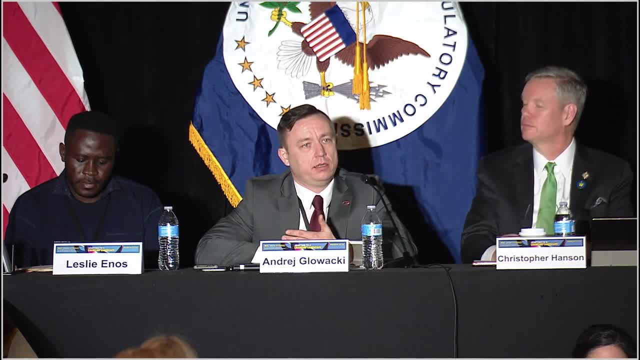 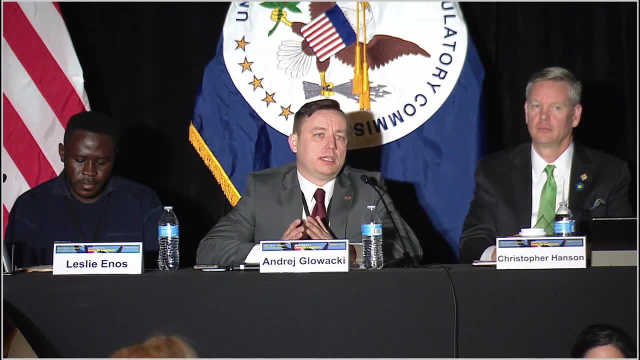 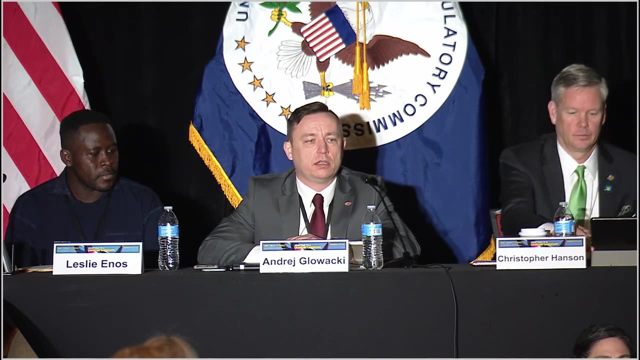 licensed in the US. It has already been built, constructed and is in the operation. So our approach is that we don't want to also, like Fanner, don't want to review all the technical information from the beginning. We 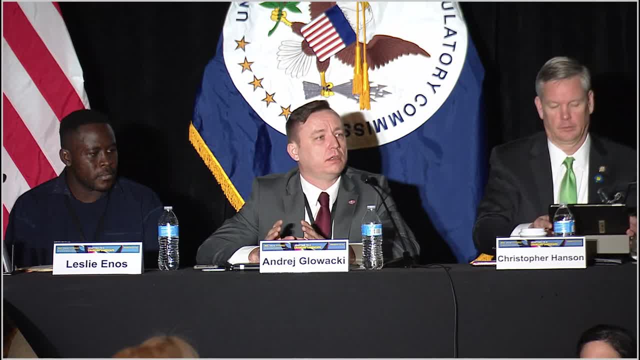 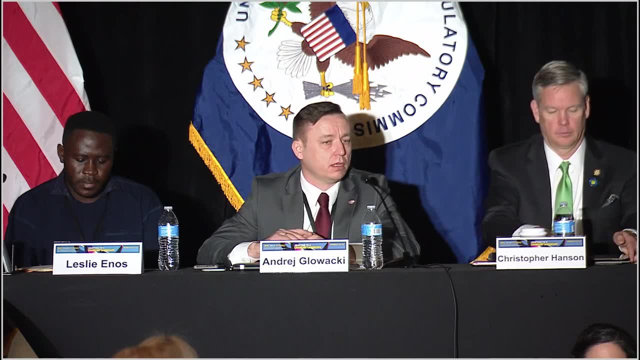 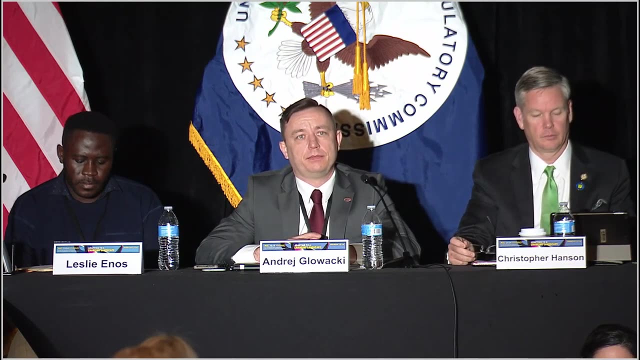 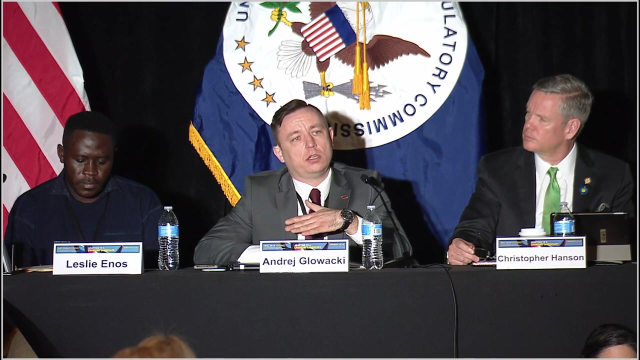 wanted to take the benefit of the work and the assessment which has been done in the US and and to take some of those to our review. There are some legal challenges, of course, to what extent we can use this kind of information, but for sure the 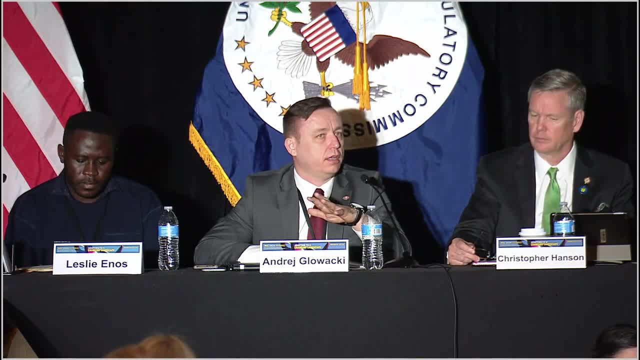 aspects, which are quite general. we're going to take them into our review and our assessment. We're going to focus on the site specifics. We're going to focus on the environmental specific issues. There are some differences in requirements and this is what I wanted to. 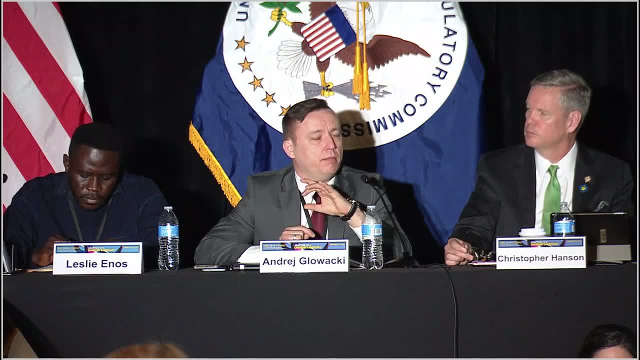 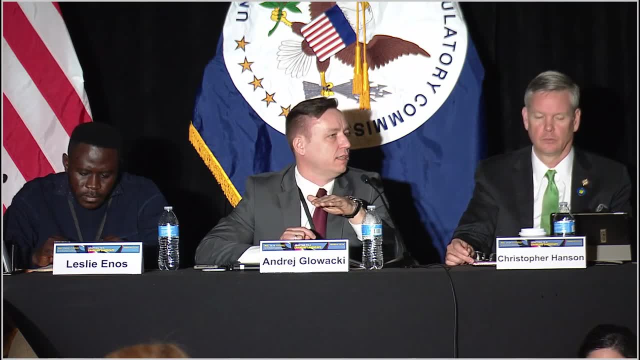 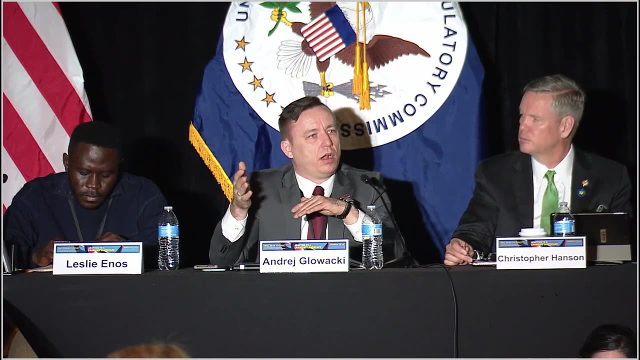 emphasize. So the biggest challenge is make sure that you understand what was the design basis, what was the legal basis in the country of origin versus what is in your country, against what kind of requirements the design was verified. So we started to fix those that are missing. 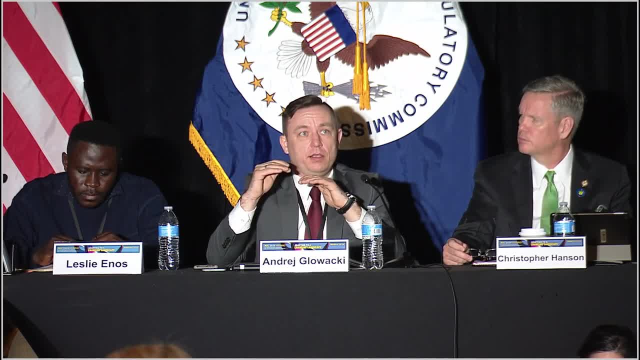 – the ones, those there are not. If we can check people, hopefully they'll be more informed about what were the requirements, and this will only try to hint and help us in order to закi t check. In other said that they confirm that it's a. 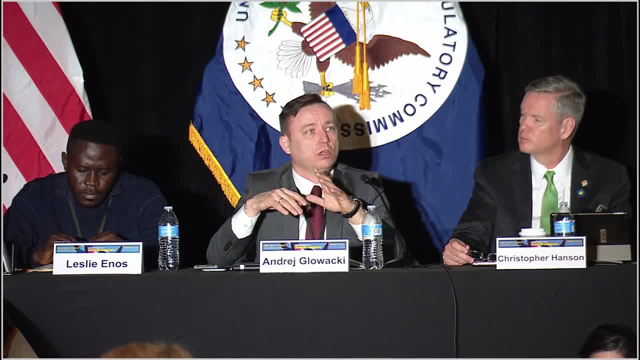 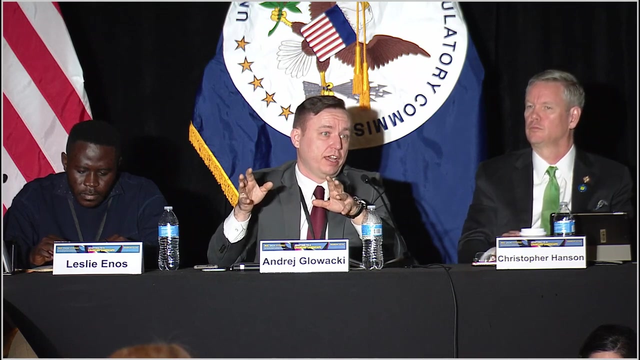 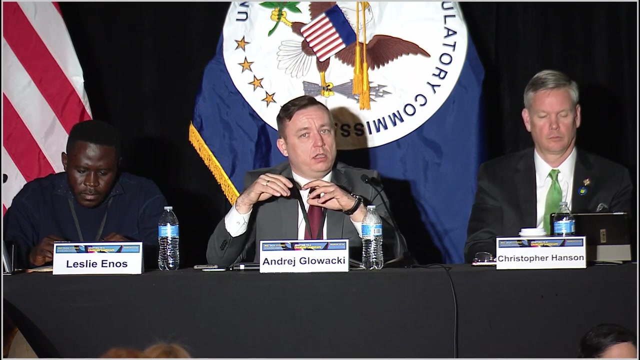 really good example of how the types of along fringe of New York were, and those were the some of the basic requirements for making sure that they could work. doing this, So we are verifying and using the time which we have right now to compare also the requirements in US and in Poland to be knowledgeable enough that we can assure. 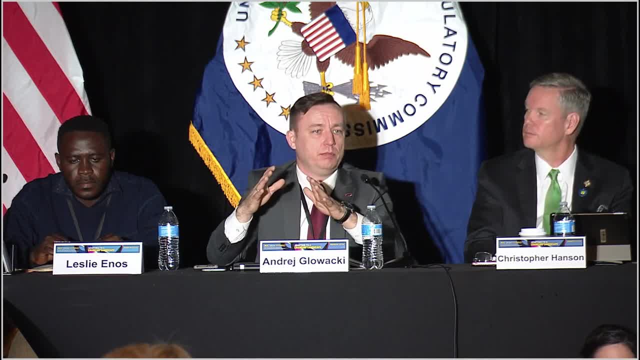 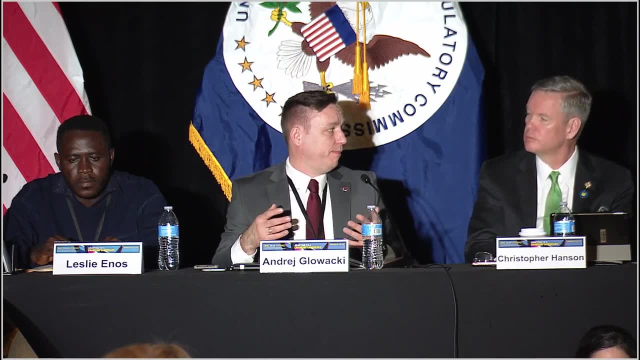 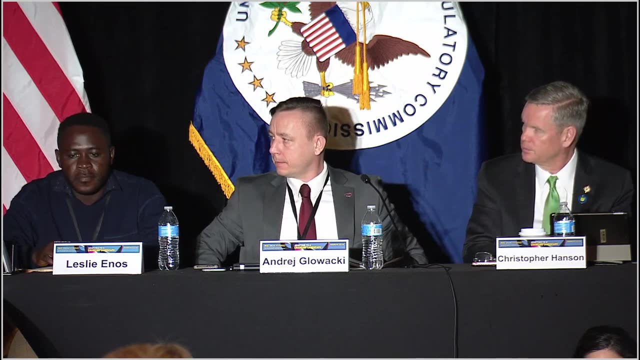 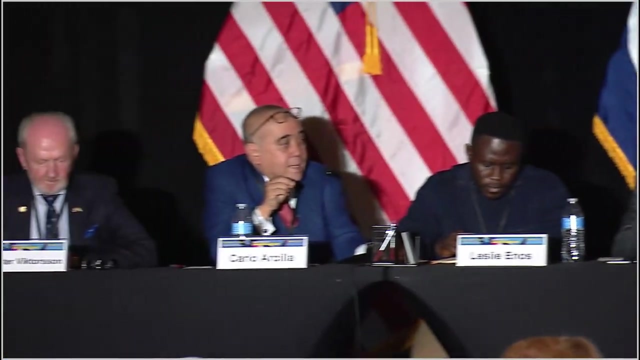 then, when we will get the application, we will be knowing which kind of documents reviews we are able to accept. So I'm going to leave with that and give the floor to the next. Regarding the question, in our current law that will be approved soon, there's a provision that if a technology has been licensed in another country, 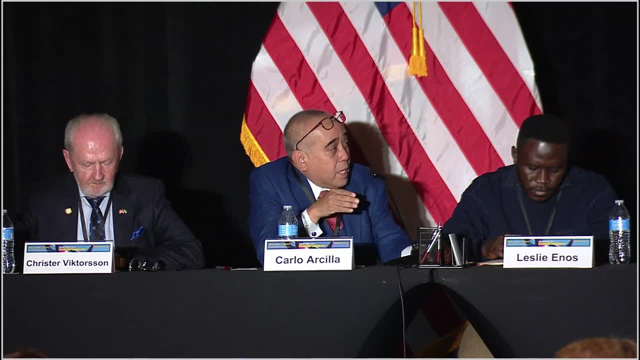 with a credible background that we can consider that. so to shorten the licensing, And I think this is especially important for SMRs. The Philippines is interested in SMRs because we have 7,000 islands and the most expensive power are those not connected to the grid. 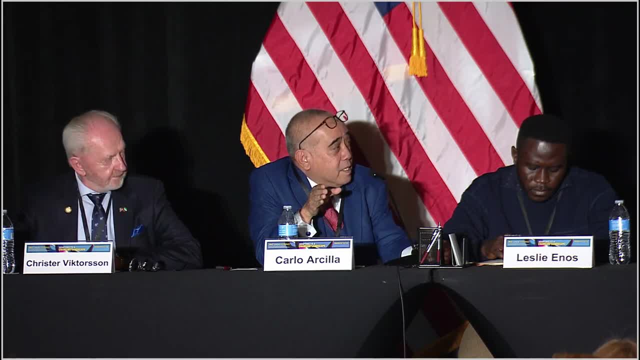 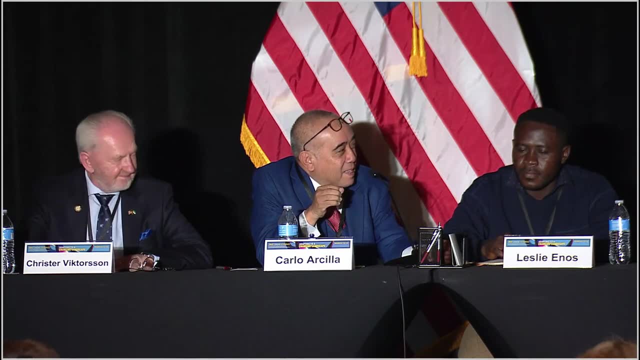 But the problem with the SMRs is that there are 100 designs. They're mostly PowerPoints. We need power plants, So we need that something is operating, because it's the only way that you can check. Anybody can sell anything. 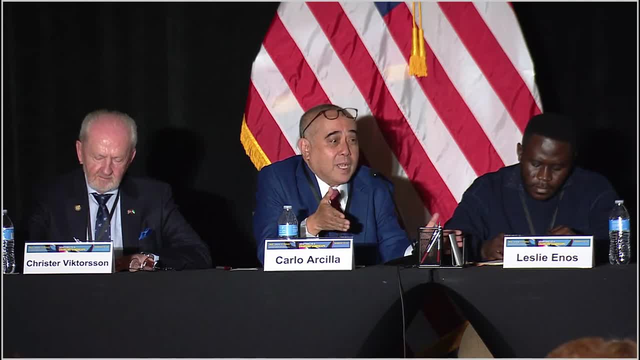 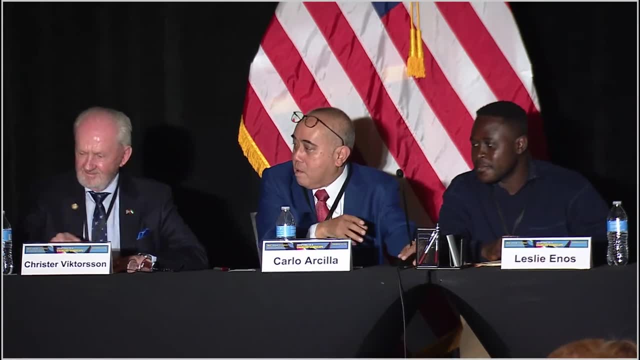 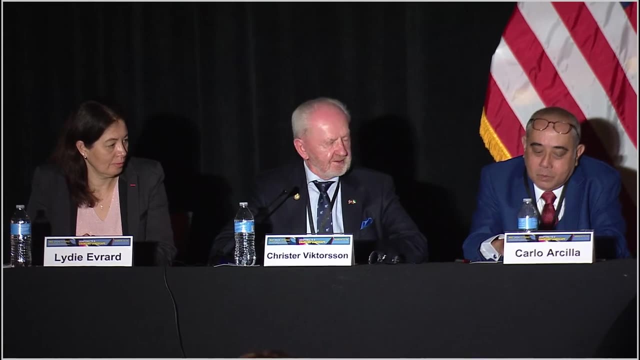 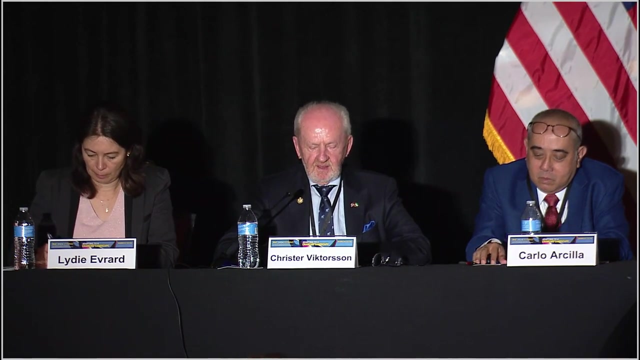 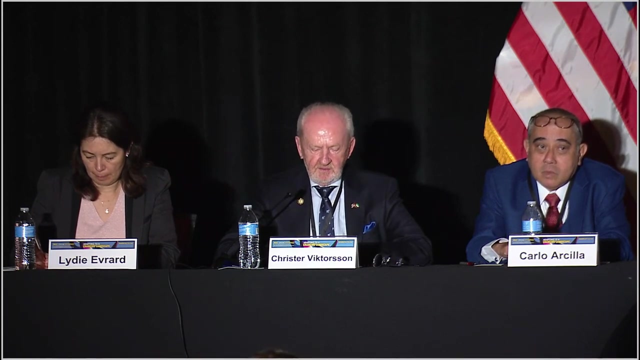 So there's no first of a kind. I mean, you guys won't buy a first of a kind car. What more for a nuclear power plant? Thank you, Yes, a few comments from Fanner. So first on the new technology. Yes, we have to prepare, to be ready to review a new technology, whether it's a light water reactor or a small modular reactor or other types of new technology. 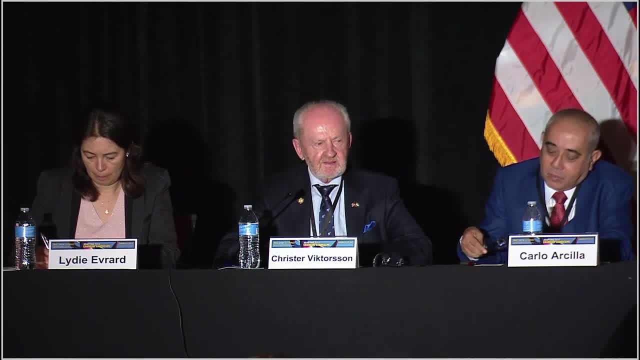 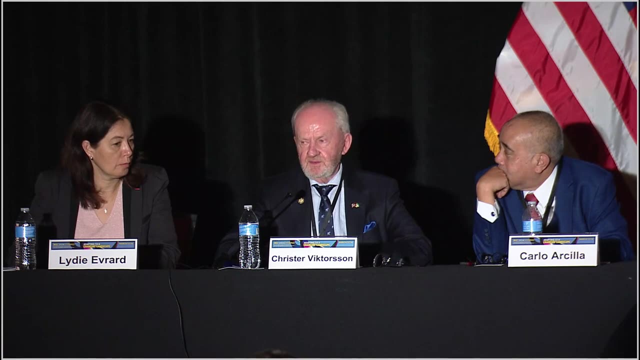 And on the question of there are 80 or 90 different designs, that's true, But you can also, if you work with the industry, you can screen- Thank you- All these design- I mean we have done it and we are down to five or six which could be of interest. 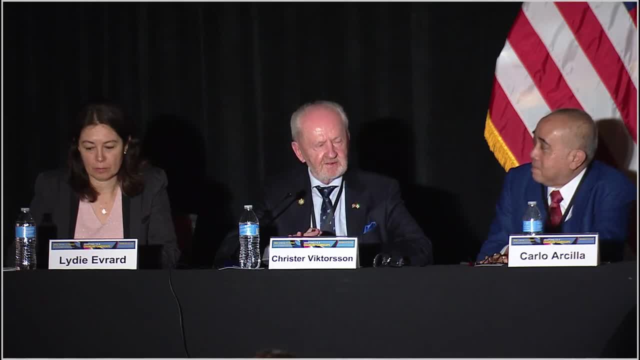 And I think that is one aspect. And then we study those and study the country of origin, who are the sort of vendors of these types of reactors and make sure that we understand their regulatory system On the acceptability of the country of origin reviews. it's an important topic. 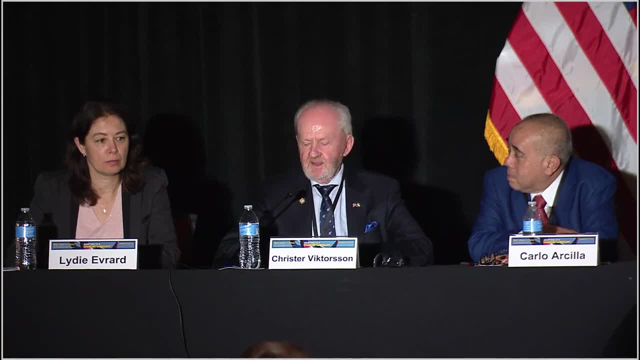 But it is not the first. We have two things to discuss and reflect on and we are trying to work in this initiative that was mentioned from the IEA nuclear safety and harmonization and standardization initiative In working group three. there is a particular effort to document how you can accept this type of legislation and how you can make it work. 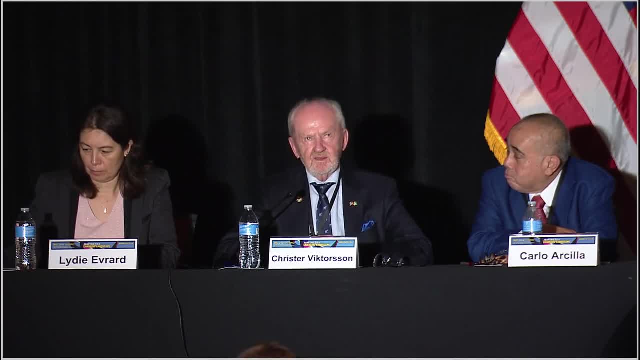 Thank you, Thank you very much, Thank you, Thank you very much. And at the end of the session, I would like to take a moment and say thank you very much, Thank you, Thank you very much. Thank you of reviews by other regulators. first of all, you need to understand their safety. 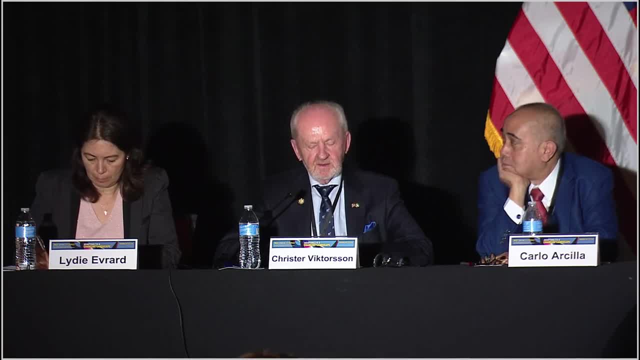 philosophy, you need to understand their regulatory system and you need to understand the operating experience. I think the reference plant concept is an very, very important concept to keep in mind if you want to be effective and efficient and use that and then. but they will always be differences between the 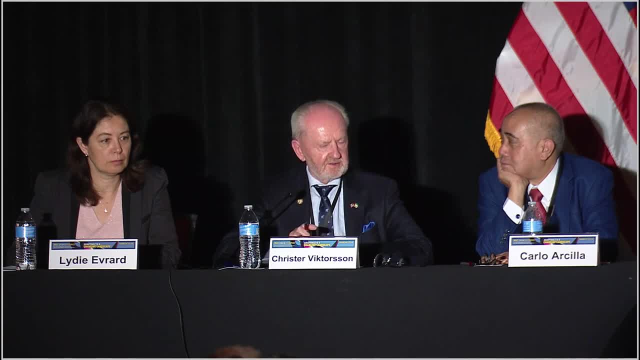 reference plan and the plan that you will get. because of local conditions, you have to adapt. we have many, many such differences. so we asked from the, from any applicant, to develop what we call a departure report, which is gap analysis between the difference between the Shin Korea plant in Korea and the Baraka design. 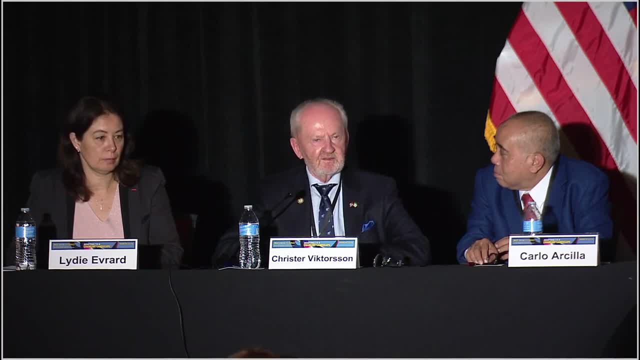 There were differences in cooling systems because of the temperature environmental conditions. There were differences in the frequency of the electricity. We have different national systems And all these things need to be very clear. So those are the focus of the regulatory attention. So once you understand this, I think it's easier to accept. 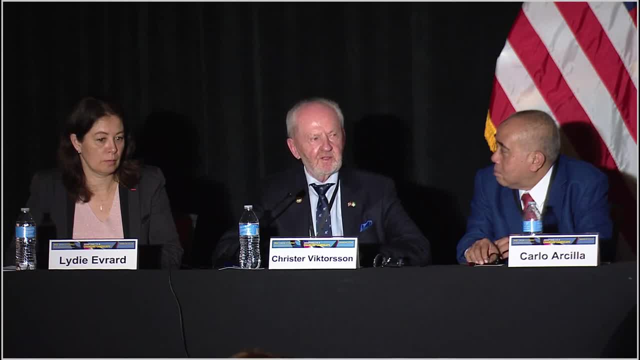 We had also second from Kinz sitting in our office for many years to help us to understand the Korean regulatory system. We will follow the same methodology for any new nuclear power program, whether it's SMRs or light water reactors of big size. Thank you. 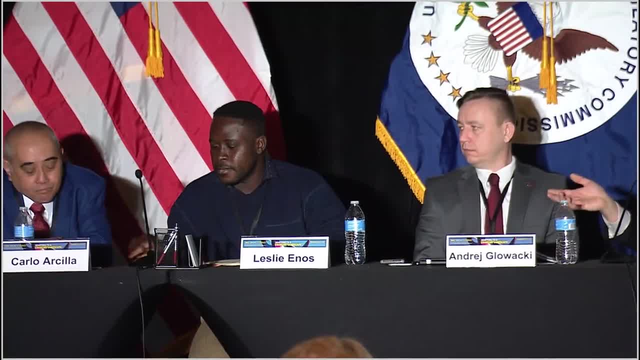 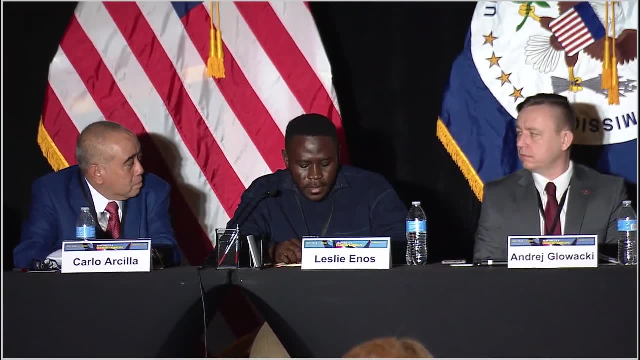 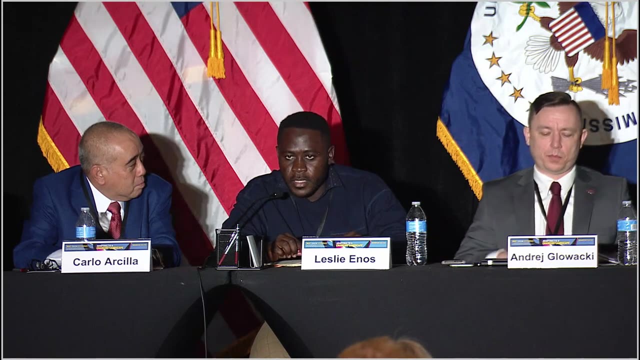 Thank you very much. Would you like to jump in, Mr Enos? Okay, So I would just like to say that, in perspective of Ghana, we, right from the beginning of developing regulations and guides, we are encouraged to not do anything in isolation. 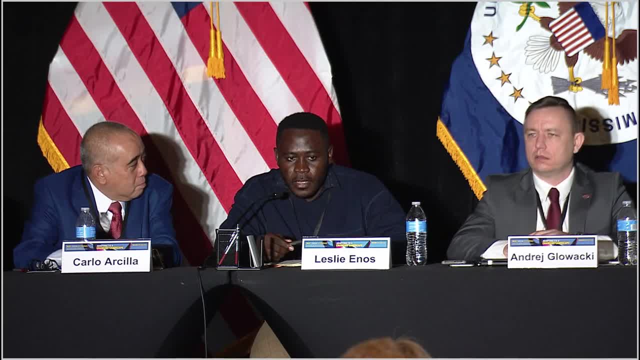 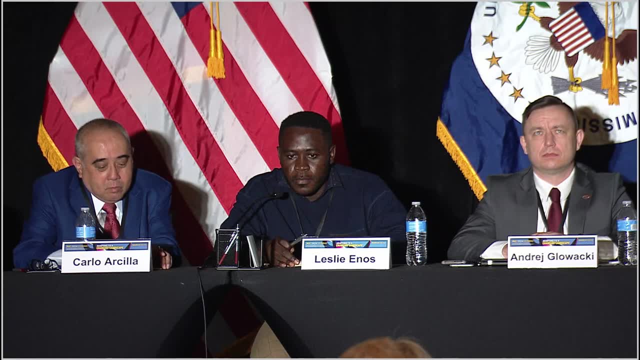 We try to look at perspectives from other countries and what the requirements are like. So everything is, Everything is. Everything is developed with information from other countries. We take all those things into consideration And all our regulations and documents are being reviewed through other organizations. 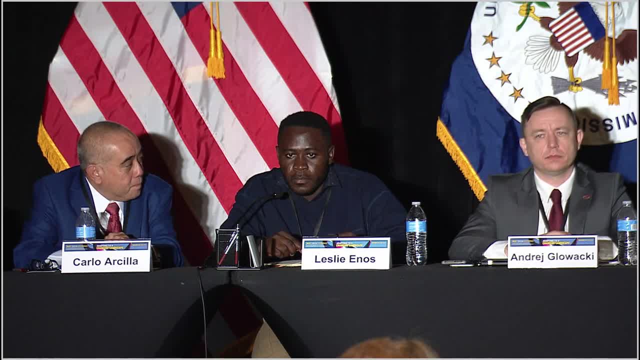 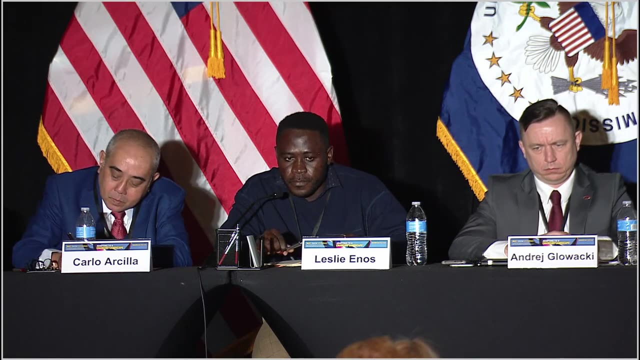 international organizations which where they try to incorporate new technologies- And we try to consider the new technologies which are coming up in our regulations as well. And, lastly, we some challenges. that we are facing is basically inexperience, but we have a very strong human competency: development plans plan. 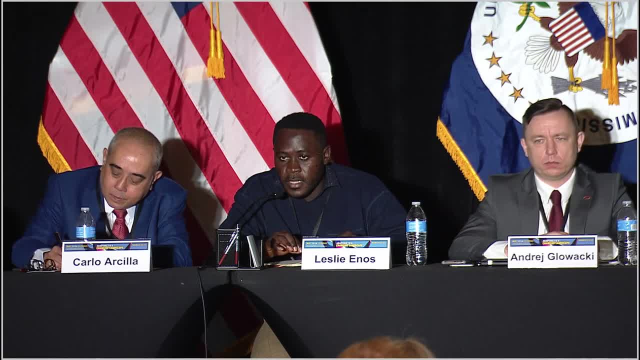 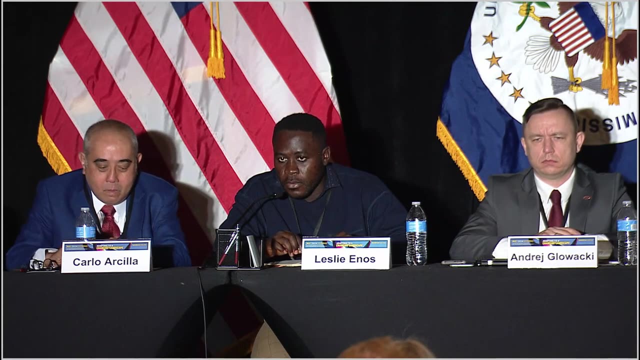 which is currently ongoing, and most of our staff have received them, from level one to level four of this training and more support from other international organizations. It's been provided to us And that will make us prepared for our review and assessment process. Thank you. 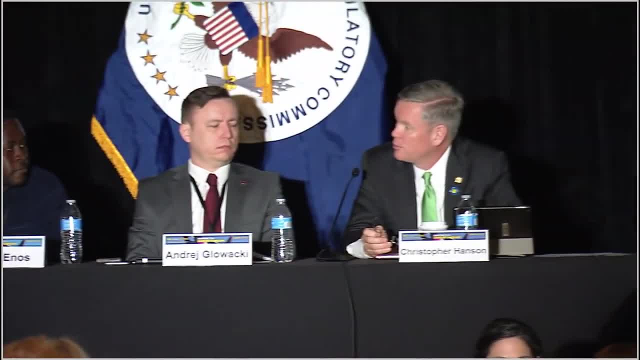 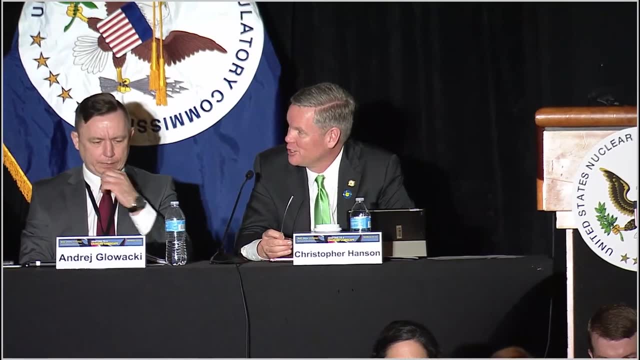 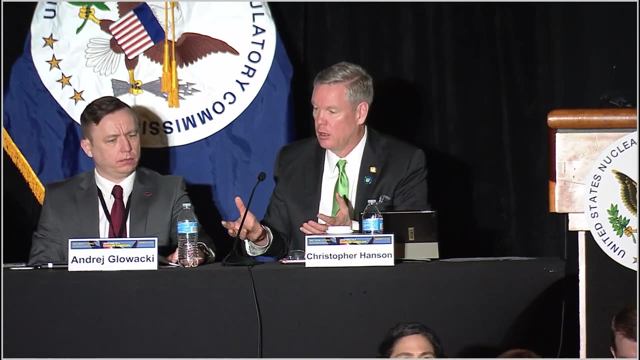 Thank you, Deputy Director General Everard. I wanted to ask kind of a follow-up question. Director General Victorson raised NSE and working group three and, as we were having this conversation, I was curious about how the particular instances of frameworks and controls are being implemented. 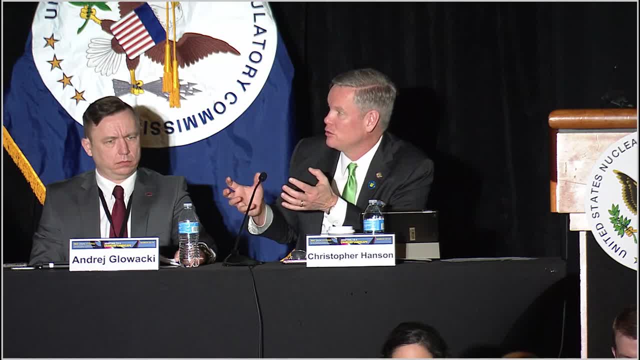 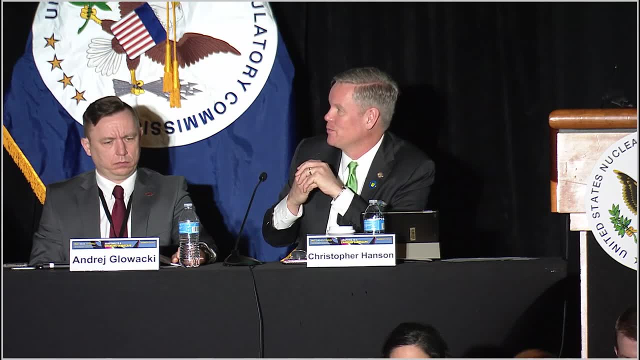 I mean, I know that NSE is one of the countries adopting other reviews as kind of being generalized and elevated at that higher level, and certainly Director General Victorson kind of touched on that. but I wondered if you'd like to expand on it a bit. 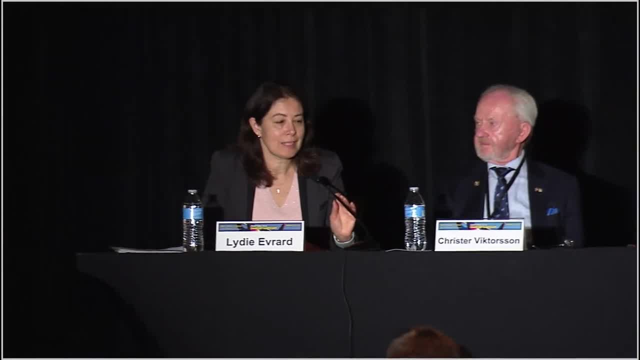 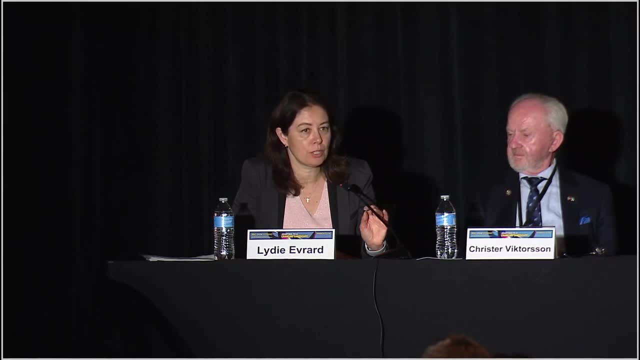 Thank you. Thank you very much for this question. So NSE, it's a new approach for the agency and, I think, for many member states, because we are considering different approaches at national level or at regional level, Because there are some initiatives. so the US, Canada, in Europe as well. 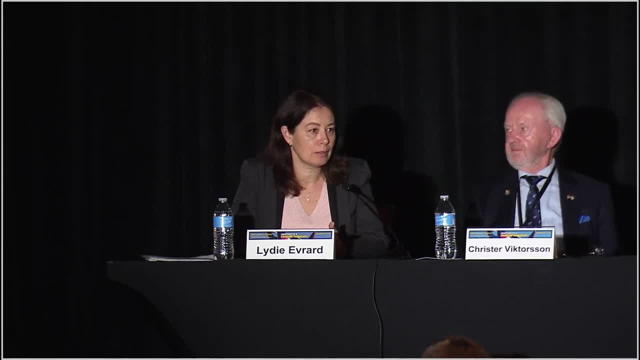 So we observe that there are already some ongoing work: how to learn from other experiences and how to leverage, you know, these lessons learned, for the benefit of greater efficiency, of course, but in addition, to avoid duplication, because we can observe that there are similar. 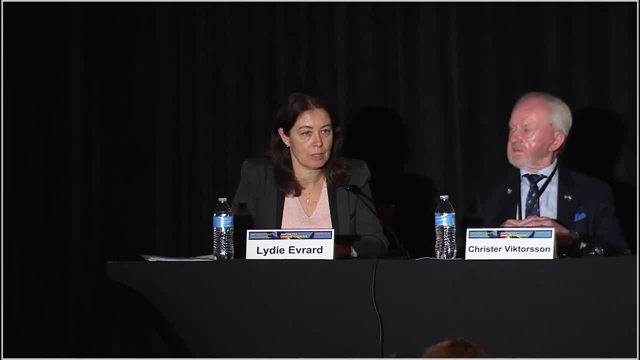 priorities, of course, throughout these different initiatives, and we may have some benefit from capitalizing this new experience in new designs. So this is really the concept of NSE. After two years now, we have learned a lot, including regarding the definition of the 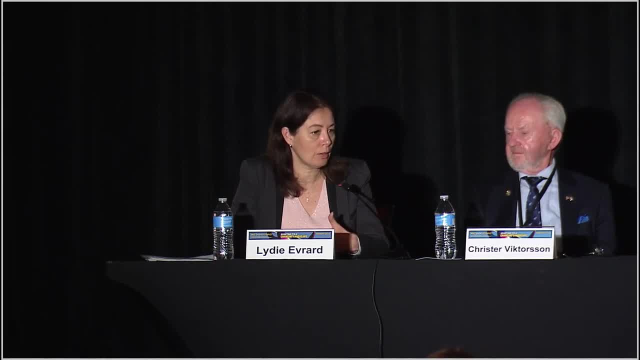 objective And really now I think it's clearer that the objective is to facilitate the development of SMRs, to facilitate the safe and secure deployment of SMRs. So it's not only how to deploy SMRs but how to make it as safe and secure as possible. 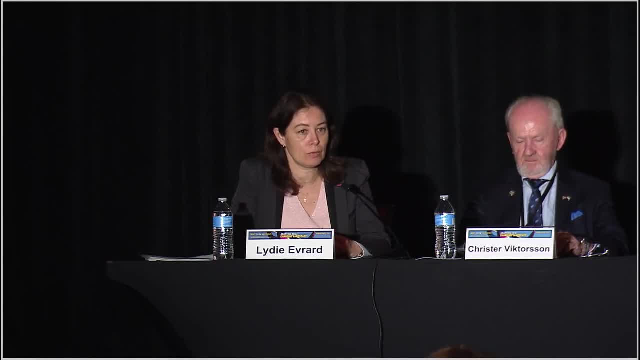 And there is a wealth of knowledge throughout the world, and NSE is really aimed at capitalizing, you know, this great experience and then putting this experience at the level of, at the global level, so that many member states can benefit from this experience, even if member states need it. We have countries with very developed nuclear programs, but we have member states that would like to use SMRs for domestic needs and they are starting from scratch. So we are trying to have this international cooperation as a force multiplier, as we mentioned. 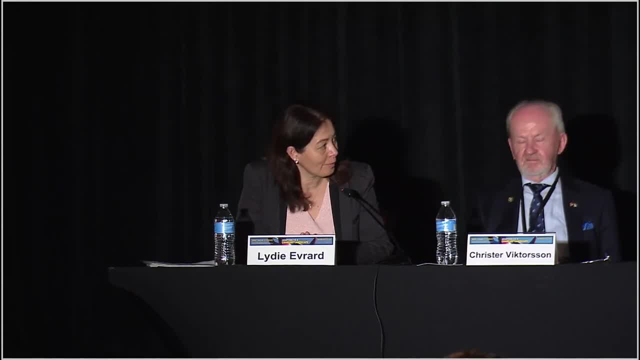 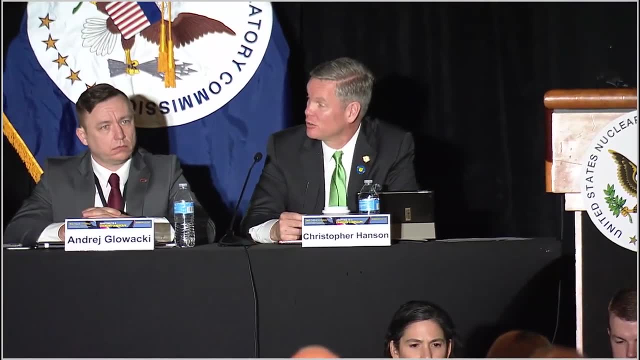 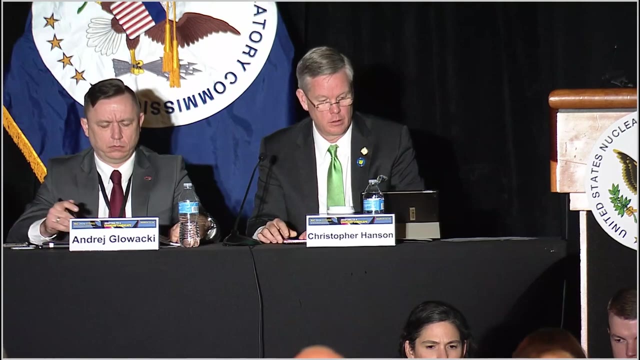 on Tuesday and this is really, you know this- objective. Thank you, MR. I've got a number of questions from the audience, so I'm going to start to go to those, And the first one that I have here is for Director-General Victorsen, and you know, 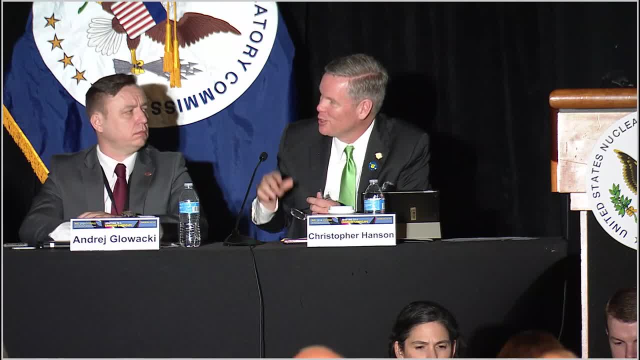 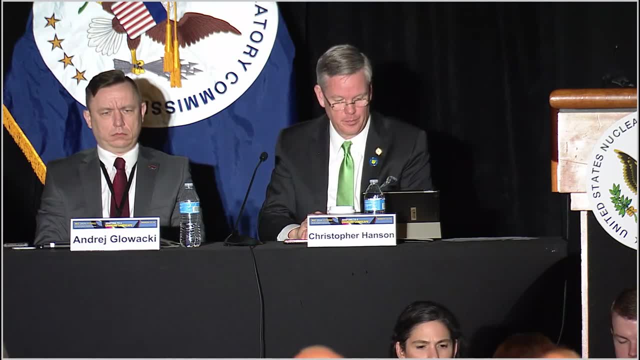 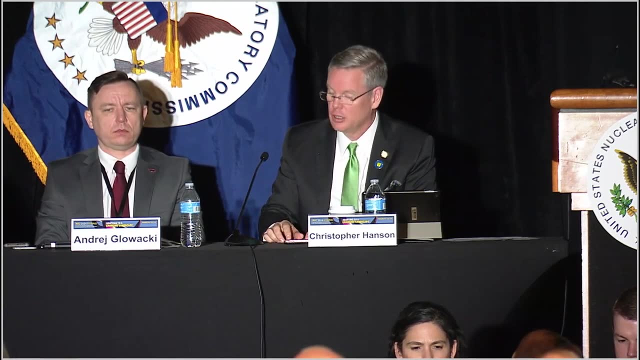 I think there's a question here that I think was drilling into maybe some of the lessons that you've learned, as standing up an entire regulatory body while you know, while safely licensing and overseeing The construction and so forth, and particularly are there lessons that maybe haven't gotten. 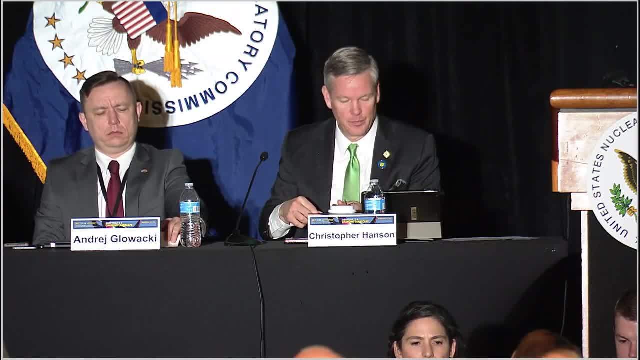 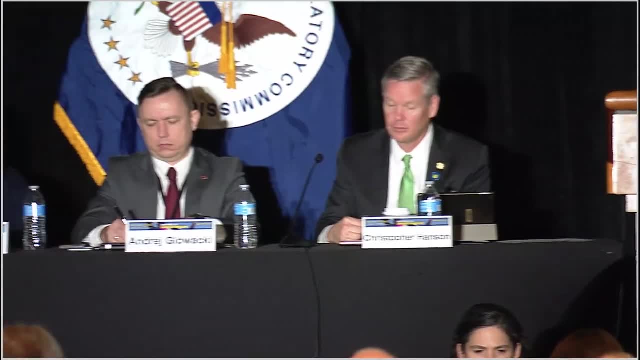 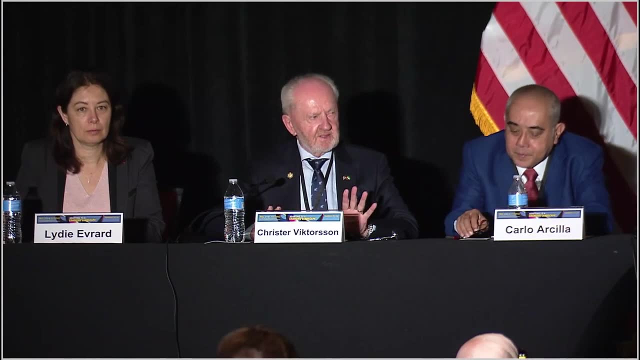 as much attention, but that you thought were really contributed to your success, MR. Yes, certainly there are. We were in a particular situation. As we have heard from this panel, my colleagues in the panel, There are a number of things. 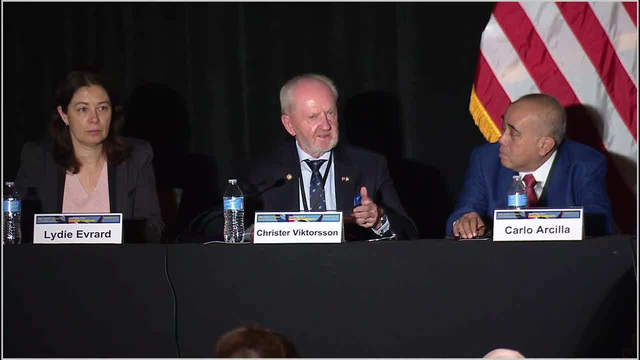 There are already programs or regulators existing In the UAE. we didn't have anything of that, So this is a difference. So we started really from scratch. So the approach was recruit experienced foreigners to establish the regulator, But this was not fast enough. 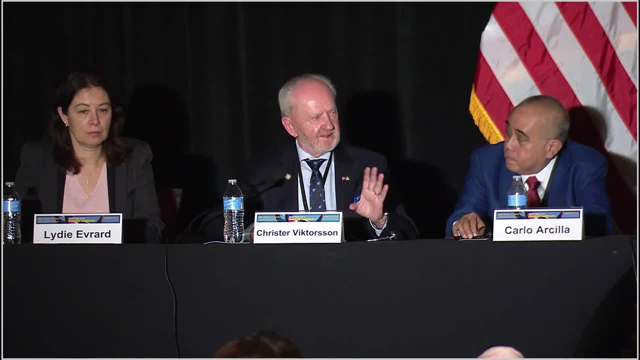 We couldn't do it fast enough. We couldn't do it fast enough to cover the capacity and capabilities. So we contracted technical support organizations, two US-based and one European-based, and divided the PSAR, the application chapters, and distributed to them. 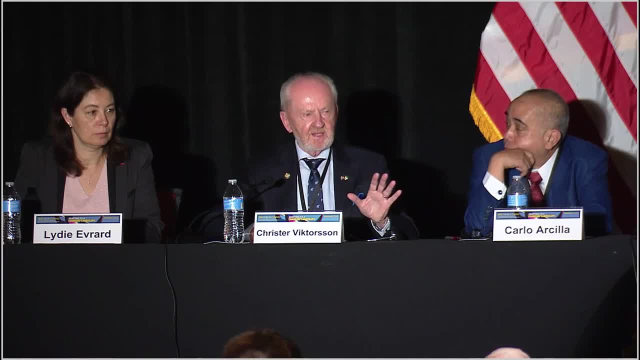 And we- our expats that we hired- they led, they were project managers and they led the TSOs And we made sure that we got the results that we needed according to our own regulations. So we needed to provide hundreds of detailed instructions to the TSOs. 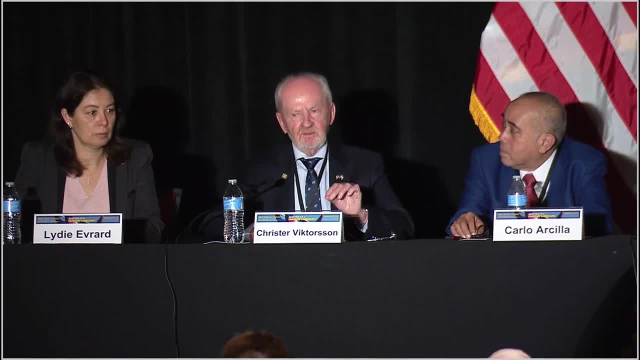 So it was a significant work to do in order to lead them And the people we recruited. they were knowledgeable to make the decisions, So we made our own decisions. We were a small organization, But we relied on external resources, MR. We had a lot of internal organizations. 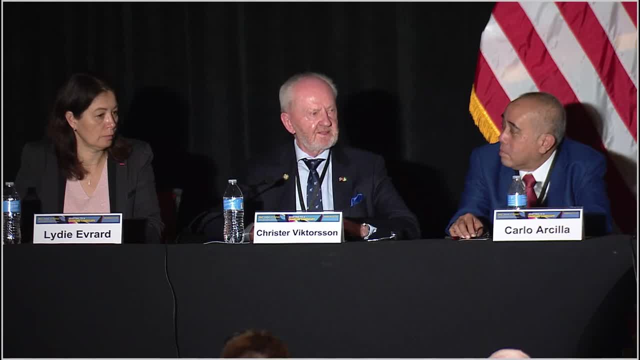 We used a lot of IEA support. I should mention that the first in-EAR mission we had in 2011, where they checked that we have programs ongoing to cover all the infrastructure elements. So we needed security. We needed offsite emergency. 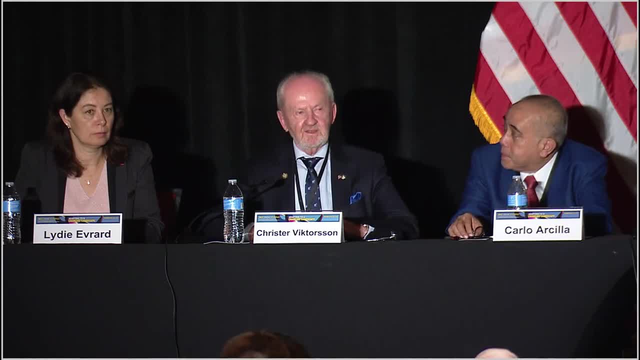 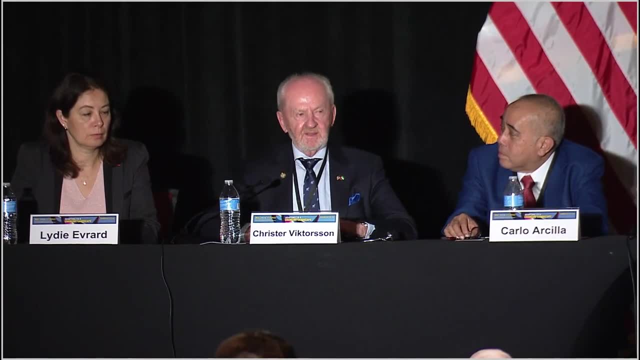 We needed safeguards, And many other organizations are involved in this: security organizations, customs for export-import control. It's a big project, MR. It's a big project. It's a really big project, MR. It's a big project. 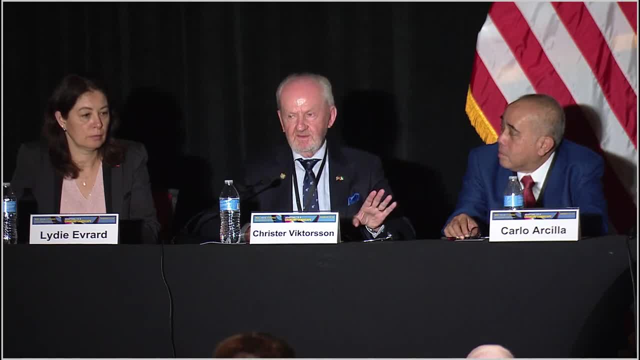 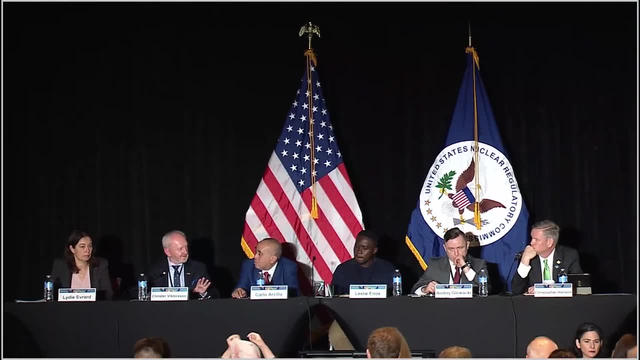 But it's not just several different organizations, It's a big project that has a huge impact on the environment, et cetera. And so, and then the first IRS in 2012.. Quite early stage, But this was in relation to our issuance of the construction license. 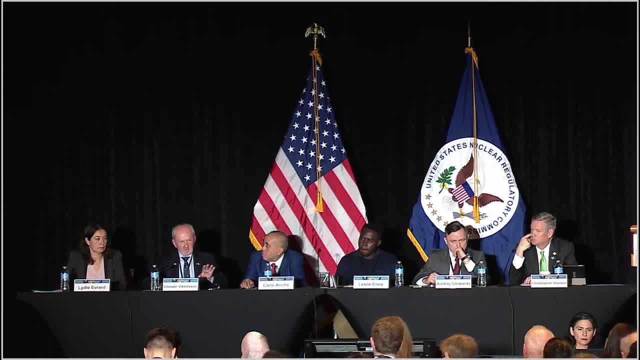 We issued the first construction license in July 2012.. It was a little bit delayed because of the Fukushima accident So we had to factor in- So we sort of stopped and paused MR, a joint NSREG approach in Europe, and made sure we understood how they did this in the 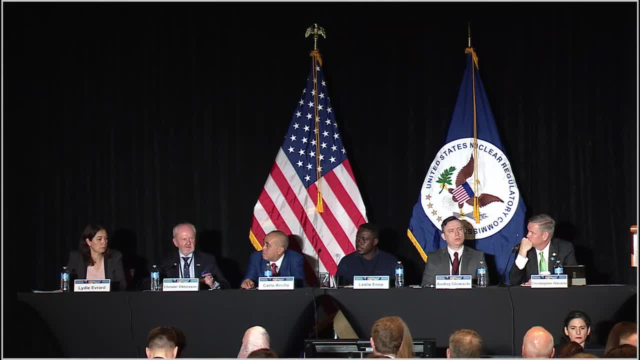 European countries, And we used the same methodology: identify the cliff edge effects in various steps, And then we were done by that by July 2012.. And then we could issue the construction license for Unit 1.. We have also another concept which I didn't mention before, something called 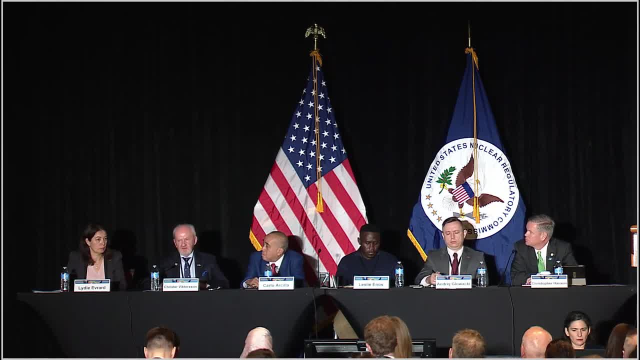 International Advisory Board. So the government of Abu Dhabi set up something called an International Advisory Board with high level experienced policy makers and nuclear professionals from a number of countries. It was led by previous IAEA Director General, Hans Blix, who was a representative from France, from US, from Korea, from Japan, from all over the world, with 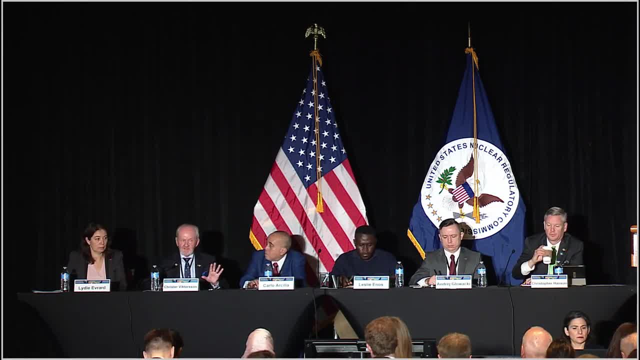 experience And they were very challenging. They came twice a year and asked to report, not only Fanner, they asked Enec, they asked Khalifa University on the capacity building side, asked the other authorities to come and report. what is the progress you have made? 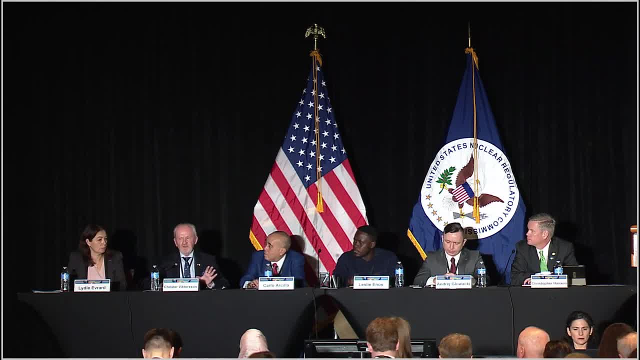 Thank you And gave us advice. If you are interesting to follow this work, they published very transparent reports on the internet So you can. International Advisory Board of the UAE. you can find all their reports And it gives you the history of our development. This was a very useful concept. 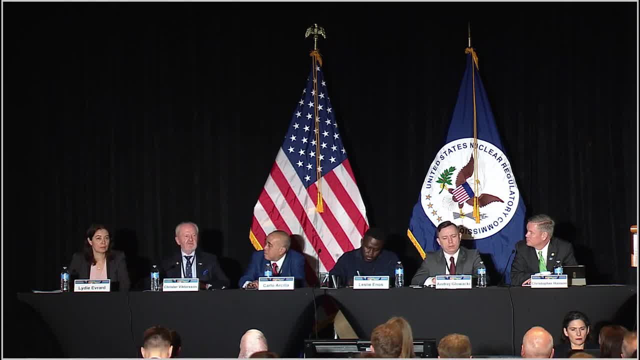 which gave us support. It gave the international community confidence that we were developing the program peacefully and in line with highest standards of safety, security and safeguards. Thank you, That's fascinating and I think there are a number of good points. I'd like to pick up on just one and I want to ask some of our other colleagues about the use of TSOs and how, in each of your unique contexts, how you're approaching the issue of the use of a TSO and kind of what the status of that status is and how you're going to do it. 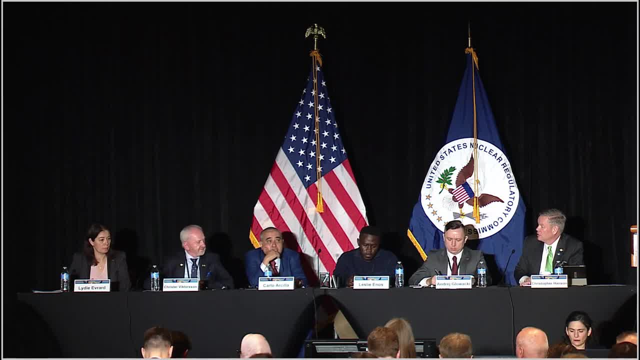 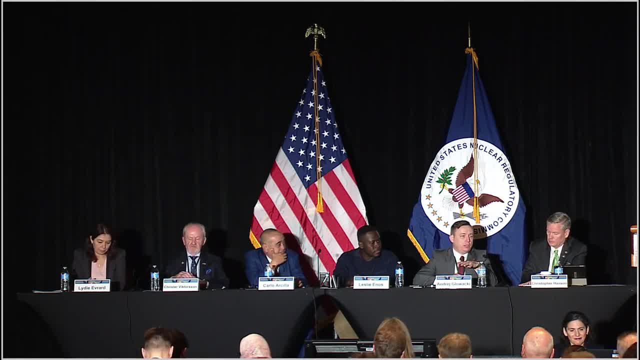 in licensing nuclear power plant. yet then we did not create any unified TSO for regulatory authority in Poland. We rather wanted to use different organizations, different institutions on different disciplines. that they will help us reviewing the documentation, And there is a mechanism in Poland. 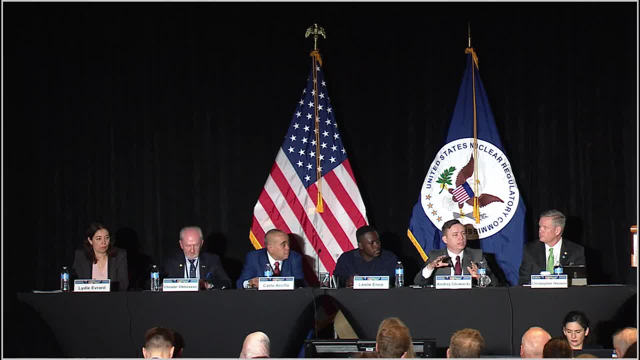 which is called the authorization for the TSO. This is a kind of a mechanism to pre-verify the institution which has to have enough competence, but also to avoid a conflict of interest, And this is a mechanism we use up to now. 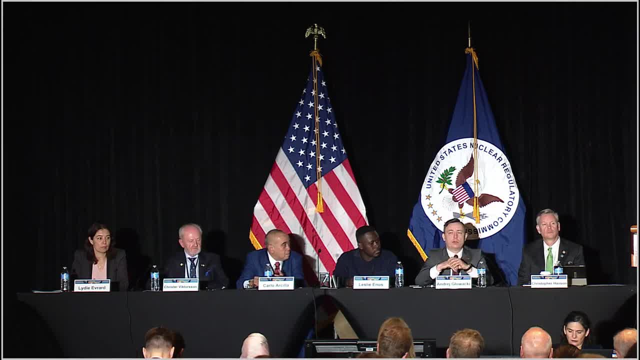 And so we've, as a regulatory authority, we've kind of selected these topics which we will ask for, the technical external support and the competencies we do not be able to build in-house. These are some sitings site specifics. 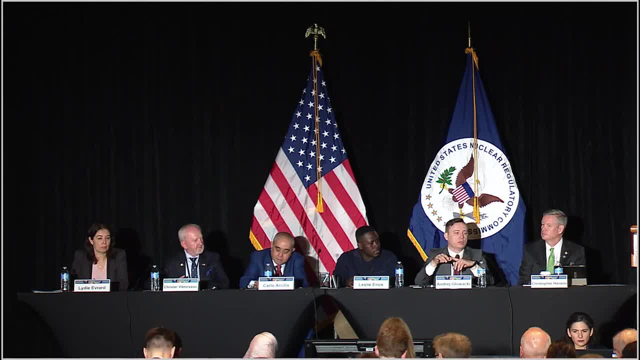 There are some competencies in the site examination, but also the review of safety assessment, safety analysis. The biggest challenge which I see- and we are working on that currently- is that according to our Polish law, we got 24 months to review the documentation. 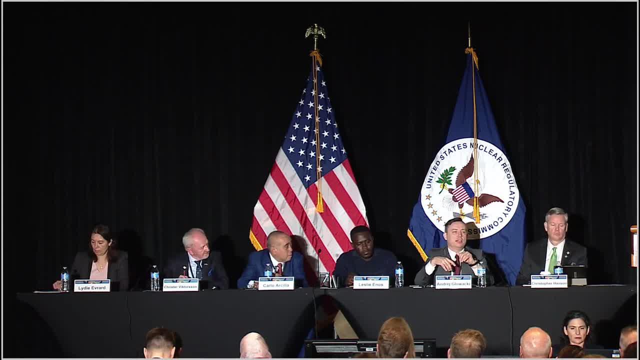 when the application will come And you can imagine that this kind of system of technical support organizations you have to. we have to go through the public procurement process which probably in some of the countries, at least in our country, it might take time. 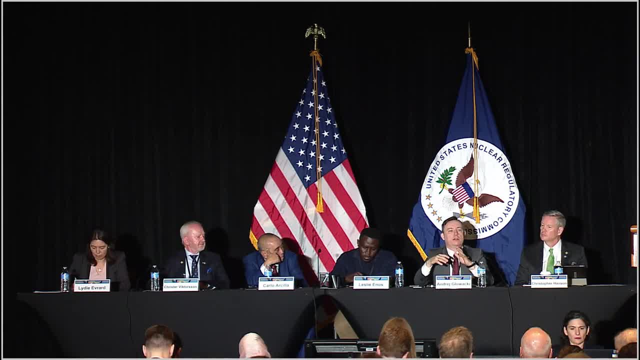 So we wanted to kind of also take this time, before the application will come, to prepare an agreement with those institutes, those institutions which gonna help us with the technical analysis being ready before the application will come. and mechanism: we have some ideas which kind of mechanism we can use, but it's a, it's a like a big challenge and advice. if 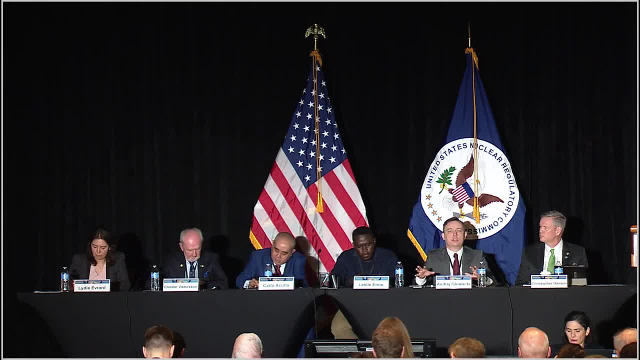 if you guys trying to use this kind of system, make sure that when, when the application will come, you will have a direct path to the Institute you choose, that they can help you. thanks, would anyone else like to tackle that? okay, fair enough. one of the questions that I've got here on the 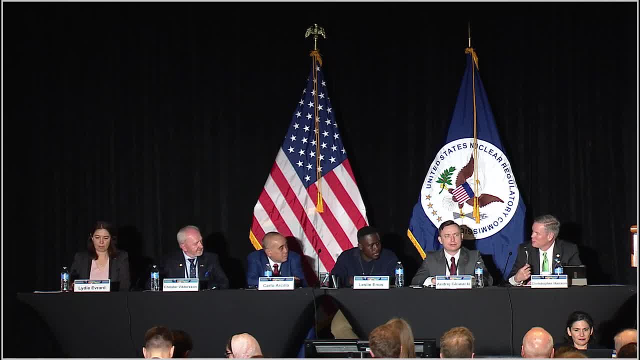 iPad actually has to do with. how are the countries in this group actually helping other countries? so, for instance, you know our friends in Poland and Ghana and the Philippines. you all have taken significant steps to prepare to regulate nuclear energy. how are your phones ringing from other countries who might be learn? 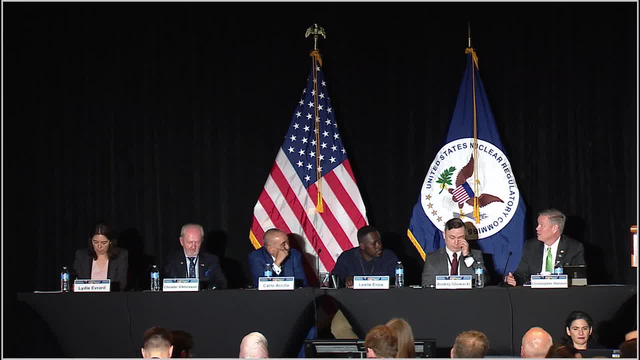 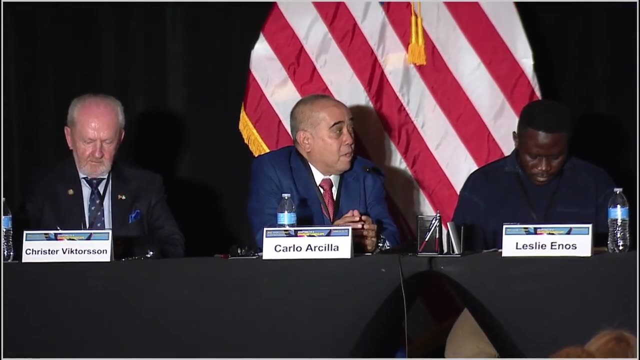 might be ready to learn from where you are on that, on that journey. yeah, please, dr, I see it. yeah, the Philippines is part of the ASEAN. ASEAN is the largest agglomeration of countries, about 600 million people- with no nuclear power, and it's one of the richest two per capita. that includes Indonesia, Thailand, Vietnam. 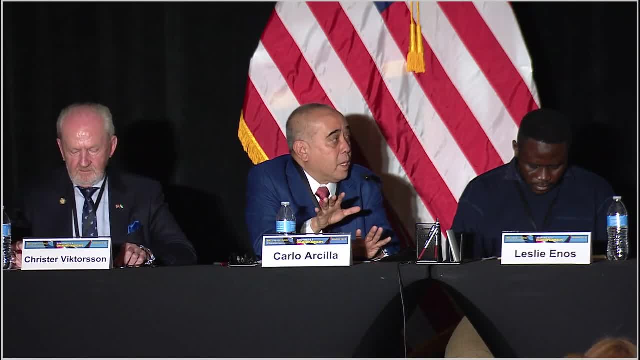 Philippines and and then differing, different levels of economic development. but we have a group called ASEAN Tom, which is the Association of regulators, and we meet yearly and believe me in scholarship, so we have many fake tenses. for example, we used three times around the world. so 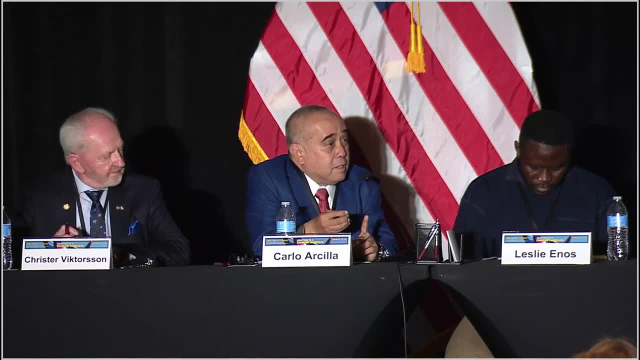 it's a really big group. we have 300ängen. what exactly is that medium? the? this is one of the thousands of people we are training in Brazil, so they have the same asylum equivalency, as big as the one from Indonesia. and you know, you just kind of get the picture. but the month that makes most 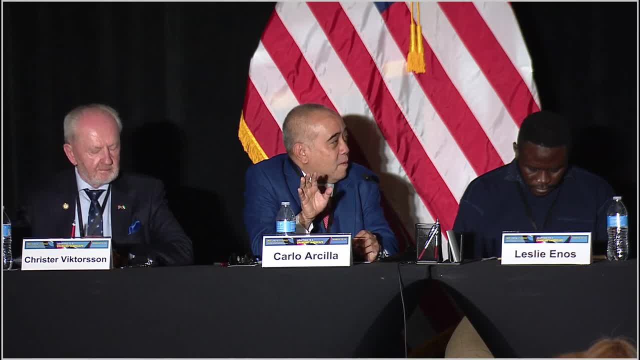 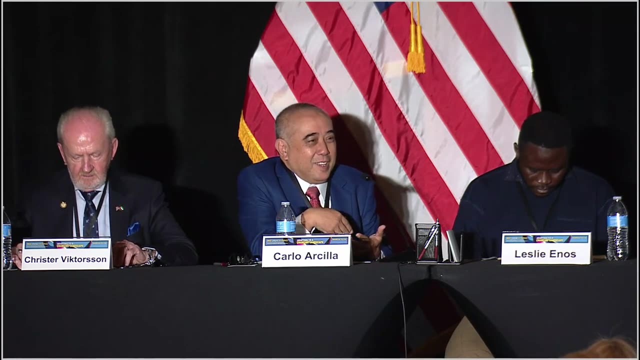 only job is to vet existing technologies. They say we have to choose the safest And they're willing to share, And they've shared especially vendor characteristics. And vendors are like car salesmen: They promise you everything And so it's good to among countries to see. 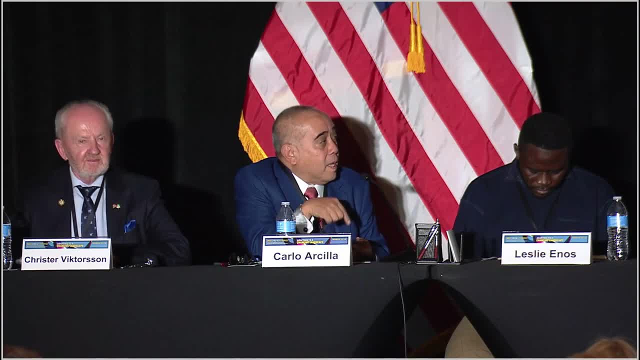 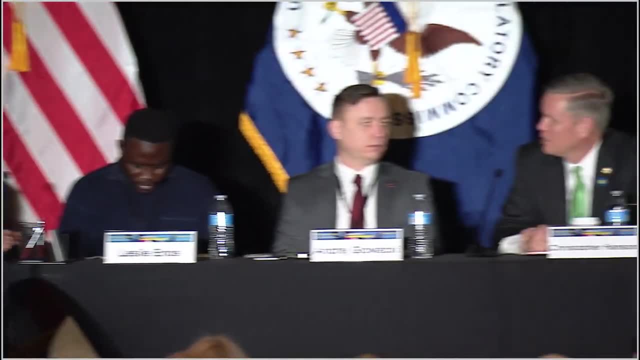 what are they offering you? And then so, for the realistic, And we will be doing that, We are doing that now in the ASEAN. Thank you, MR. Yeah, thank you, Mr Ennis. is the phone ringing in Ghana from neighboring? 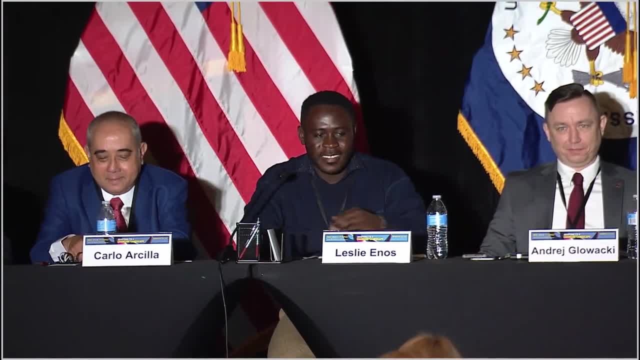 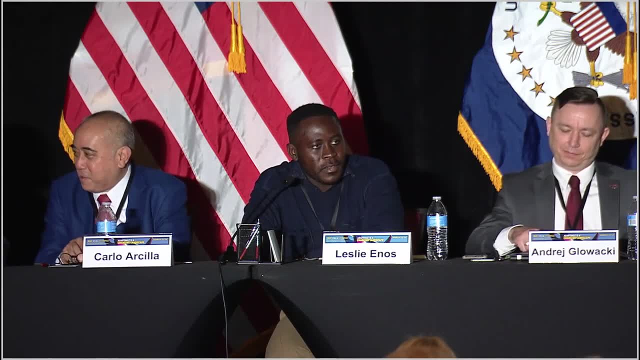 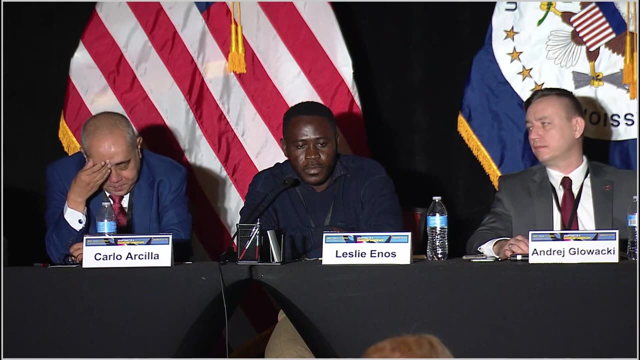 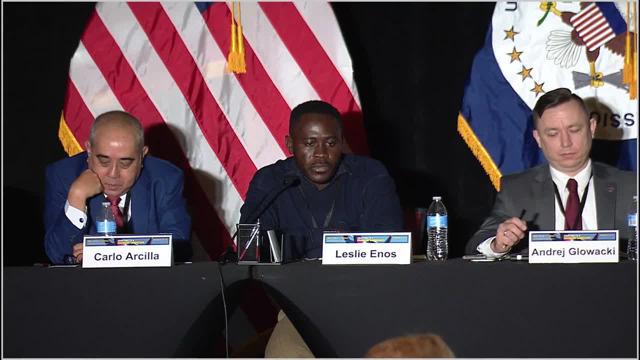 MR. Can I go to Nigeria? MR Yes, MR, Thank you, MR. Thank you, MR. This is Danhow Missou from Ur chang eiga lady from Nigeria, Ghana. MR. Yes, Morning, MR. Oh wait. 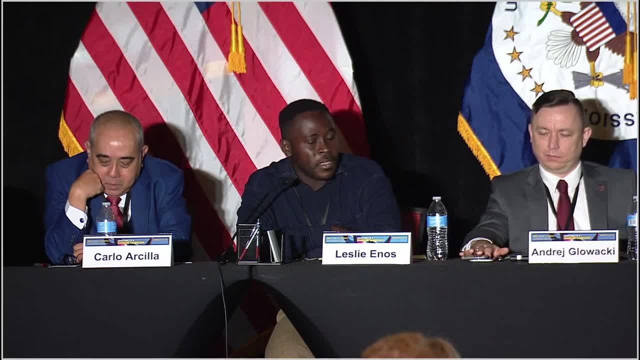 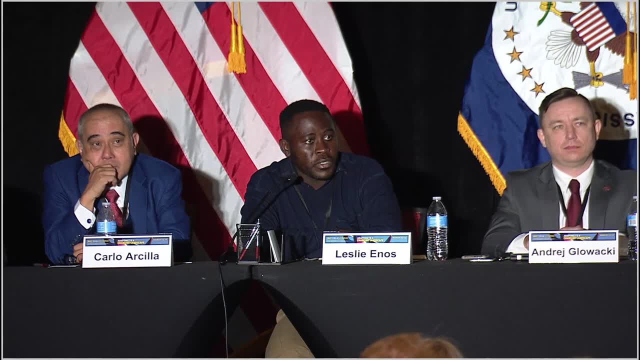 MR. Okay, MR, I understand what you said. MR, I said we are in the phase two, So we are-. Ghana is one of the foundation members for the markup for regulatory authority in Africa. So they are two currently senior management acquiring position in the forum where they extend their expertise to other. 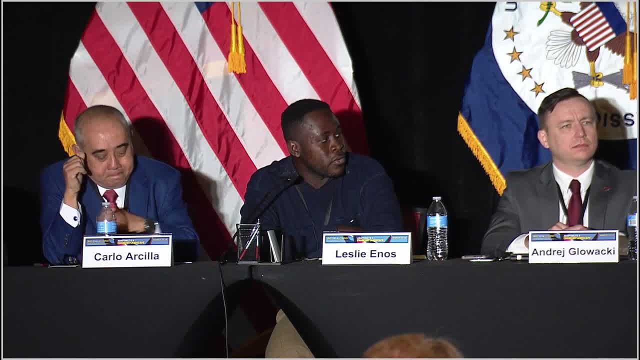 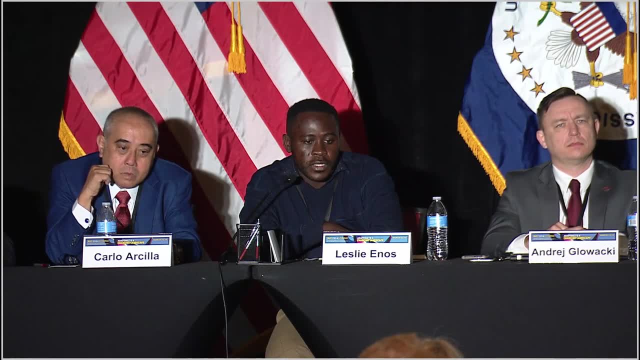 African countries like Kenya, Nigeria, Morocco, so that there is a-, MR And so- And in this way we're trying to leverage the opportunities in order to also give other helping hands to other African countries. MR Good, Thank you. 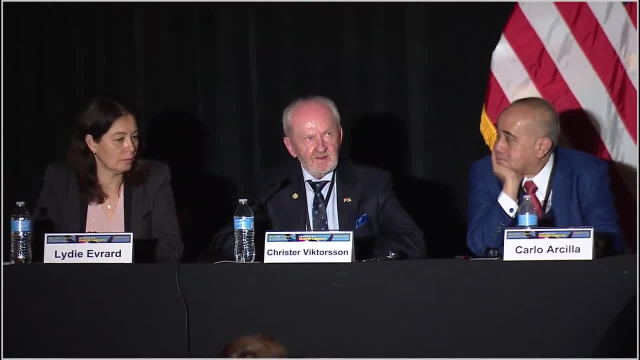 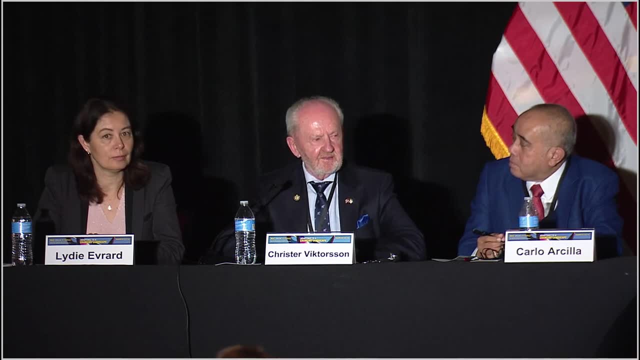 Yes, please, Yes, Thank you. So there is one topic that I think is very, very essential. That is, the regulation. So you are immediately faced with what type of regulations- design, siting, et cetera. So our approach was to rely on IAEA safety requirements, which are, I would characterize- 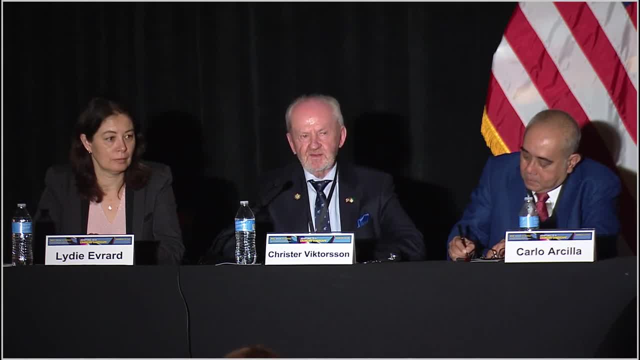 them as risk-informed, performance-based, And of course you have to. so we adopted essentially them, not word by word. We changed some aspects that were needed to be changed Because of local conditions. it can- security guidance is one example- and also design. 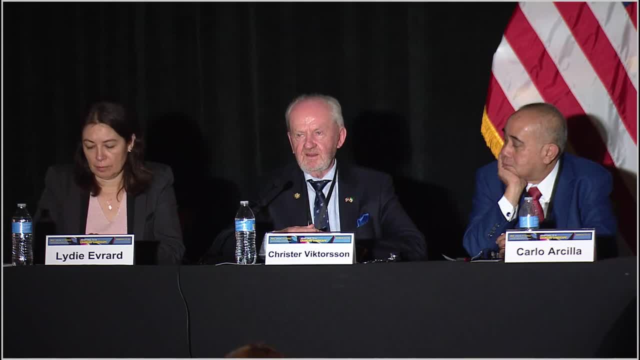 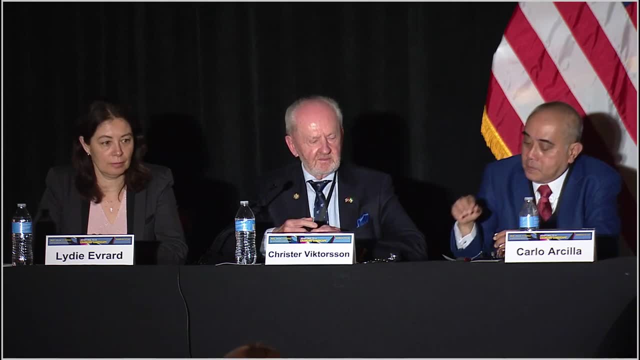 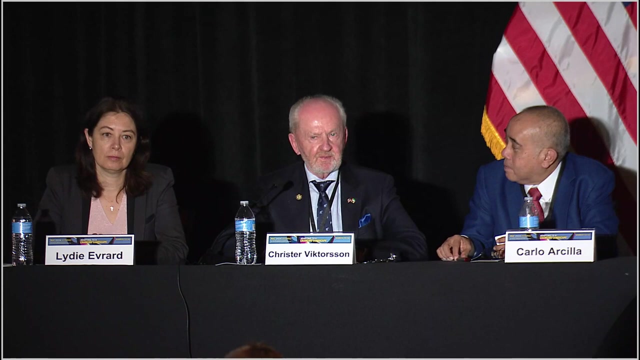 We are now revising the design regulations based on new revision of IAEA, but also because we might get new applications to site power plants in the UAE And we need to factor in the climate change aspect because we need to recognize that a nuclear facility it will. stay there for one century, 100 years, And many things can happen around us because of the climate change which we might need to think about when we site a new nuclear facility. So this is an important consideration that we will include now In the new revised regulations. 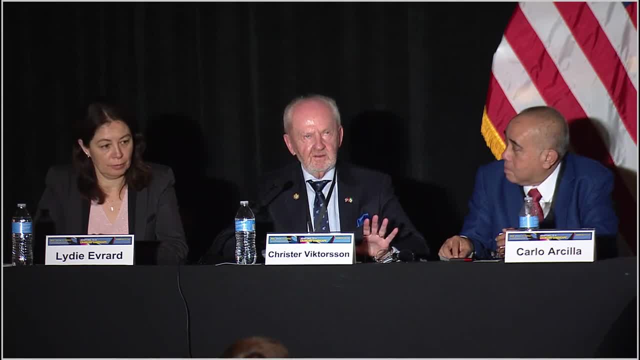 We have recently updated the regulations on leadership and management for safety And included requirements for the licensee to make sure that, on their highest level, they consider safety. We had recently an inspection for NAWA- And led by Mira, by the way- on the integrated management system of the operator, including. 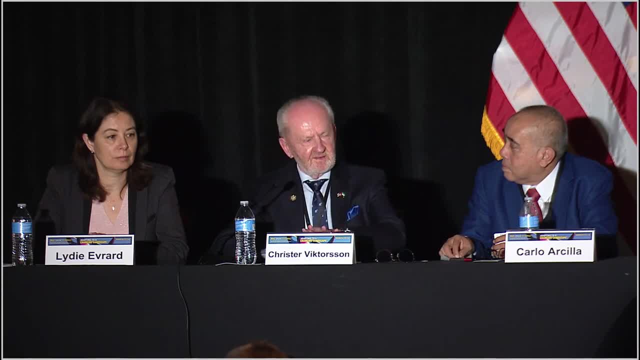 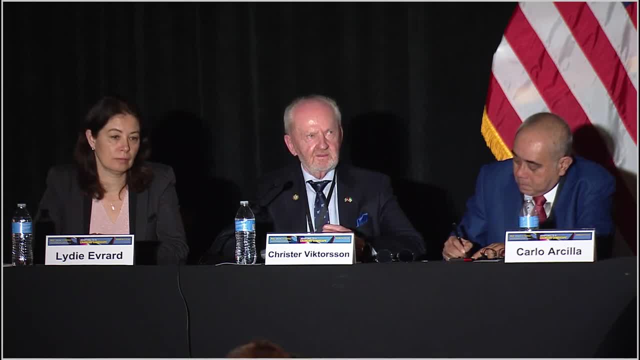 that, that, that, that that are, that they are against the spirit of safety culture. Do they have a questioning attitude? Do they have employee concern programs, for example in the utility? And another topic is the peer review services. 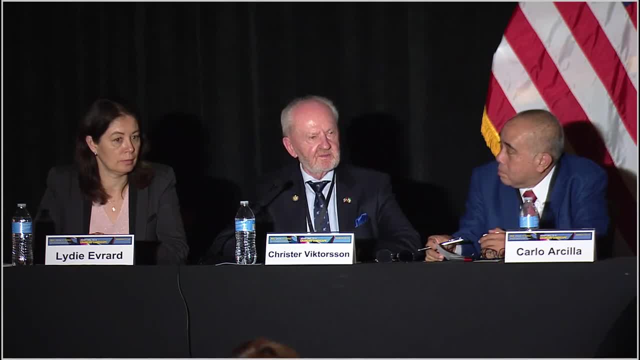 We have benefited a lot from IEA peer review services. We have done 12 or 13,, I don't know. almost all of them have given us very valuable advice, So I'm grateful. thank you for the IAEA to keep this going. 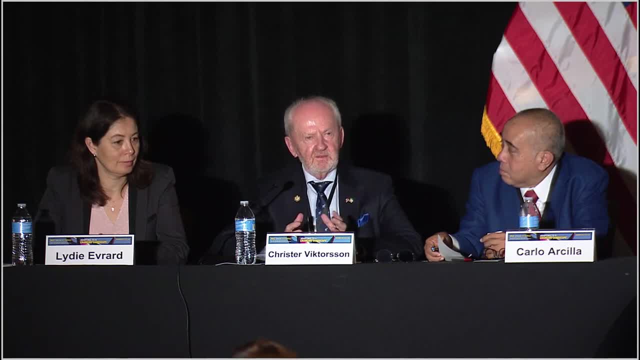 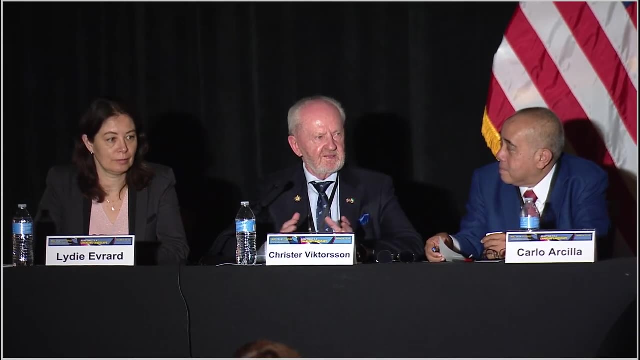 We are a member of RCF, by the way, and we have many requests to meet with other embarking countries in order to learn from the experience of UAE and FANR, and we are willing to do that. One of the principles of the UAE government is transparency, so 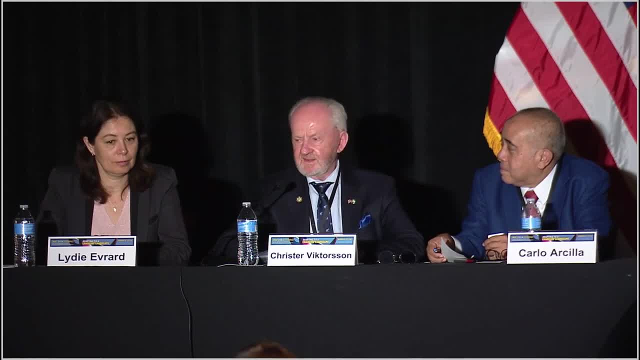 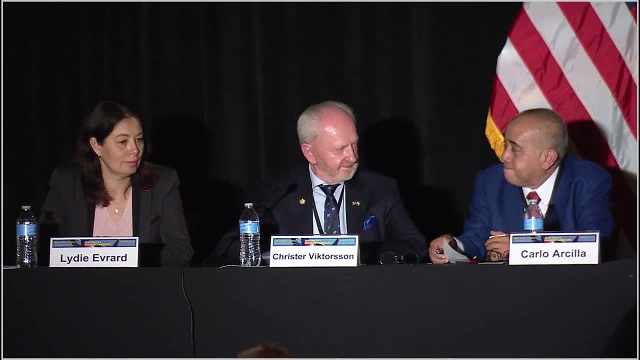 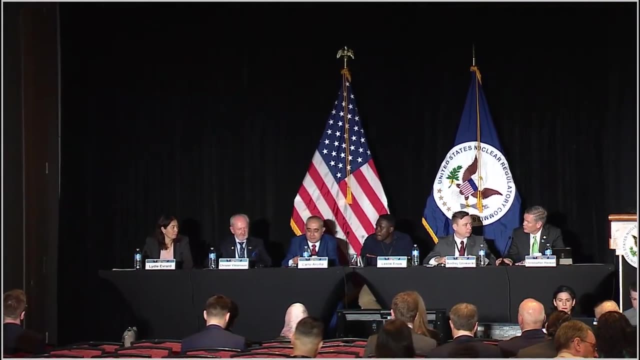 we are willing to share, But we try to go through as much as possible through IAEA, through the various documents and conferences, and share our knowledge, Thank you. Thank you, President Glavatsky, or Deputy Director General Everett. do you have anything you'd like to add? 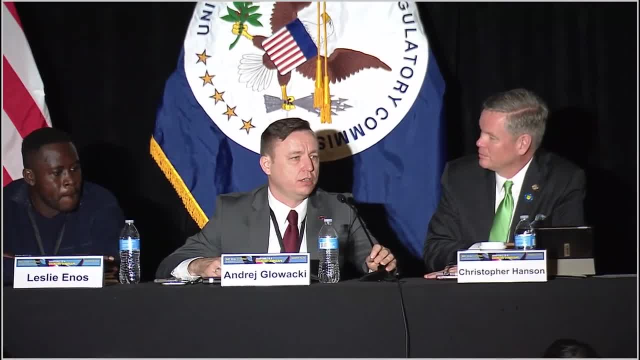 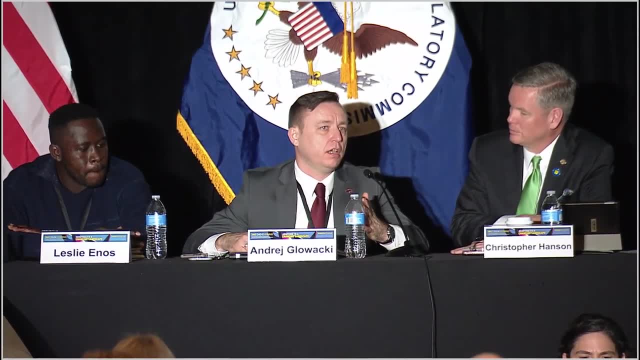 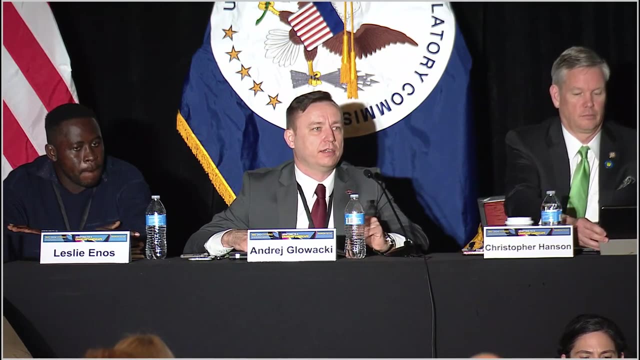 Well, I wanted to emphasize this RCF initiative, actually, which we are also a part of and we are ready to share our experience. Well, surprisingly, there are some- I see some faces from the European regulators who approached me sometime because 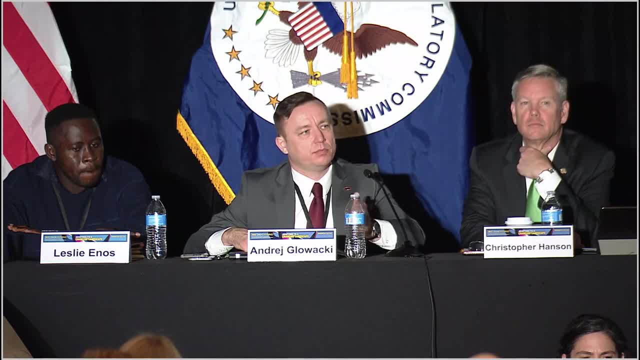 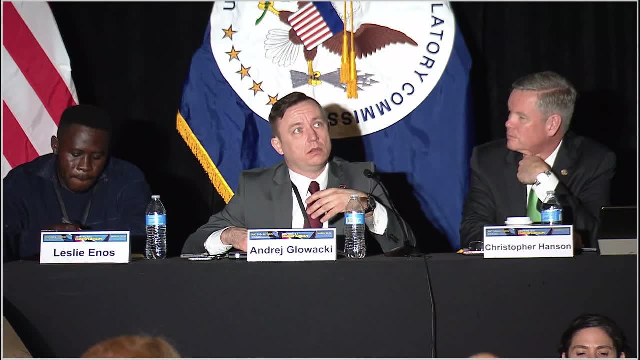 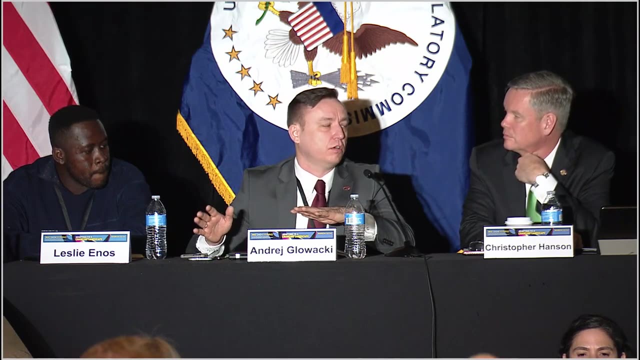 well, we got some knowledge, some experience in preparing for the licensing the new reactors, especially SMRs, And we are ready to share this kind of experience. One thing I wanted to also add is that please document the work that you have done. 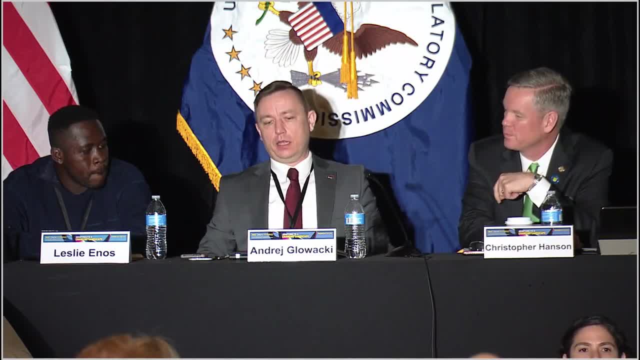 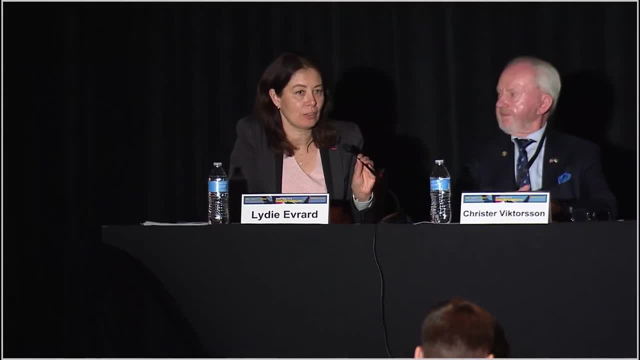 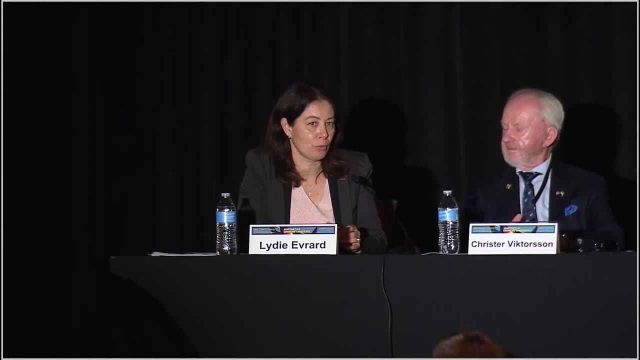 to share then the experience that you can gain. Thank you, Yeah, just a few words to maybe follow up on what just was mentioned on the services provided by the agency. So the range of activities is very wide, but we are continuing, you know, expanding the possibilities with ad hoc services.